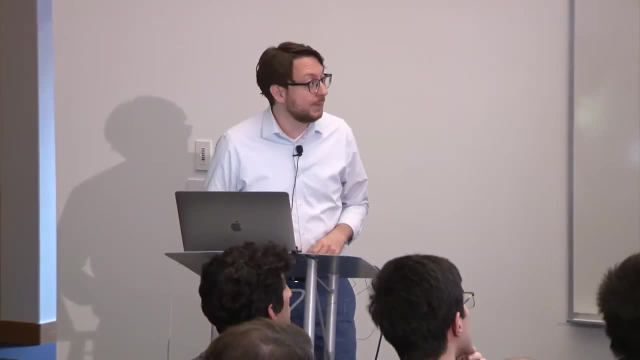 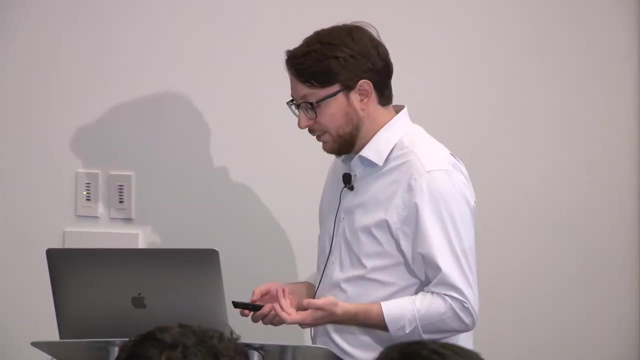 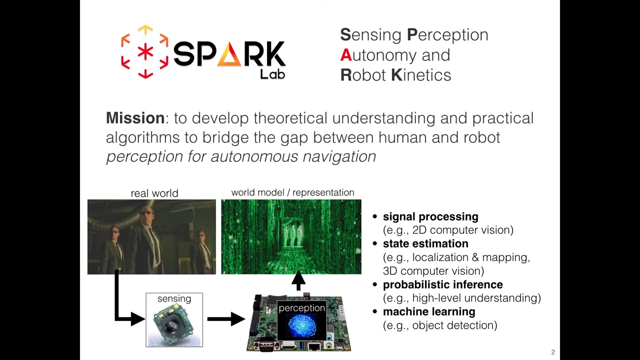 We're here to talk about Certified Robust Special Perception for Robotics. As Alberto said, I started at MIT as a faculty one year and a half ago And what I did at MIT is to create the SPARC lab. SPARC stands for Sensing Perception, Autonomy and Robot Kinetics Lab. 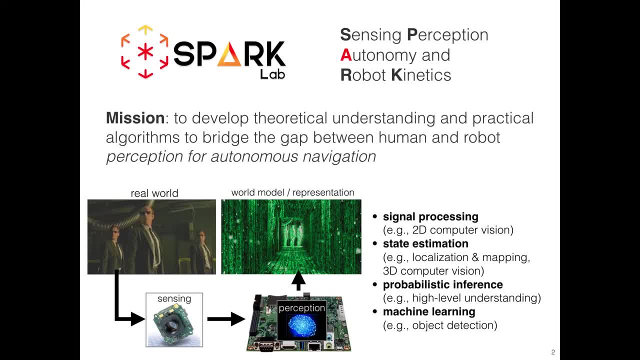 And the mission of my lab is at least pretty simple on paper- is to develop theoretical understanding and practical algorithms to bridge the gap between human and robot perception for autonomic resistance. And in this lab I'm going to talk about a number of topics. 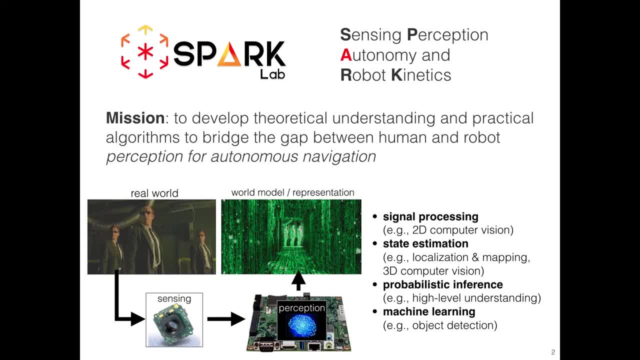 navigation. I'm sure that this audience knows what is perception, but you know. for those of you who don't know, you can think about this cartoon, in which imagine that there is a robot sensing the external world, the real world, with some onboard sensors. and perception is a set of algorithms and hardware. 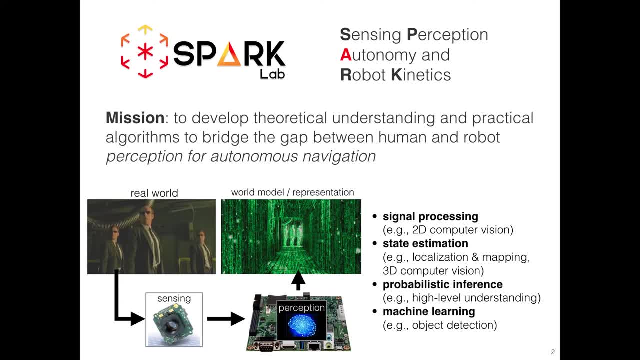 processing the sensor data and some prior knowledge to get an internal model of the external world. You can imagine that perception is essentially a broad umbrella for a number of challenges in signal processing, like computer vision instead, estimation, like localization and mapping in 3d computer vision, probabilistic inference, machine learning and so on. So my lab really. 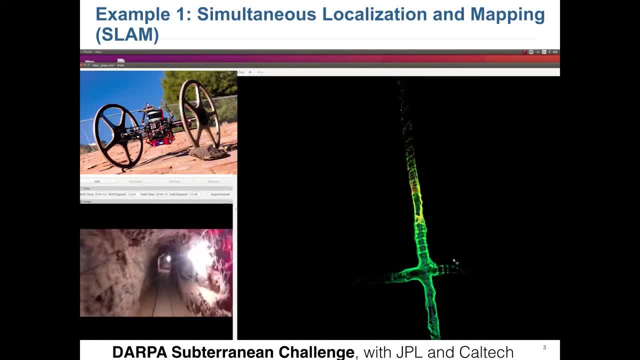 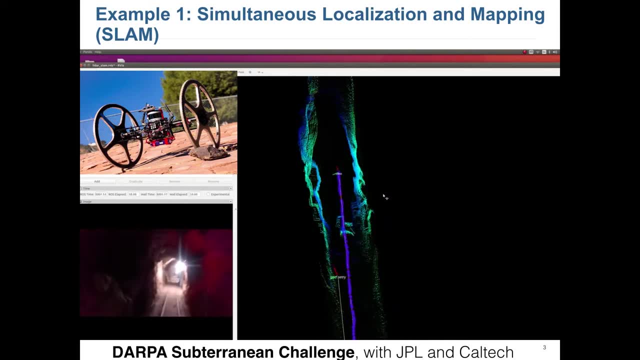 cares about perception and I want to give you two practical instantiation of perception problem that we care about. The first one you guys will be familiar with is simultaneous localization and mapping, SLAM. in this case you deploy a robot in a completely unknown environment, in a GPS denied environment. 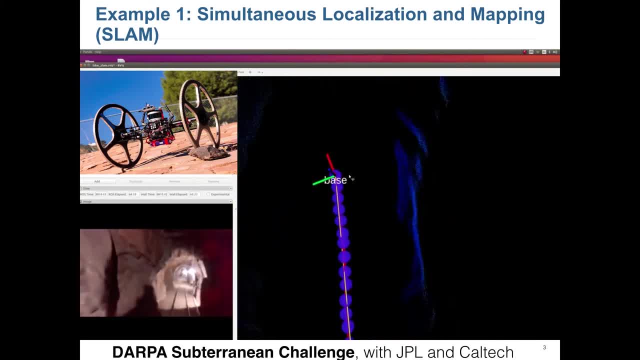 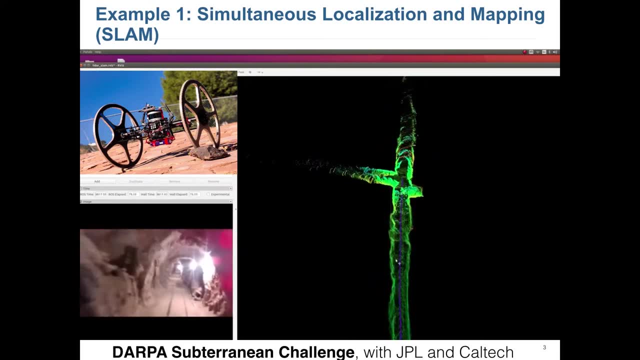 and the robot is in charge of reconstructing a map of the environment, while figuring out its trajectory, while moving in this unknown environment. This, by the way, is an example from a project I'm very excited about. you are part of the DARPA subterranean challenge, in collaboration with JPL and Caltech, and 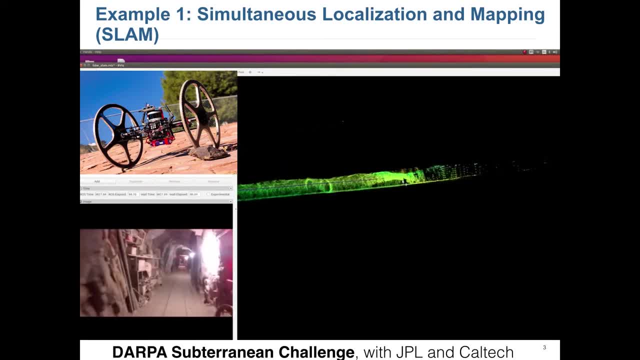 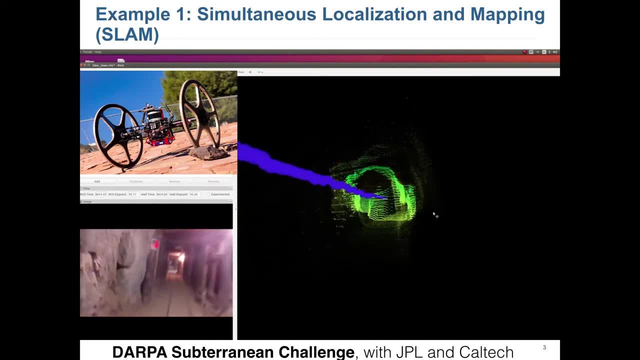 this is some experiment in which are mapping this underground cave. So of course, for this case I'm doing mapping with the LiDAR sensor in this kind of robot, but of course you can imagine that SLAM is a quite general technology that will apply also to different types of sensor and different types of robots. 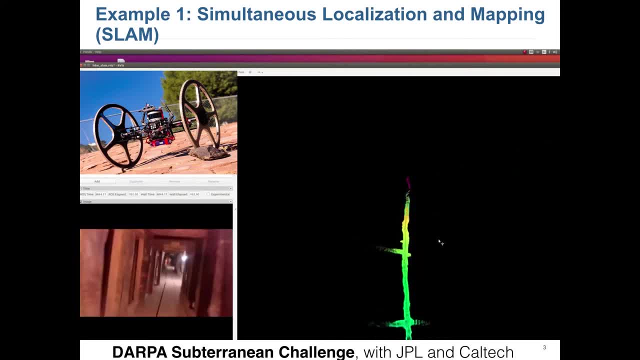 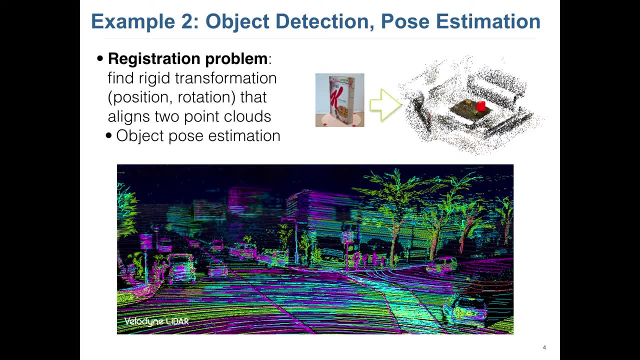 Alright. so example one is SLAM. another problem that I'm going to touch upon today is object pose estimation and object detection, and in particular, I'm going to talk about the registration problem, which is about finding the rigid transformation, which is a position and rotation that aligns two point clouds. 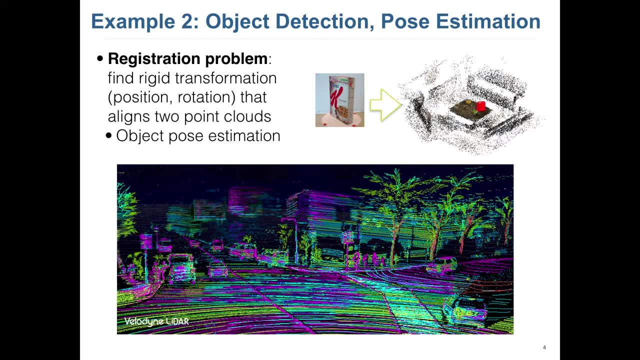 The typical problem that shows up when I give you a template, an object that I wanted to recognize, and I ask you to find that object in a big point cloud. Of course, typically you don't care too much about serial box and more practical instantiation is the case in which I. 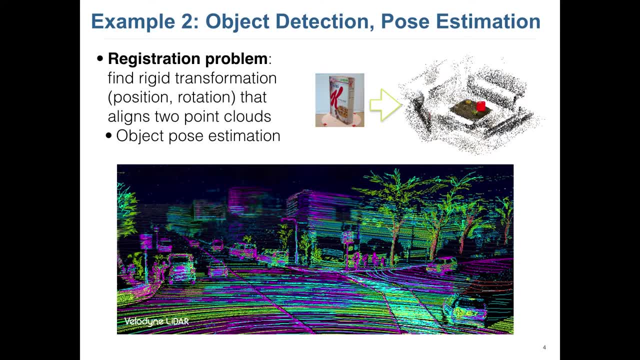 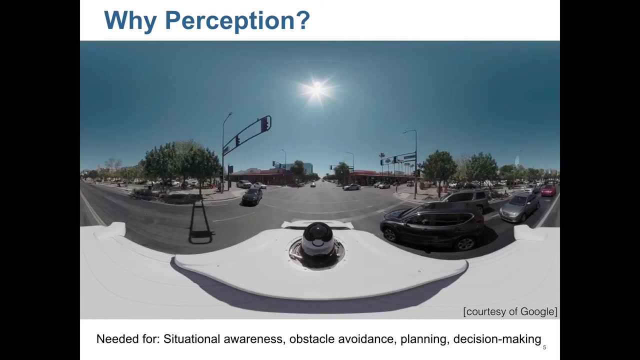 give you a valid and lighter scan here to look for a car, for example, for a known object. So a couple of examples here of perception and I want to stress for a few minutes why perception is really important for robotics. Let me start with an application we're all familiar with, which is self-driving cars. You can 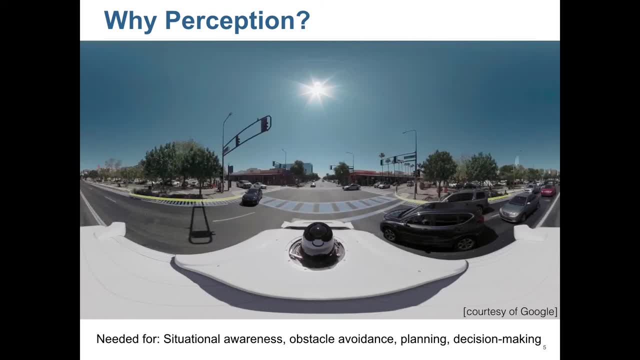 imagine that for a self-driving cars to operate safely in the environment, the car has to figure out the lane boundaries, pedestrian crossings, the position and the presence of other cars, potentially track the speed of other cars, detect traffic lights and potentially reason in terms of the 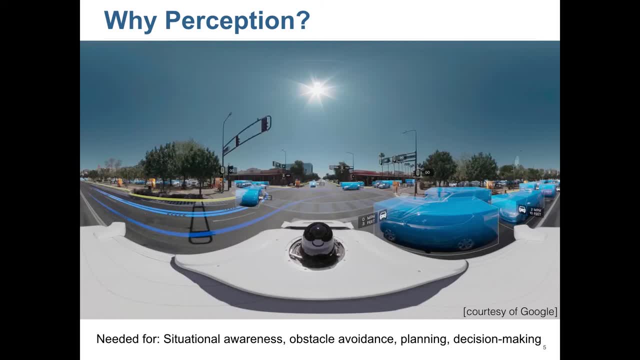 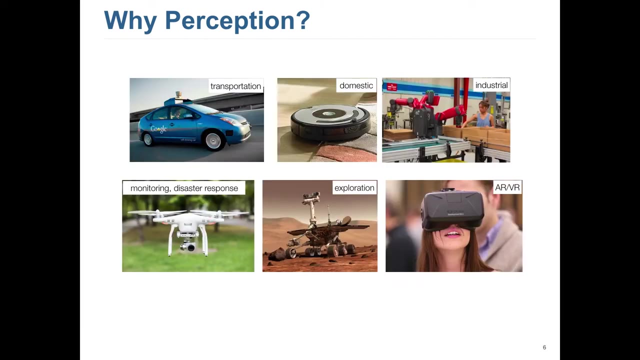 intentions of the other cars. Well, these are all perception problems. okay, and in general, beside this application, perception is needed for situational awareness, obstacle avoidance and to support planning and decision making. Beyond the example of self-driving cars, it turns out that recent advances in algorithms and computation for perception are making 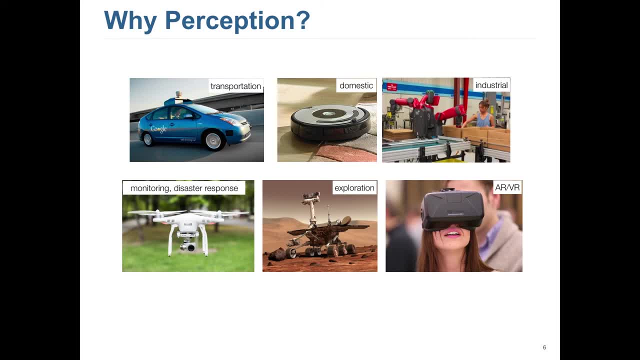 possible a broad number of applications. So perception algorithms is steadily transitioning from academic research to products, and you can see these in domestic robotics, application, industrial robotics, search and rescue and disaster response with drones, and even application and tradition are not associated with robotics like virtual and augmented reality, So the good thing. 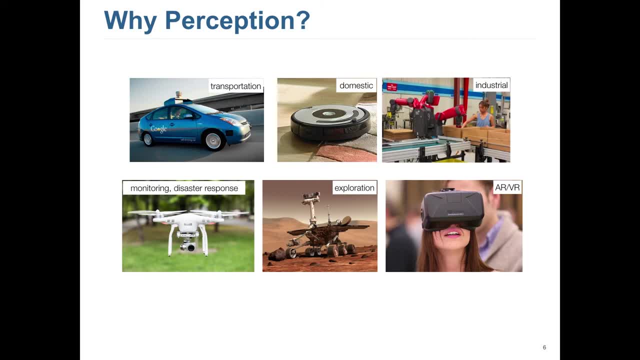 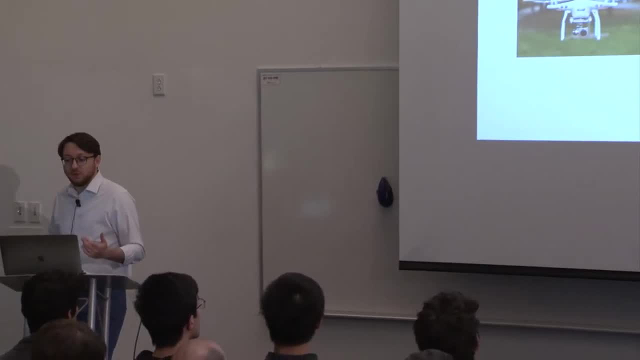 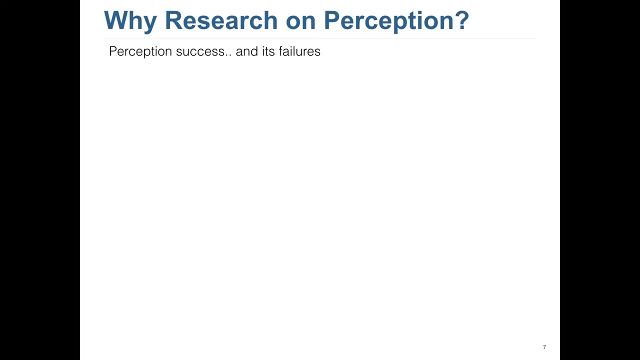 is that whatever research we are doing in robotics nowadays is having a huge impact on societies, getting really a practical impact on society. The bad news is that the broad adoption of these technologies is also showcasing a number of limitations of existing algorithms and, in particular, you guys might be. 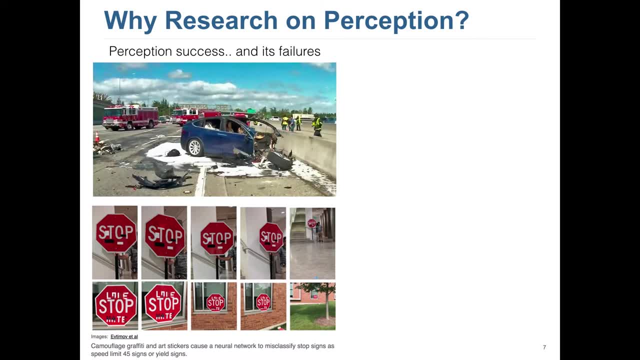 familiar with a number of failure modes here. This is a Tesla accident in 2018 in which the computer vision system misclassified the concrete obstacle here on the left and decided to turn into the obstacle just because of a failure of the perception of the computer vision system. and this is another popular 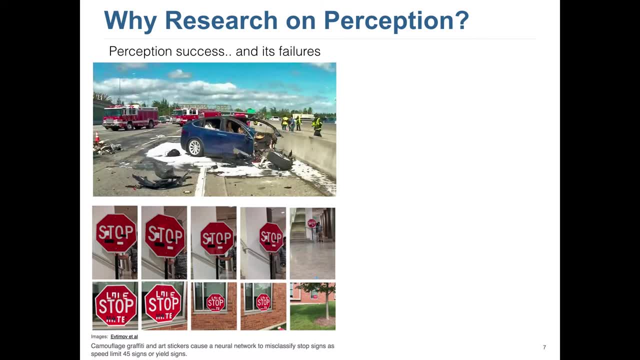 example, How many of you have seen this Good portion? Okay, so this is a case in which stop sign in nominal condition and neural net is able to detect and classify a stop sign, but if you carefully place these markers on top of the stop sign, 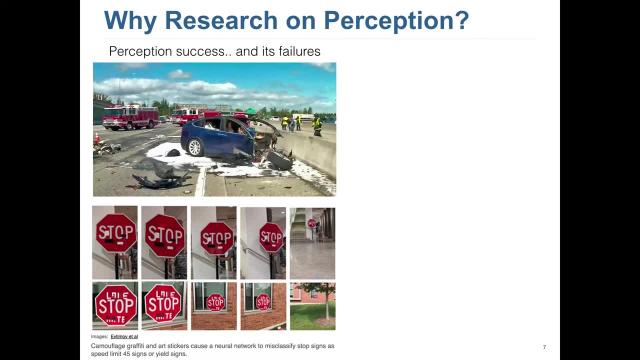 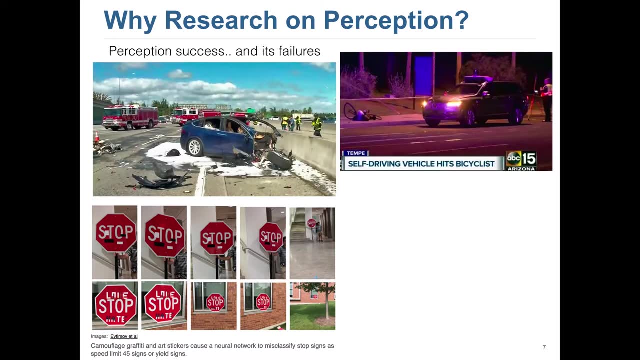 you can mislead a neural network to think that this is a 45 mile per hour speed limit, which is a pretty bad mistake to make an intersection, And there are multiple examples. So failure also in problems related to object detection, object classification, pedestrian detection. One thing that is quite surprising is that even very 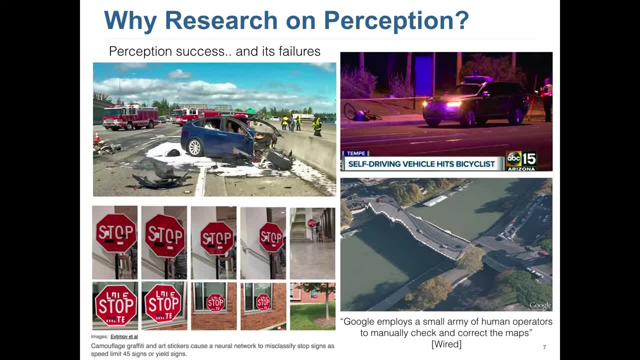 established products like Google Street View. if you spend enough time on the internet, you will find examples of failures of Google Street View, as in this case, and it turns out that Google has a huge amount of people just in charge of verify and sanity, checking the maps and fixing them manually. Okay, so, 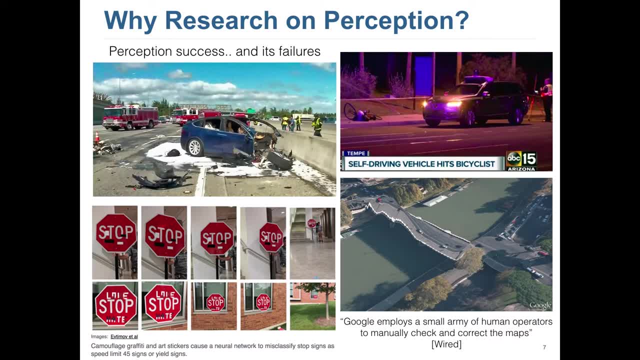 what I want to say here is that, despite the fact that this technology is starting to have an impact on many practical application, there are still fundamental limits, and ideally there is. we really would like to go beyond this kind of manual human supervision. Okay, so so far I should be. should have convinced you. 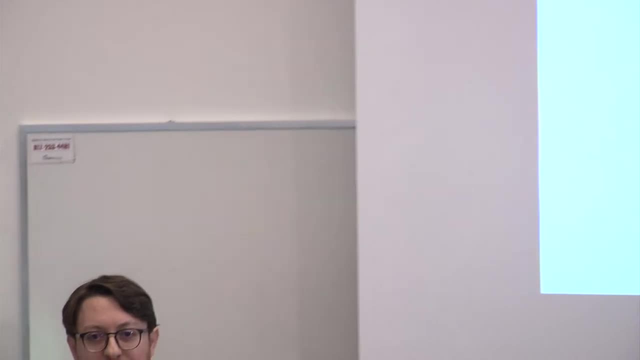 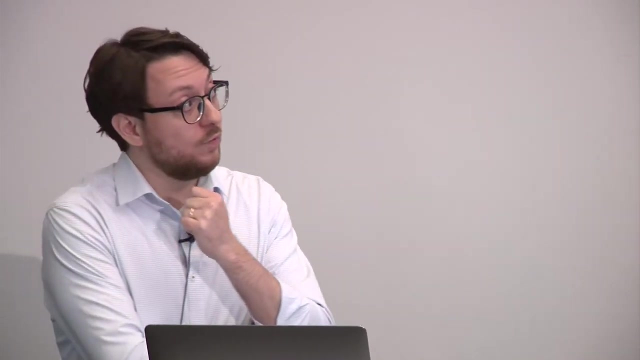 guys that perception is important for robotics, and what I want to do in the rest of this talk really is two things. I want to go over a number of key challenges in perception. I want to give you like a broad overview of what are the key. 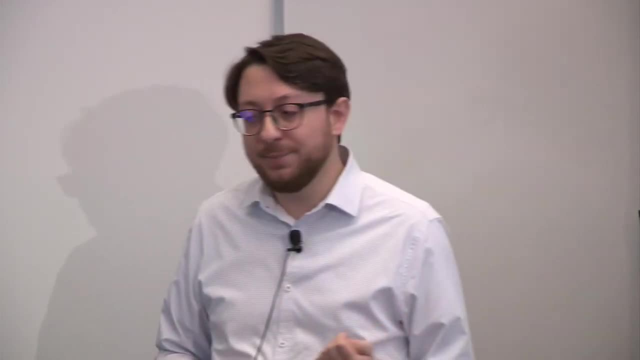 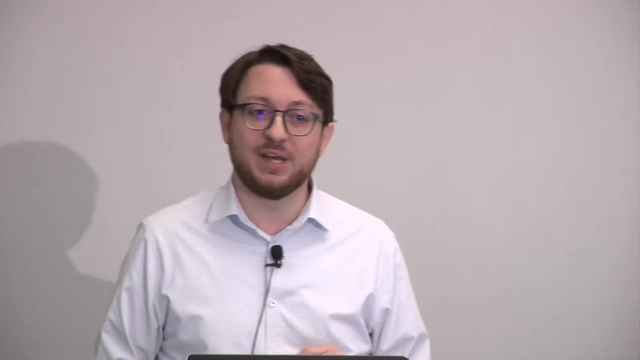 challenges, which is also an excuse to tell you about the work that you are doing in my lab. And the second part of the talk is really about focusing on a specific challenge which is outlier robust spatial perception, and tell you about two contributions: recent contribution from my group, which I'm 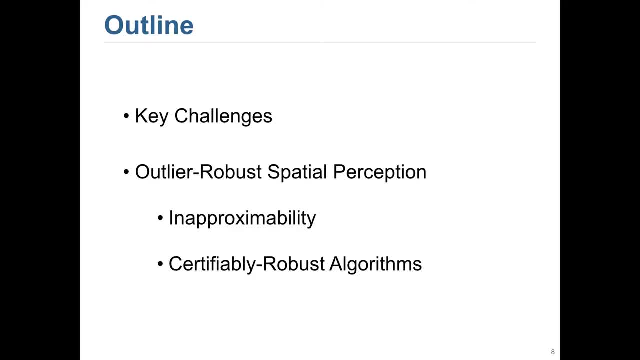 very excited about. Feel free to stop me at any point. So let's start with key challenges. So in my opinion, a good way to think about key challenges is to think about what are the axes of complexity, of perception, And here I'm putting like: 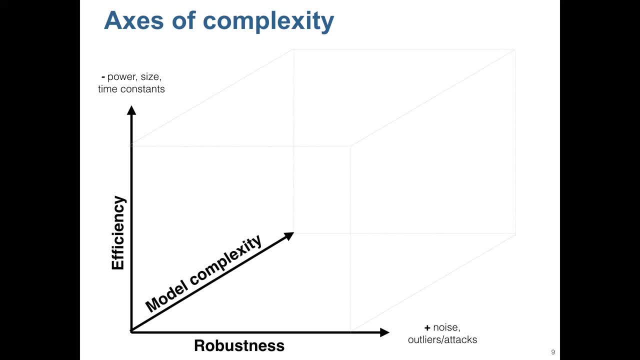 three main axes of complexity: robustness, efficiency, model complexity. You can imagine that if we go along the robustness axis from left to right, we are trying to design algorithms which are more and more robust to noise outliers attacks. If we go along the efficiency axis, we are trying to design algorithms 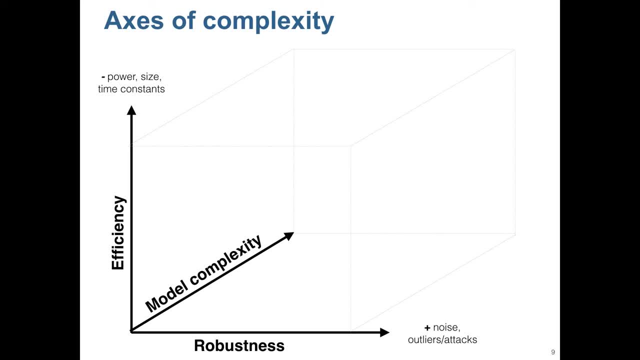 which are more and more efficient. So they take less power, they require less. you know, smaller hardwares, machines, but still lower levelANS horas. so in this葬, or they are just faster. The third axis is a little bit less intuitive. 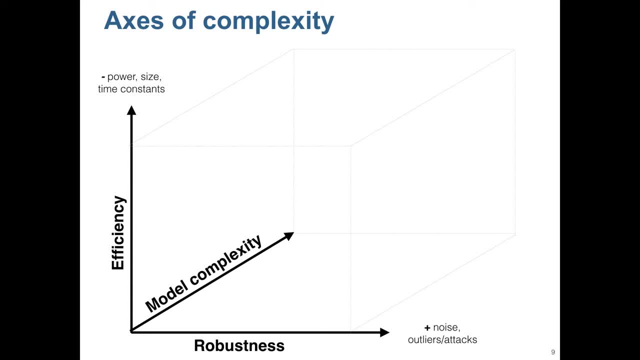 it's about model complexity. So you can imagine that as you go along this axis you are building richer and richer representation of the world. So here you are building a very simple model of the world. here you have, like a very rich understanding of the external environment. 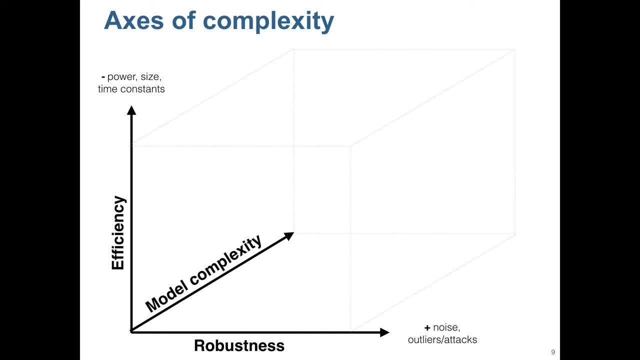 To understand a bit better this axis of complexity. let's try to populate these with few examples just for the sake of the exercise, And you can imagine that human perception is probably up there. Human perception is a pretty efficient perception system. The human brain works on 20 watts. 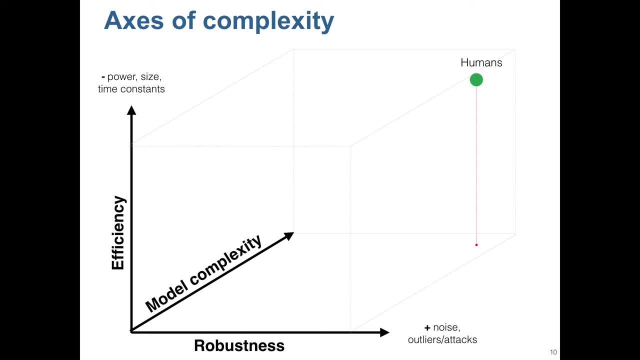 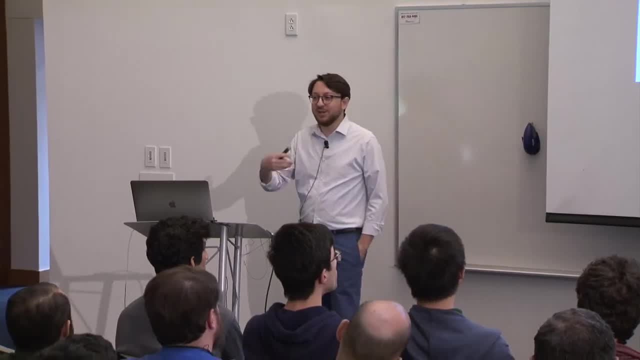 which is a very good, very efficient embedded system, And robustness is also pretty good. I can show you optical illusion to trick your perception system, but in general it's pretty hard to confuse you like with your perception system is pretty robust. 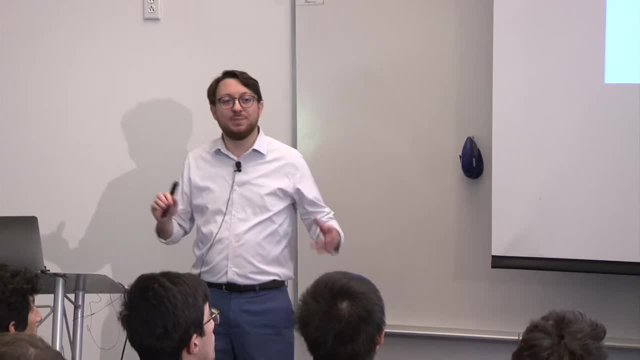 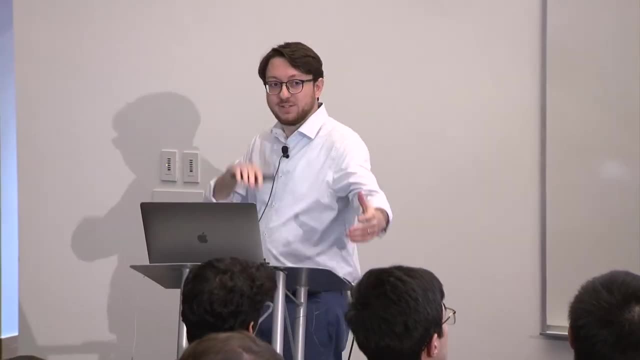 And, of course, you have a very rich representation of the world. You can imagine that if you close your eyes, you have a very complex model of the environment around you in terms of the geometry, presence of people and so on. If you try to repeat the same exercise. 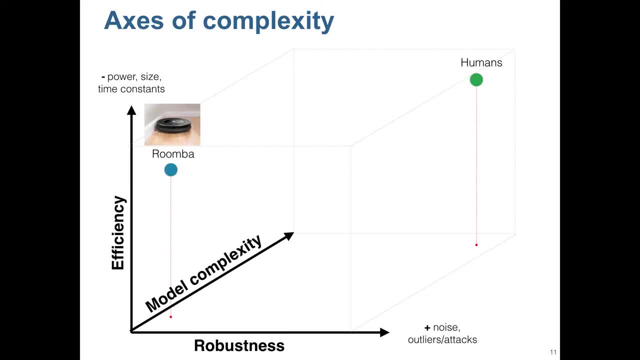 for the state of the art in robotics. you can start with the Roomba. very popular robot Turns out that the Roomba is as efficient as a human. The Roomba is probably 28 watts power consumption, which is comparable to the human brain. 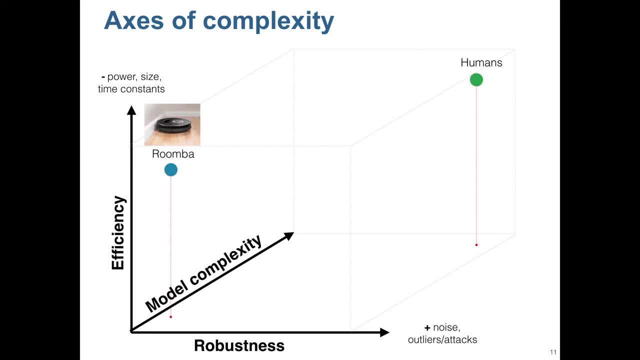 And that's a bit disappointing, I guess, as a data point, but And in terms of robustness, of course you know the Roomba is not designed really, it's designed to be cheap, it's not designed to be very robust. 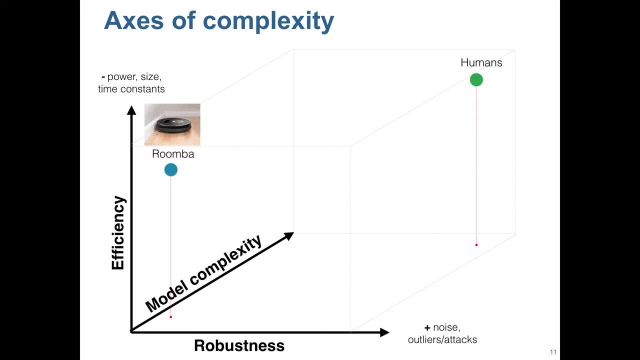 or to build a complex representation of the world. Other data points: state of the art in drone technology: the Sky-DR1 drone more expensive, so we get like a more complicated representation of the world. Extra robustness because you don't want to break this project: $2,000,. 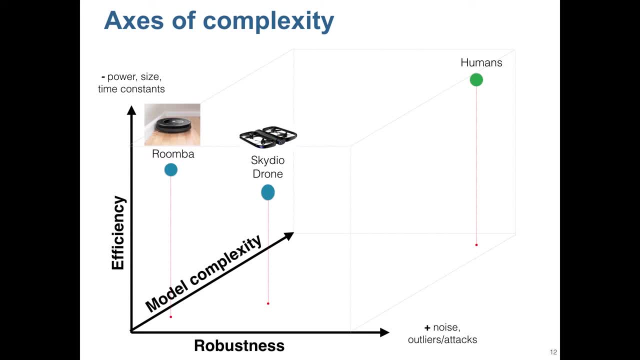 and that will come at a price of efficiency. You iterate this exercise. you put here self-driving cars, Google Drive, street view And by interpolating these data points, what you can see is that there is a very intuitive trade-off here going on. The intuitive trade-off is that 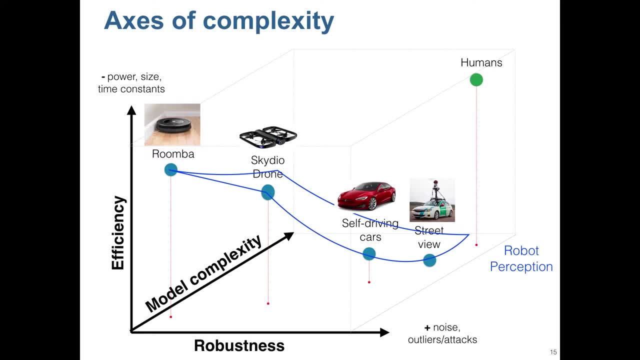 nowadays, in robotics, if you try to design systems which are more robust and gets a more complex representation of the environment, the efficiency of the system goes down, which is a very intuitive trade-off, right. The thing that is interesting is that humans somehow are defying this trade-off, or are just 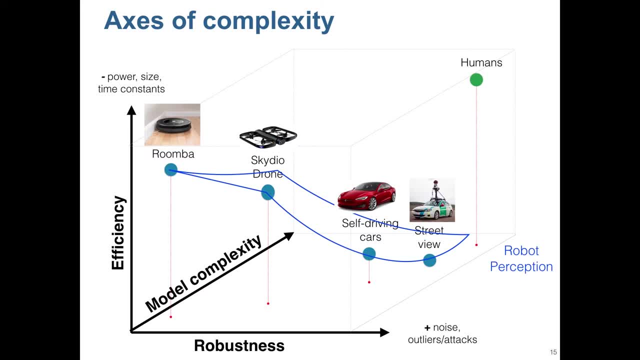 finding a much better Pareto curve out there And really the goal of my lab- and I believe part of the goal of people doing perception in general- is about bridging this gap right now. So in my lab we're working really across all the spectrum. 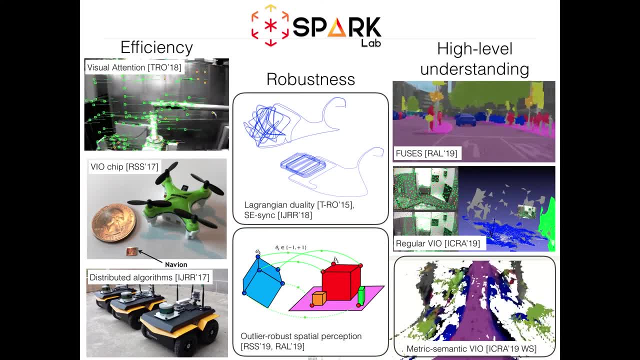 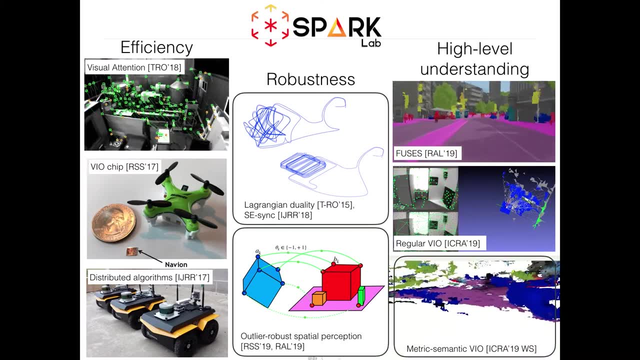 along these three axes, pushing the boundary along these three axes, and I want to tell you about- you know a few things about work we are doing in efficiency to improve efficiency, robustness and high-level understanding In terms of efficiency. we're exploring. 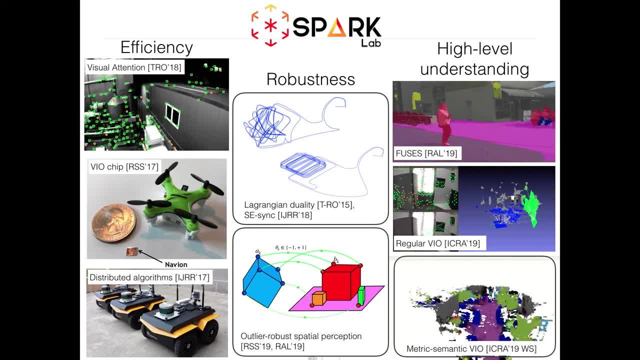 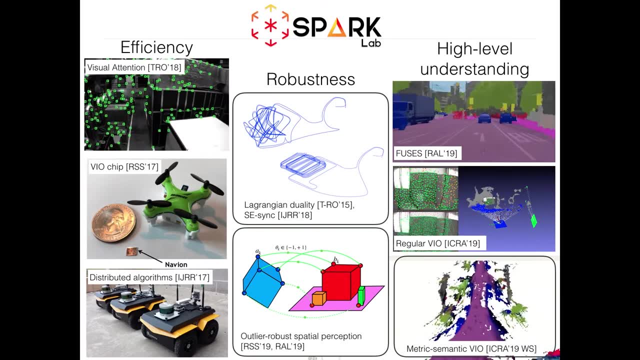 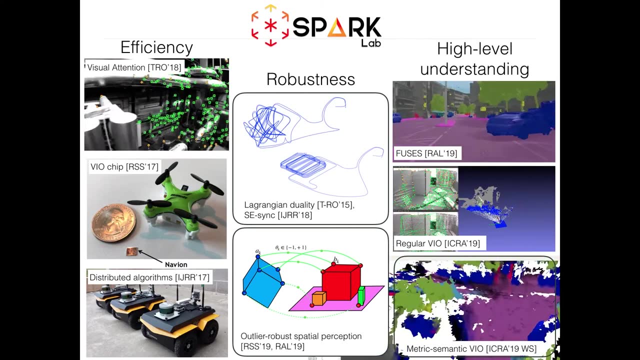 this notion of visual attention, The basic idea, that is, that the key to be efficient is to be very selective. You are not efficient by processing every bit of data. you are efficient by selecting what are the subset of bits that you really care about, which is the notion of attention. 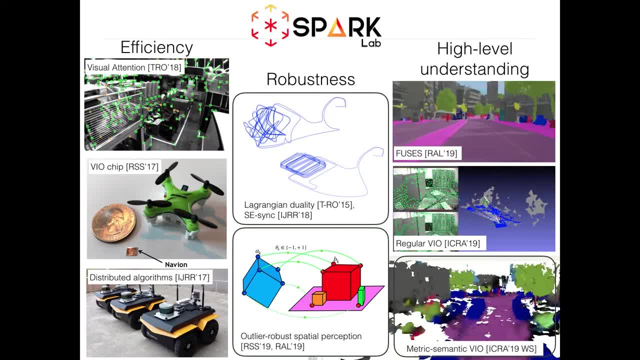 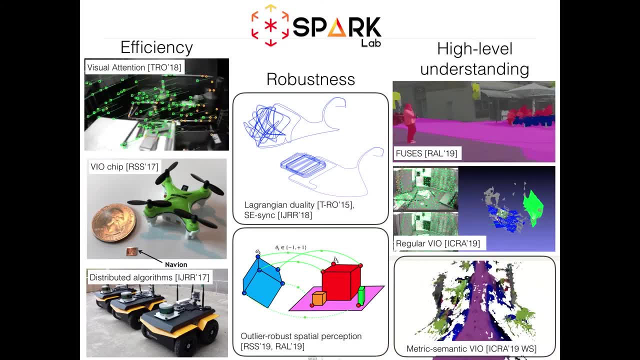 in humans. okay, We've been working on a notion of visual attention, for example for SLAM or visual inertial navigation along, you know, the efficiency axes. we have been pushing the boundary also with the contribution, which are not really algorithmic. 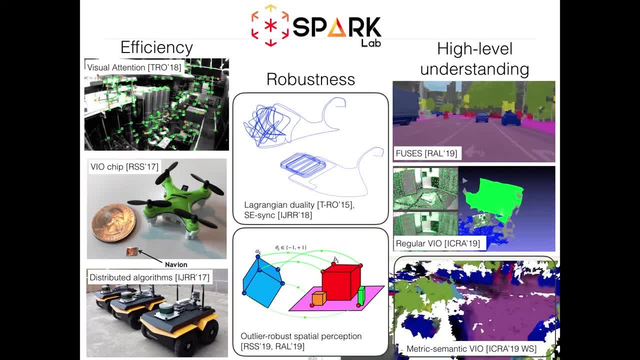 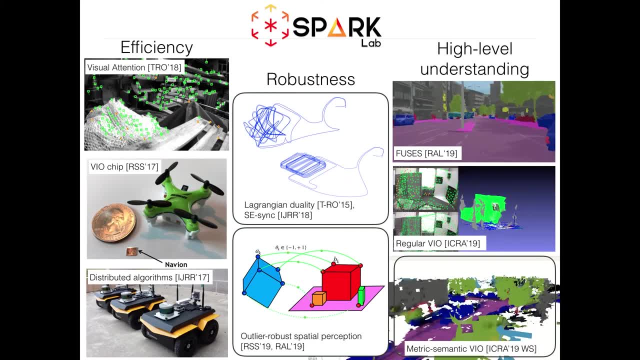 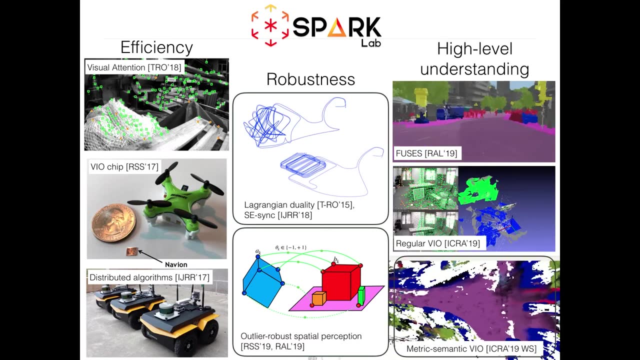 but are really about chip design in collaboration with the other faculty at MIT. And, of course, you can think about the notion of efficiency being applied also to multi-robot system. In this case, being efficient means really reduce the amount of communication that you have in multi-robot system. 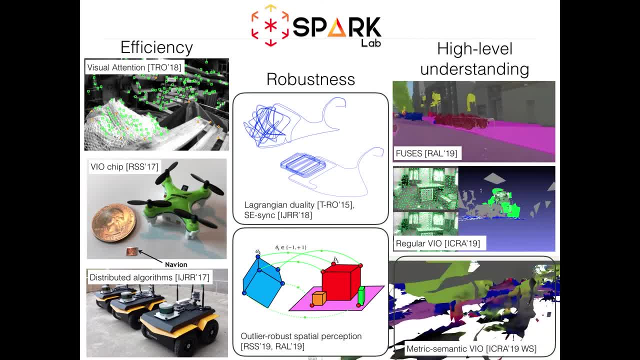 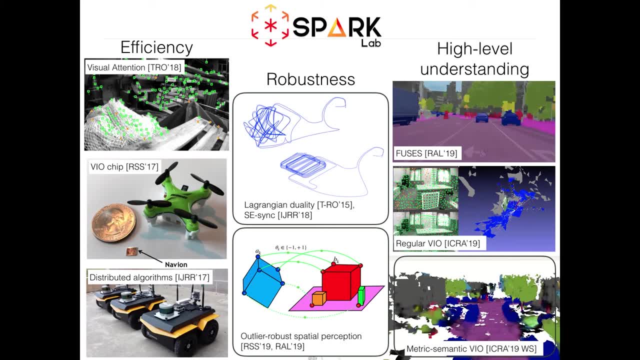 to get essentially multi-robot mapping in this case Put a lot of work on. robustness, I believe, is one of the key problem, the key issues here, And we investigated robustness in particular in SLAM problems, robustness to large noise and outliers. 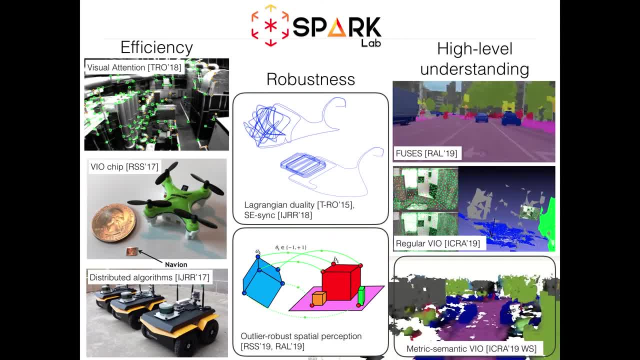 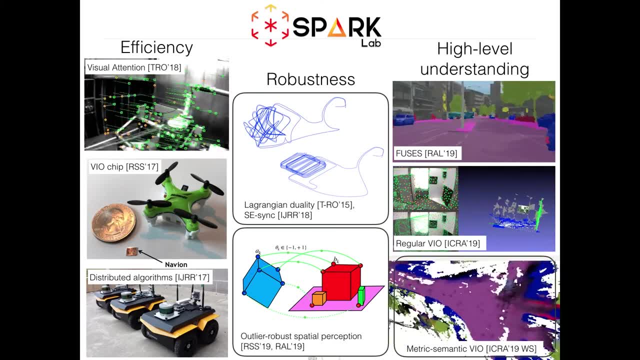 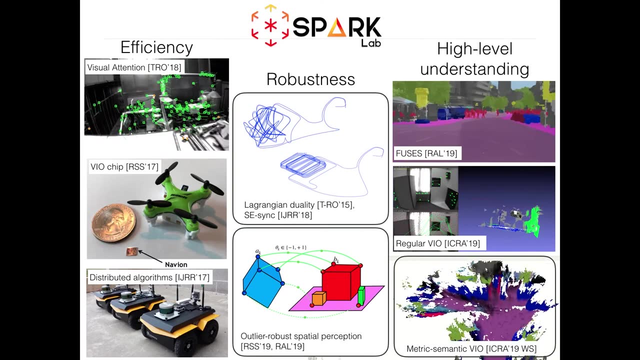 And these will be essentially the topic of today's talk- And we are getting more and more interested in high-level understanding, So we are looking at how to be clever in formulating optimization problem. to get very fast: 2D semantic segmentation and 3D semantic reconstruction. 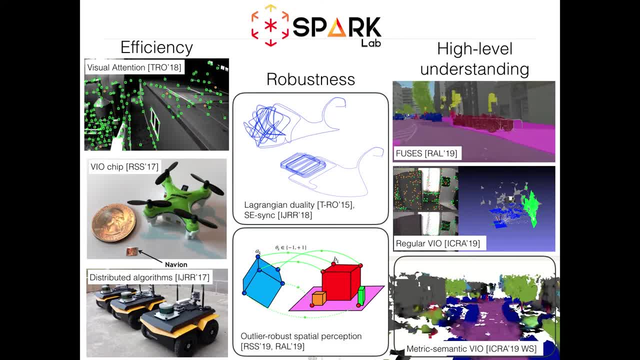 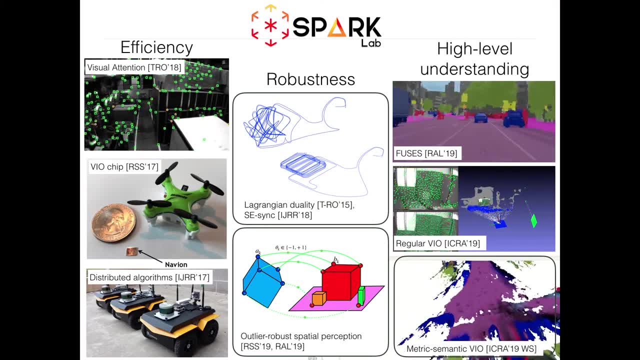 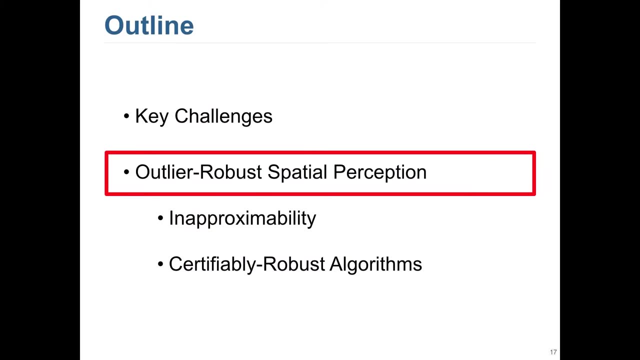 These are just a couple of examples. What we really want to do eventually is to understand how to exploit semantic understanding to improve 3D reconstruction of the environment. OK, so let's jump right in the topic, the technical topic of the talk. 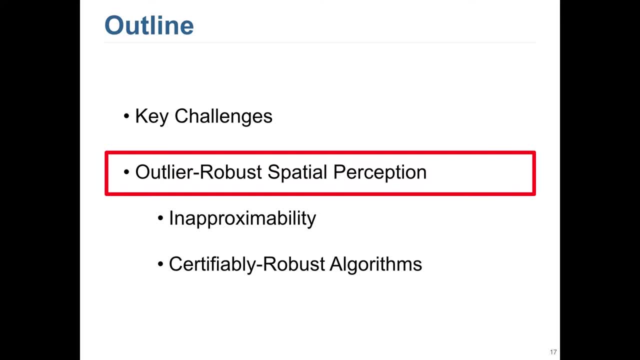 Today I'm going to talk about outlier robust spatial perception And I'm going to touch on two main contribution one which is about some fundamental property of the outlier robust spatial perception problem And the other one is propositional And I'm going to talk a little bit more about some of the 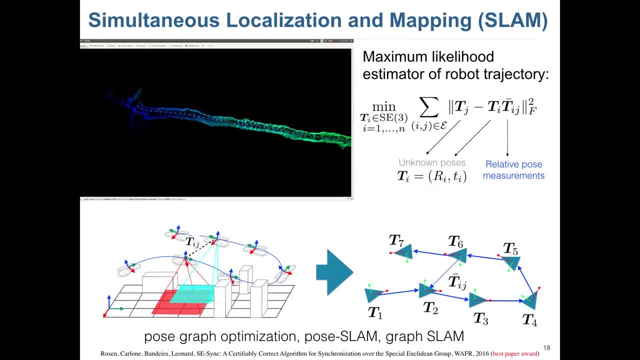 things that we are using algorithms to solve it. So why do we care about outliers? Why is it important to deal with outliers? when you do spatial perception, I want to convince you that outliers are very important to analyze, to investigate in the context of the simultaneous localization and mapping problem. 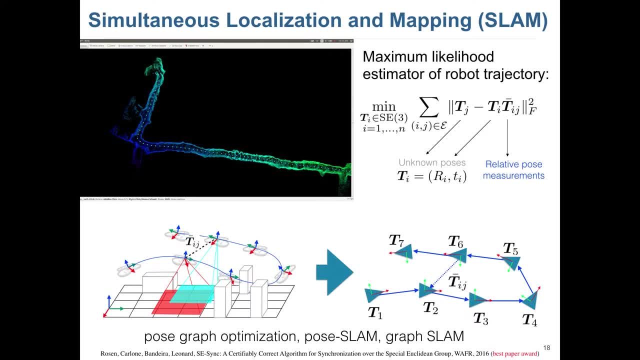 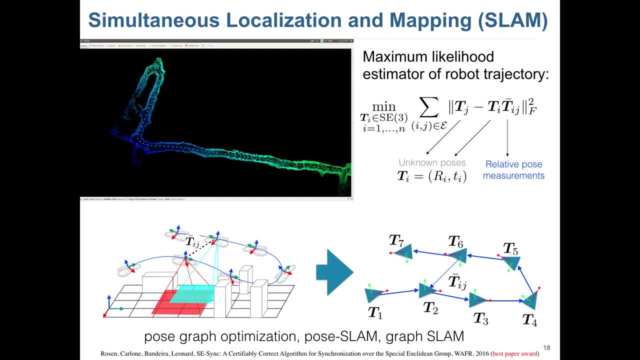 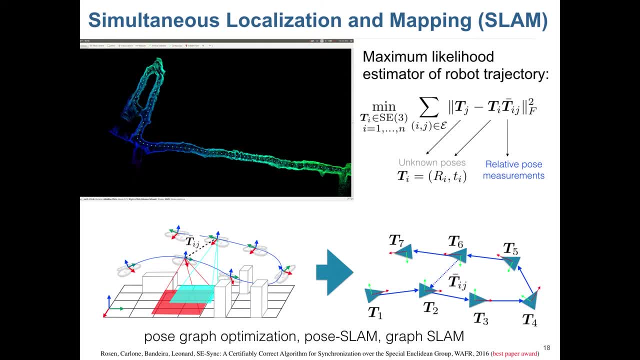 this 3D reconstruction of the environment, But really in the background of a SLAM system. what ends up happening is that you're trying to solve an optimization problem. This is what is called the maximum likelihood estimator. This is what is called the maximum likelihood estimator. 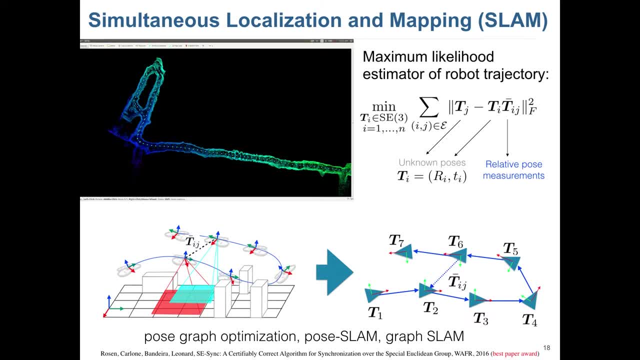 You solve this optimization problem to get an estimate of the trajectory of the robot. And once this trajectory of the robot is reconstructed, it is easy to build a map on top of it. So this optimization problem is not trying to compute a set of poses, TI. 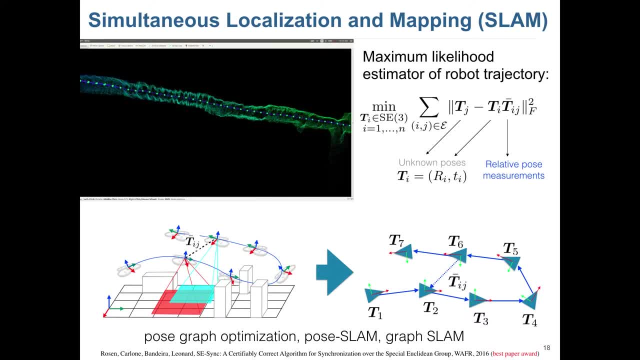 poses, position and orientation. and imagine that these poses are dropped along the trajectory of the robot And it's doing so by minimizing a non-linear, least square problem in which the TIJ bar are the given measurements. So you try to compute a set of poses. 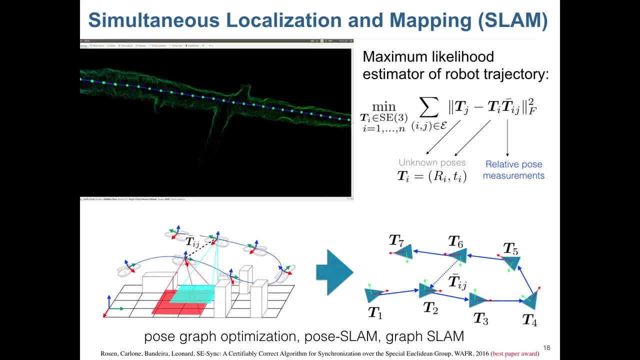 along the trajectory of the robot, given these relative pose measurements. So where do we get these relative pose measurements? Let me try to explain using this figure here. Imagine that you have a robot again traversing a completely unknown environment. We really would like to figure out. 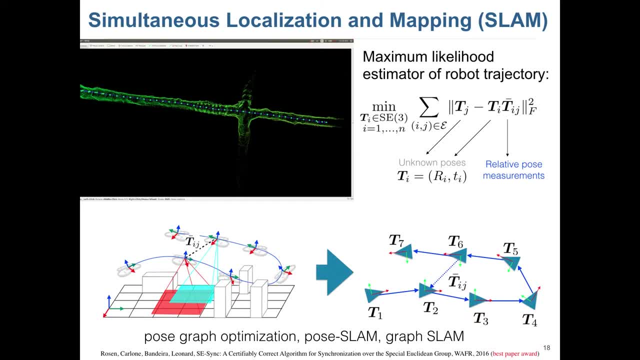 the trajectory of the robot as a discrete set of poses And what we can do is that we can compare sensor data at pose I and J and somehow we can do some magic trick, We can apply some algorithm to compare this sensor data and out of the comparison of these two sensor data, 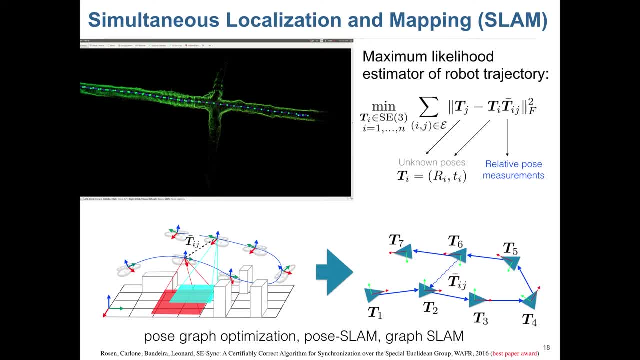 we can get the relative pose estimate, TIJ bar, which is the relative pose between pose I and J bar, And really, SLAM is about figuring out the trajectory of the robot given all these relative pose measurements. You can visualize this problem as a graph. 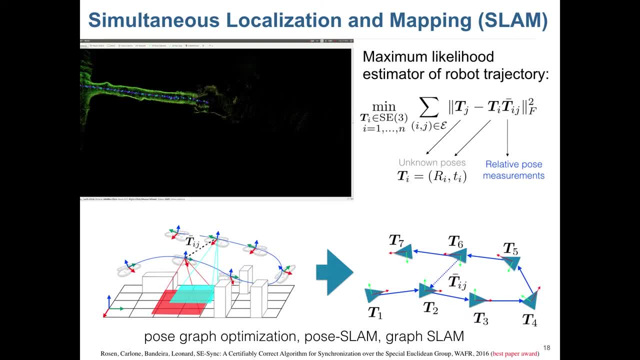 in which you have a measurement for each age in the graph- That's the TIJ- and you want to figure out quantities poses at the node of the graph. These are the T1 to T7 in this case. So this is a standard SLAM problem. 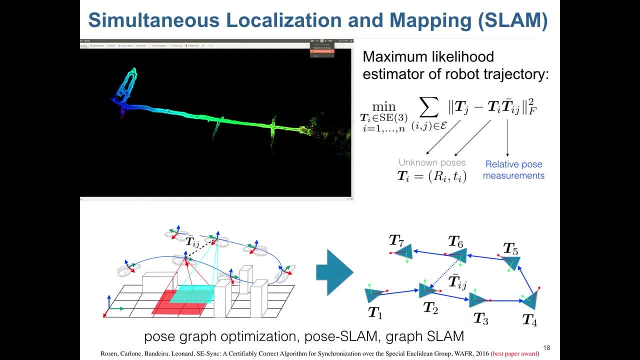 It's one of the most common problems in the world. It's one of the most popular formulation for SLAM, which is known as pose graph optimization, pose SLAM or graph SLAM, And really, given the TIJ- assuming that the quality of the TIJ is good in some sense- 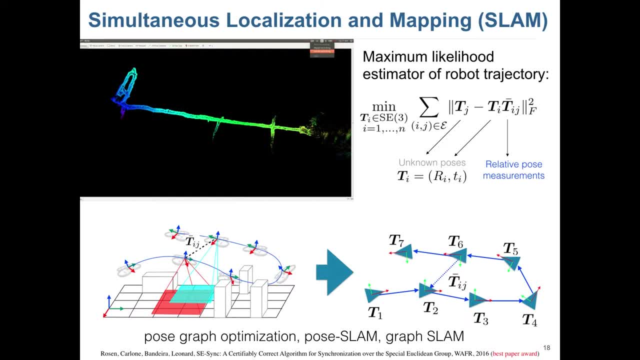 this problem can be considered solved. It's well understood how to do this optimization, to solve this optimization problem, even though this is a non-convex problem, because the set SC3 is a non-convex set. The set SC3 is a set of 3D poses. 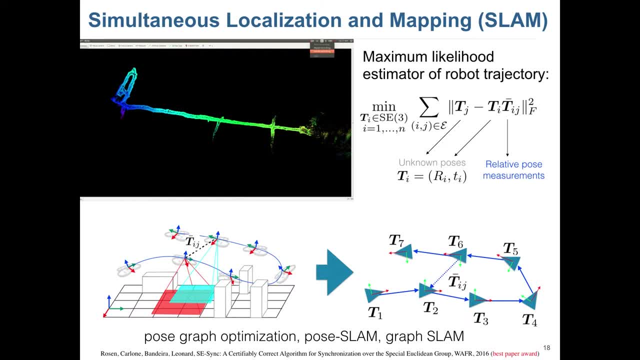 And even though the cost of this problem is high, the cost function here is just a quadratic function of the poses. the non-convex of these makes these a challenging problem, But it's well understood by now how to solve it. So the challenge here appears when we want to do SLAM. 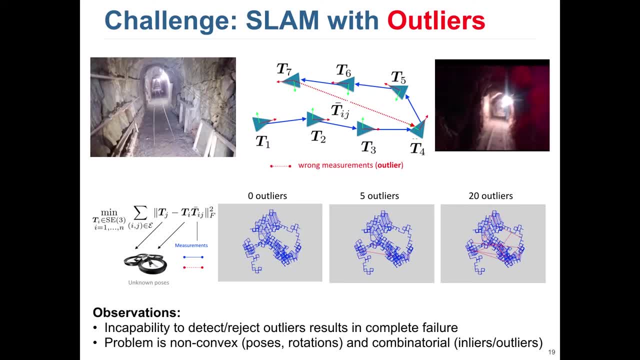 in the presence of outliers. Outliers clearly are bad measurements, and where do these bad measurements come from? So imagine that I'm exploring the cave. so my robot is exploring this cave. It's starting at some pose T1.. It's moving at pose T2, T3, T4.. 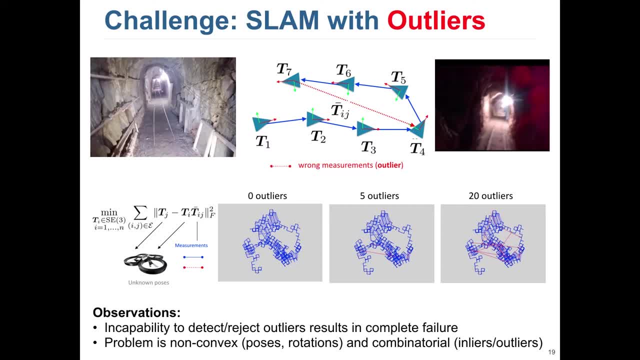 At pose T4, it's taking this sensor measurement. It's taking, let's say, this image of the cave, And then it keeps going. It keeps walking along the trajectory going to T5,, T6, and T7.. 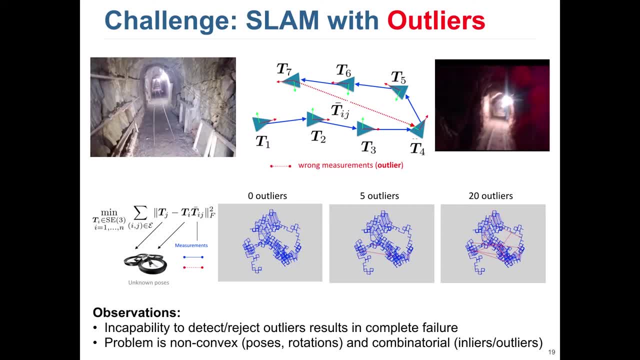 I arrived at pose T7. The robot is collecting another image of the environment And, just by coincidence, this image really looks like it's a cave. really looks like the other one that we collected at T4. Even though these are two completely different places, 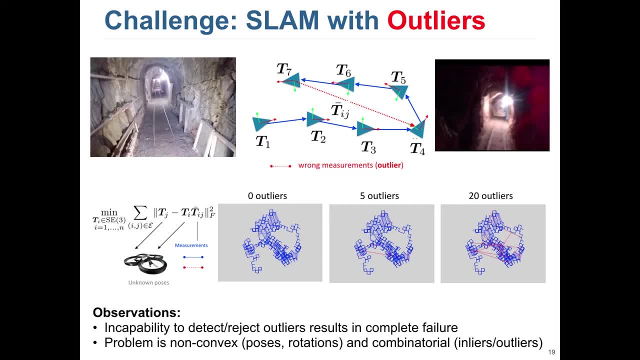 So the robot is confused to think, is misled to think, that this part of the environment is the same as that just because they look similar, And what it's trying to do is to enforce a relative measurement within these two poses, even though these two poses are really far away. 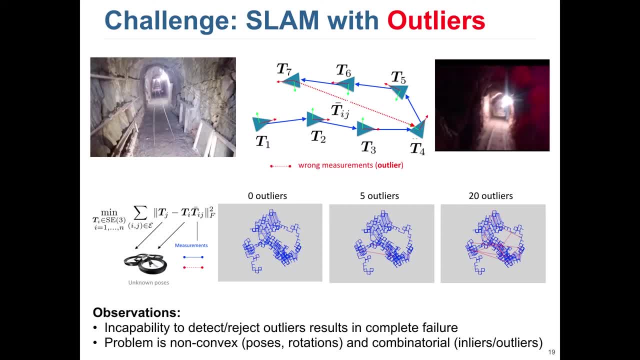 They have nothing to do with each other. So this is what is called an outlier And, by the way, that's very similar to what happens for humans If you walk, If you walk in a cave and your place recognition system fails. 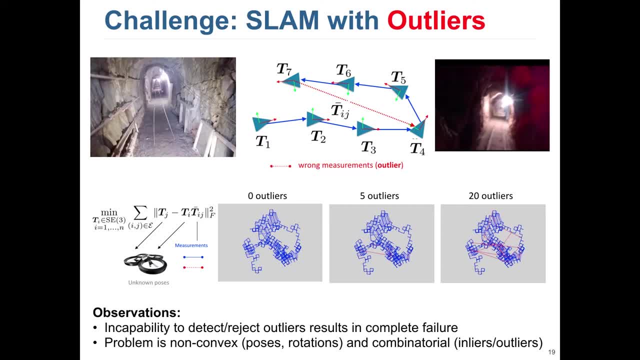 you can just get lost for the same principle here. So why this kind of phenomenon? which have outliers? Why is this a problem? Well, if you feed an outlier to the optimization problem, I want to show you what happens. So let's start with the case in which you 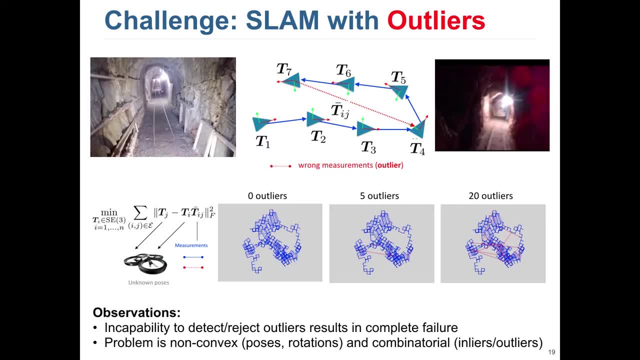 have a bunch of measurements, tij bar, and there is no outlier, So they're all good in some sense, meaning that they have Gaussian noise essentially Without outliers. you solve this optimization problem and you get the reconstruction of the trajectory of the robot. 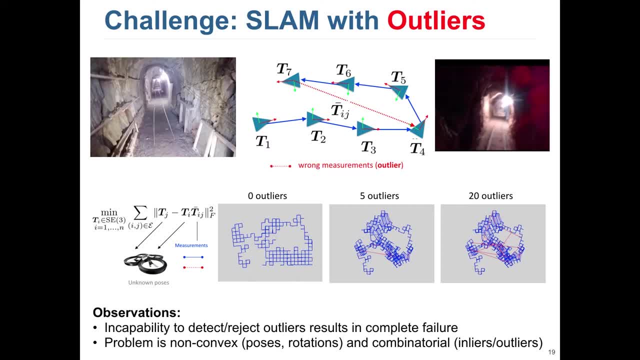 This is a discrete set of poses, but I'm just visualizing it as a continuous trajectory And I can guarantee that that's the right reconstruction of the trajectory. That's how the trajectory looks like Now. the problem is that if I just add five outliers, five random outliers- 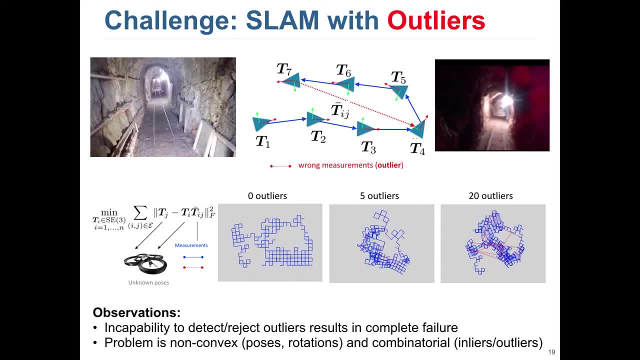 to this set of measurements, the same trajectory. I feed five outliers to this problem I try to solve and I get this reconstruction And I get this reconstruction of the trajectory which is completely different from the actual trajectory of the robot. So I'm not really able to get a good reconstruction. 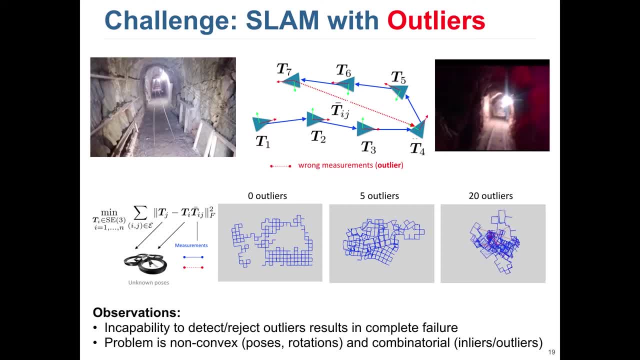 of the environment, If I have 20 outliers over a total number of measurements which is around 3,000 measurements, so it's a huge number of measurements and a small portion of outlier, you can see that the reconstruction of the trajectory is completely off. 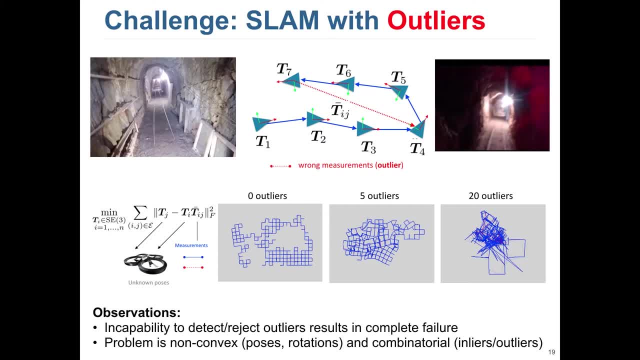 So two observations here. The first observation is that the incapability to detect outlier results in complete failure. You can see this from here- And the other observation is that we started with a problem that was already non-convex because of the presence of poses and so on. 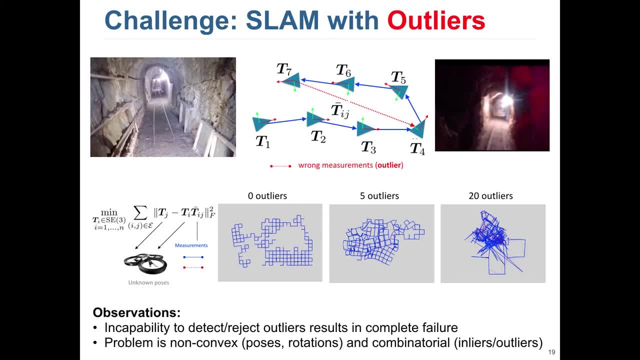 And now, with the presence of outliers, it's even combinatorial, because somehow you have to figure out which one is in liar and which one is outlier. So there is a combinatorial nature. So this makes for a really tough problem to solve. 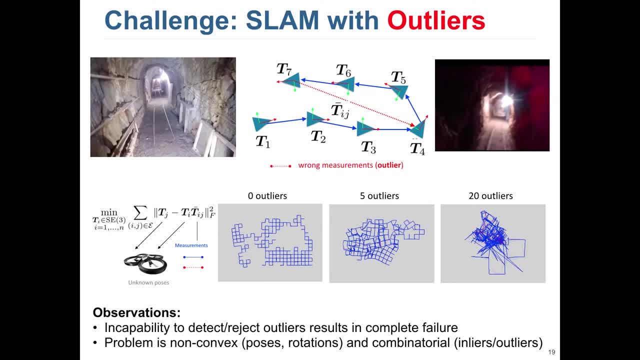 Is it clear even what problem you are trying to solve? Can you write down the? Yeah, We write it down in a few slides. Yeah, Yeah, But the bottom line here is that these definitely will not give the right solution. OK, 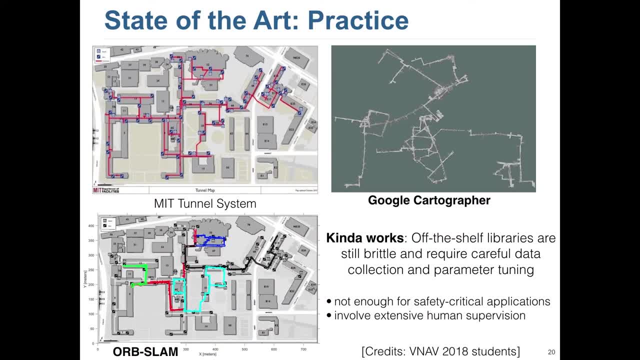 So before trying to write it down, we'd like to see what happens in practice, how essentially existing libraries are dealing with these problem of outliers and if this is really a problem. So what we tried here as part of the graduate class I was teaching last fall is to try to use a little bit. 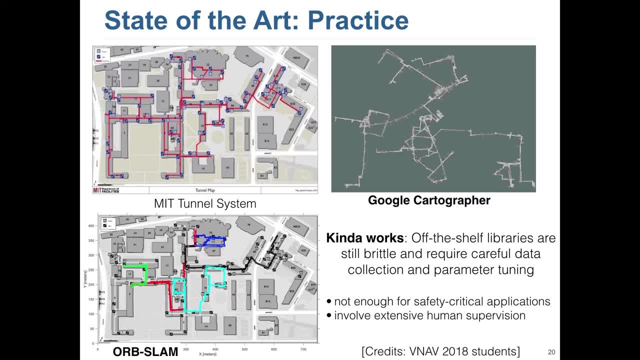 of mapping of the MIT tunnel system using existing state-of-the-art tools for SLAM. So we used Google Cartographer and Orb-SLAM to do this exercise in mapping, And what happens is that if you just try it without spending too much time on the tool, you just 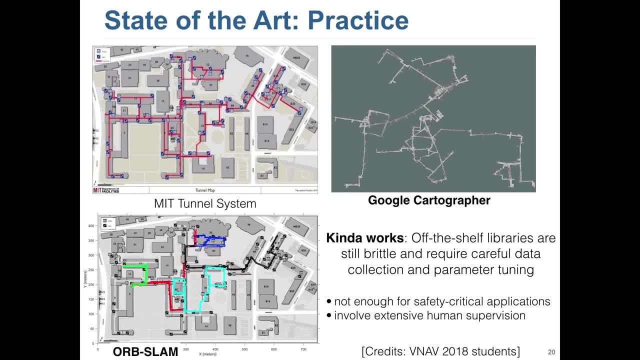 try doing mapping with Google Cartographer. you get this type of map instead of the actual map of the MIT tunnel. Who did this? Did it be enough? Yep, So Chris knows about this. If you spend more time here, you're going to have a problem. 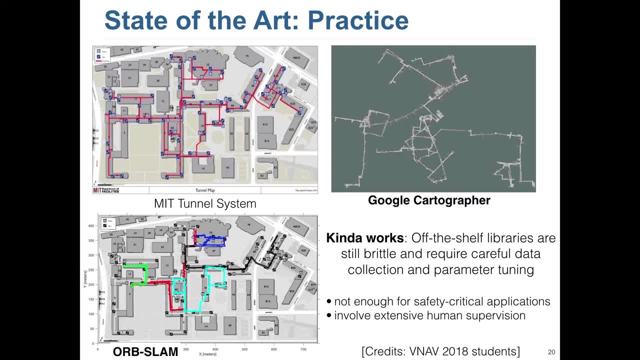 Yeah, If you spend more time here, instead you use Orb-SLAM and you spend more time and do a lot of parameter tuning and very careful data collection, you can get a much better map here. You can see the different segments and so on. 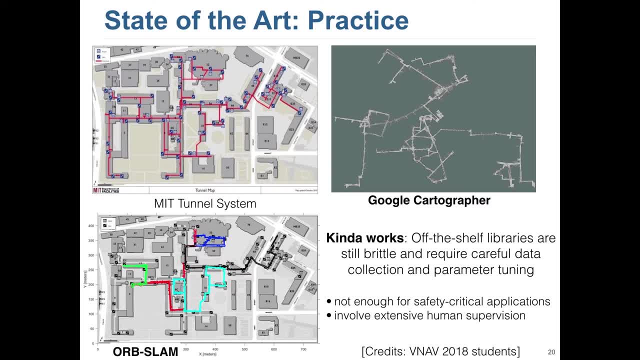 This actually is still off a little bit but looks pretty good overall And that to me is really the status of the SLAM problem and many spatial perception problem. So the state-of-the-art is that algorithm kind of work in the sense that if you spend a lot of time, 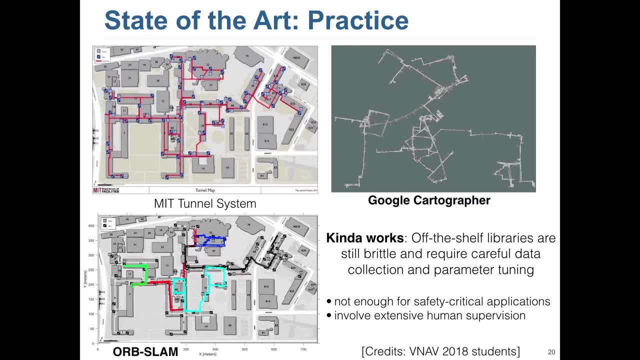 doing parameter tuning and you are really careful in the way you collect the data, you can get reasonable results. But unfortunately my point is that kind of work is not a good answer if you're dealing with safety-critical application And also it's not a good thing that we 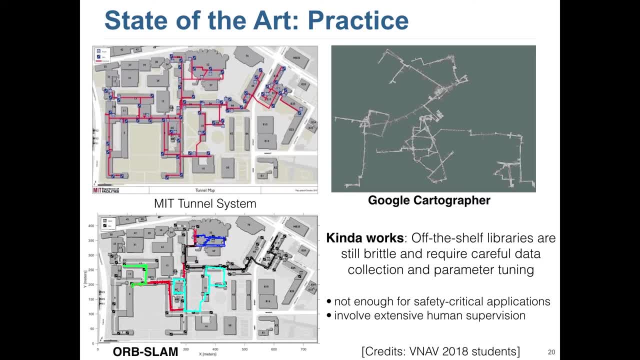 have to be so careful in collecting the data to have a good result. It's like we don't want to work too fast because, essentially, our perception system can get lost. Doesn't make sense. We don't want robots to be like that. 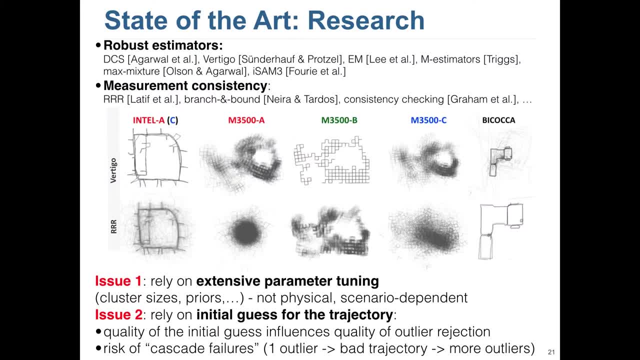 We can look quickly at what is the state-of-the-art instead on the research side. on the academic side, I'm listing two sets of works. There is a lot of work done, So two sets of work I'm listing is about using robust estimation in conjunction. 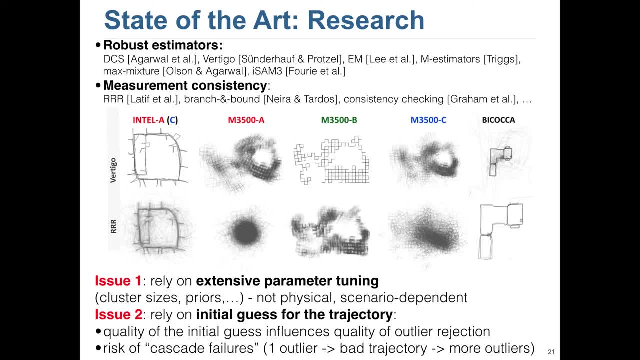 with some nonlinear optimization technique or looking at measurement consistency, And I don't want you guys to parse too much out of these, but these are examples of failure modes of two existing algorithms, Vertigo and RRR. The issue that I have with the RRR 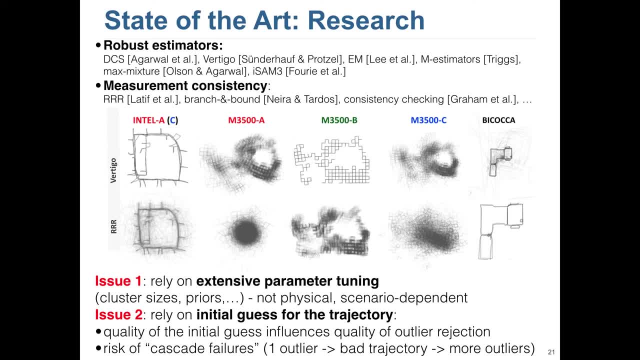 the state-of-the-art are these two aspects. First of all, again we have this issue that existing algorithms rely on existing and extensive parameter tuning, And parameter tuning is not bad in general, But the problem with parameter tuning is that in this case, 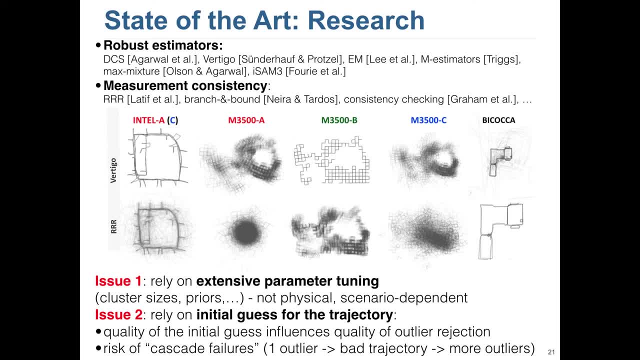 the parameters you have to tune do not have a physical meaning, which means you have no guideline on how to tune them. And the second aspect is that the parameter tuning is scenario-dependent, meaning that if I have to run my robot at MIT, spend two days doing parameter. 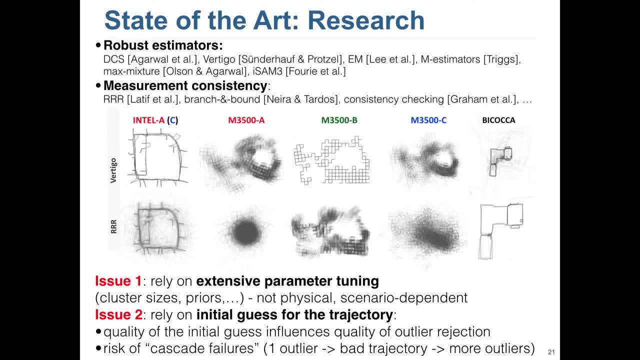 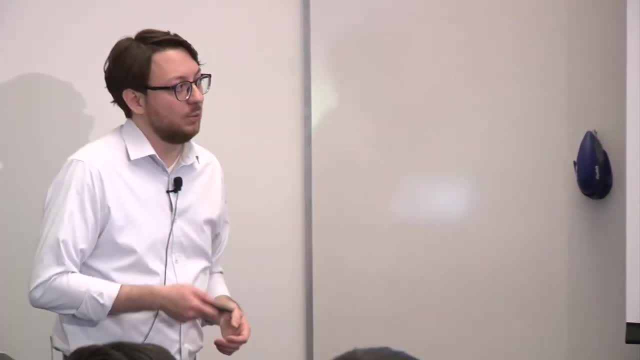 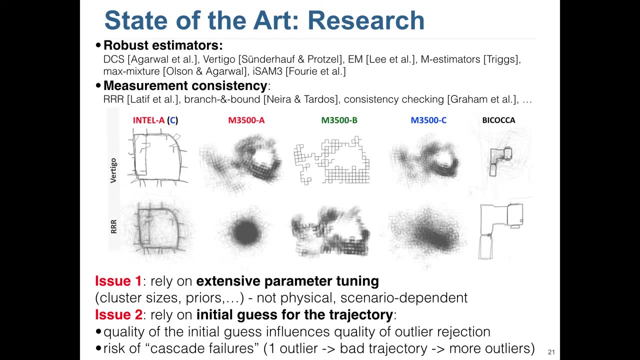 tuning, Then I go at another place, and that doesn't work. The second issue is that most of these algorithms rely on some iterative optimization technique, which require an initial guess for the trajectory, And so the quality of the result really depends on the quality of this initial guess. 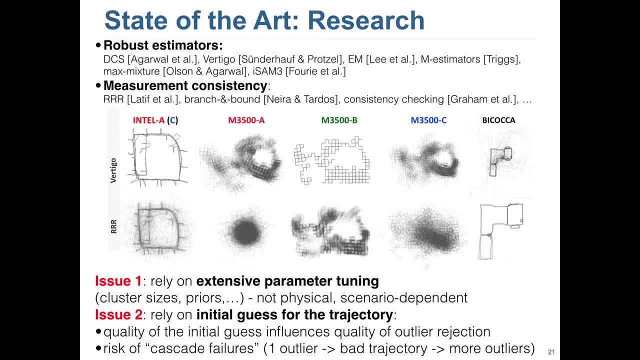 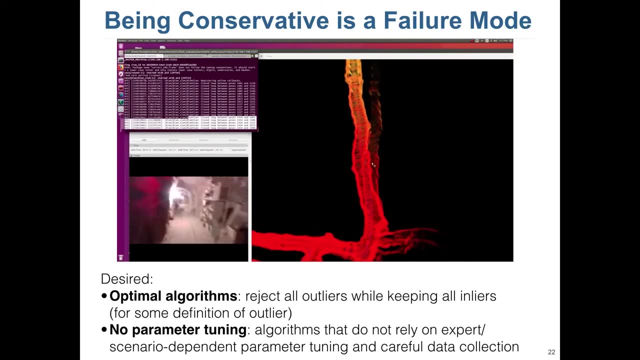 And there is this risk of cascade failure in which, if at some point you accept a single outlier, your trajectory guess gets much worse and you tend to accept more and more outliers. So you just cascade, You just have a cascade failure. What I want to stress, finishing with the motivation: 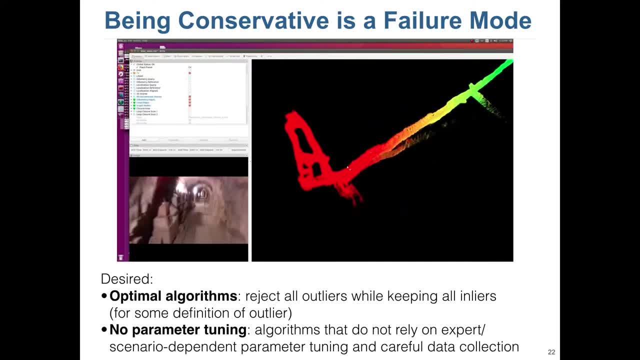 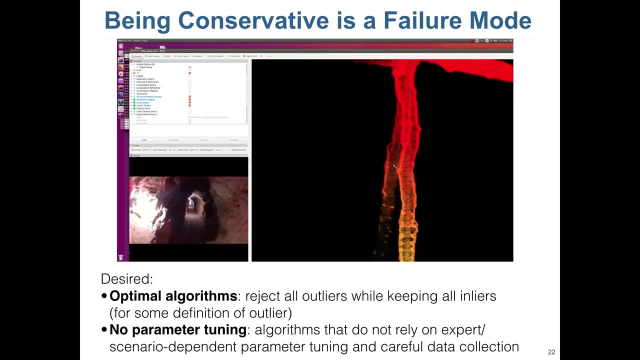 for what we want to do is that being conservative here is a failure mode, in the sense that it's not only a failure to accept outliers, because that leads to wrong trajectory estimates and other failures. being incapable of capturing in layers, For example, these are another experiments. 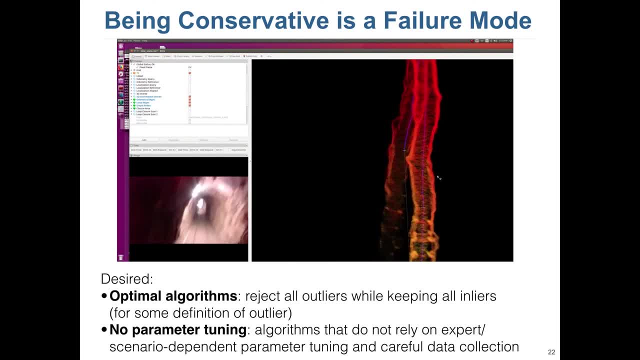 for the DARPA Subterranean Challenge And we spent so much time doing parameter tuning and making sure that we didn't get outliers in our estimate that the robot is really trying to force measurements, saying that this corridor is the same as that corridor. 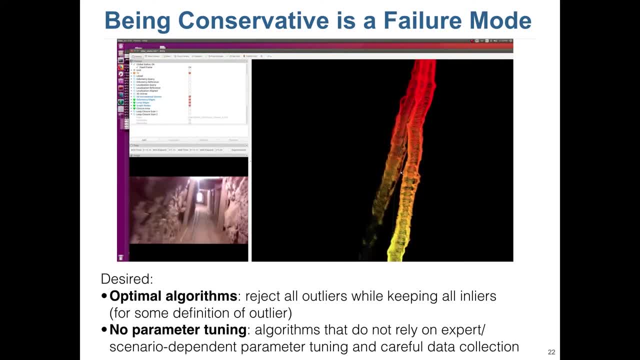 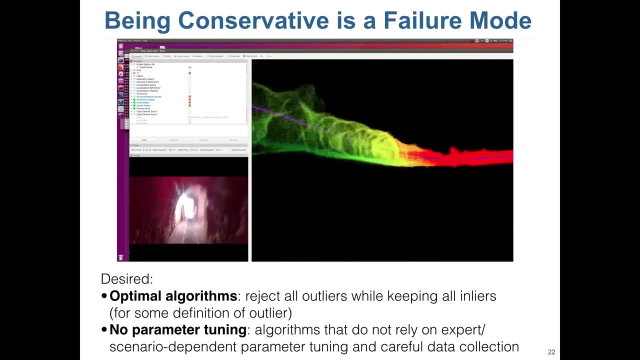 But all our tests are seeing are just rejecting that as an outlier And this, again, is a failure mode. So what we want is really two things: We want optimal algorithms And optimal means. algorithms are able to reject all outliers while keeping only layers for some definition outliers, as I 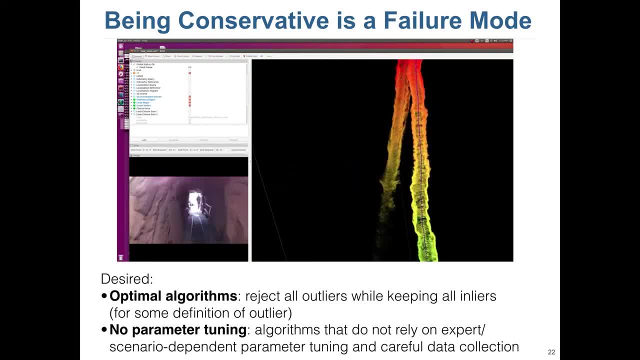 would say We'll give shortly. And the second is really we don't want parameter tuning, We just want an algorithm that does not rely on expert parameter tuning or careful data collection. So what we did really any questions so far? 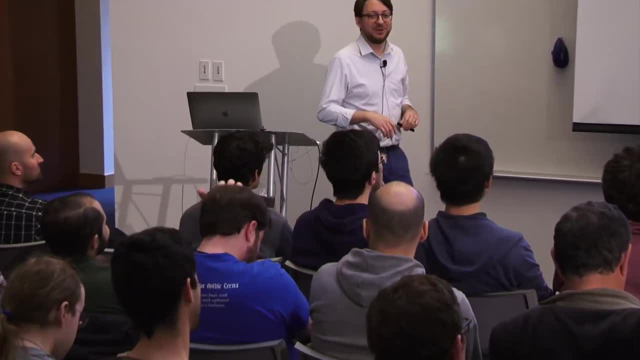 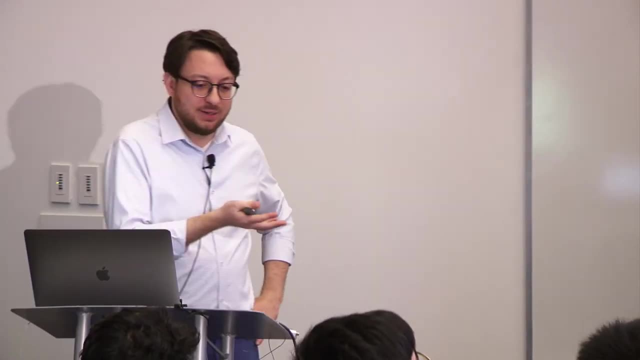 I know that was kind of a long introduction and motivation, but we'll get to the point. So what we did, seems is an interesting problem, Like a lot of practical application, and there is no good solution, in my opinion, out there. 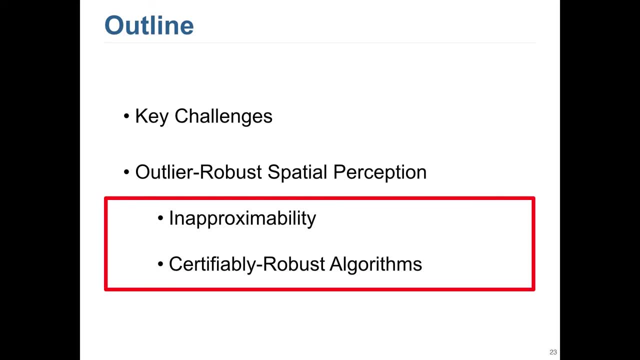 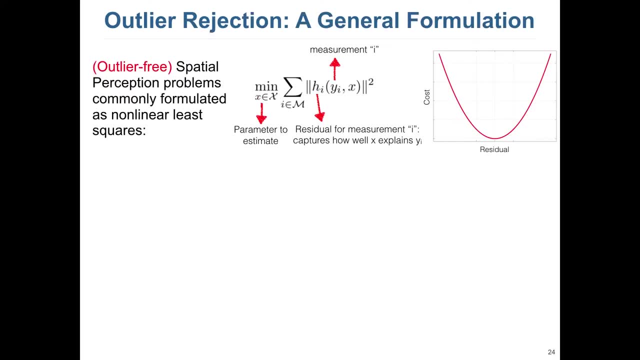 So we tried to approach the problem And I believe the good, reasonable starting point is to say: can we even hope to formulate and solve this problem? So what we did, as Luca was suggesting, is to look for, first of all, to start with a general formulation. 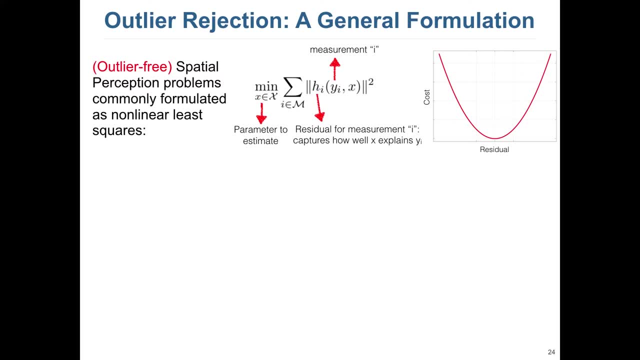 of the problem. In the outlier-free case there is a general formulation. So spatial perception problem in the outlier-free case are commonly formulated as nonlinear least square problems And in this kind, in the absence of outlier, essentially this nonlinear least square again. 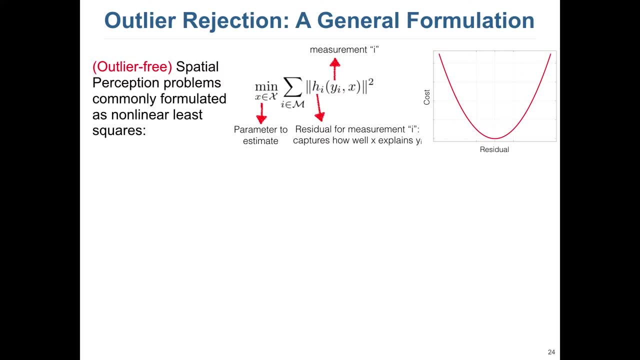 you want to compute some state x belonging to some domain, And you want to do that by minimizing a sum of squares of the given measurements, where the yi are the measurements, yi is the height measurement And hi is the residual error. You can think about the residual error. 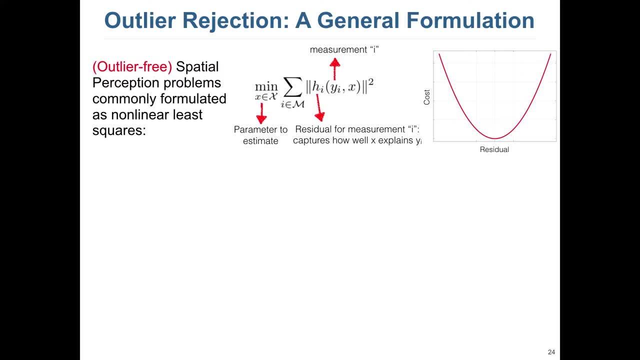 as capturing how well the x is explaining the y. I also said that this formulation typically doesn't work, And I want to give you a very intuitive reason why this doesn't work. So you can see here that there are squares right. 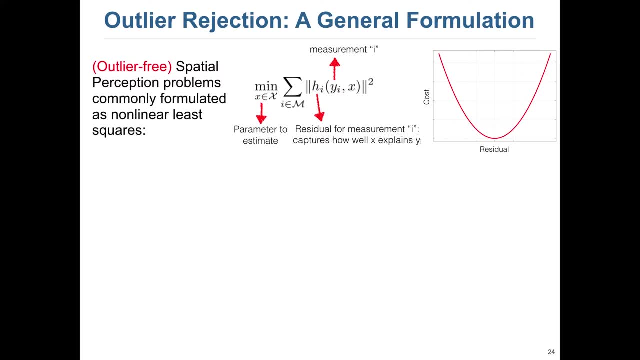 So there is a quadratic dependence between the residual and the cost. So you take the residual, you square it and you put it into the cost. What happens there is that outliers, pretty much by definition, are measurements with large residual And the cost is quadratic in this residual. 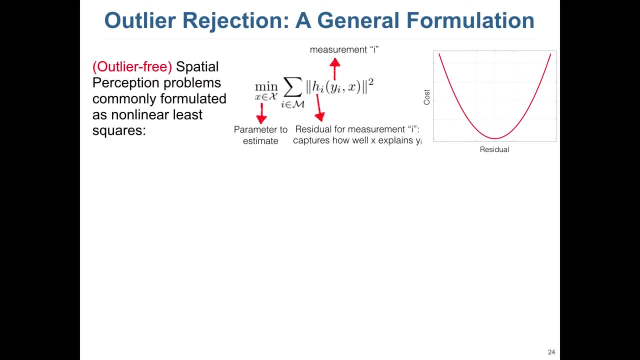 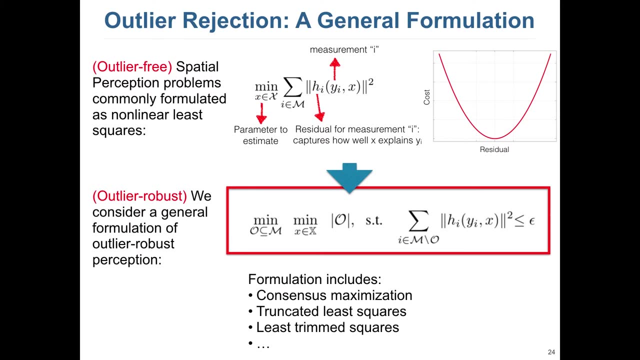 So outlier end up dominating the cost. That's why it doesn't work this kind of estimation problem with outliers. Our formulation looks like that We said let's consider a general formulation for outlier rejection. And this is how it looks like. 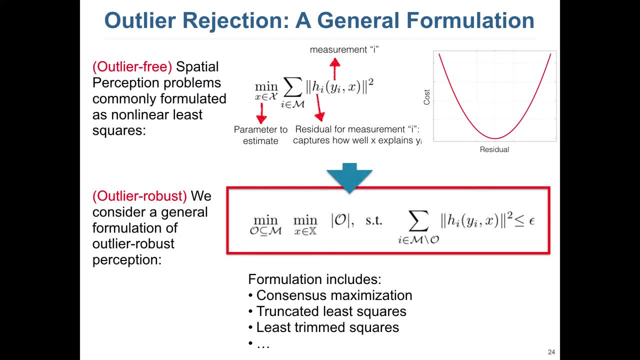 So here, not only you minimize with respect to the state that you want to compute, but you also minimize to find the set of outliers, so the subset of measurements being outliers. And you do that in order to minimize the number of outliers. You want to pick the least amount. 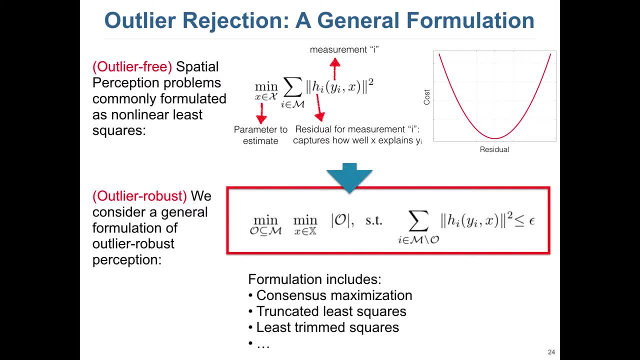 of outliers to avoid rejecting good measurements. But the condition is that whatever measurement that you consider in liar, so the set of measurement minus the outliers, whatever measurement you consider in liar, should have small error. So in other words, again we try to find the smallest. 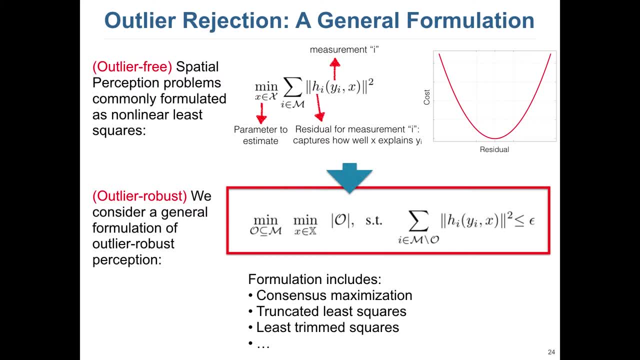 set of outliers, such that the remaining set of measurements can be well explained by a state x. Why would that be? Well, it's because the set of outliers, the set of measurements, can be well explained by a state x. So why did this? 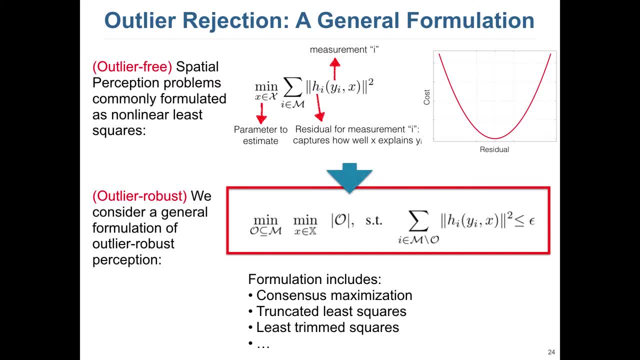 Well, I believe the real reason is that this formulation is quite general and it's including a number of standard formulation in the literature, including consensus maximization, which is very popular in computer vision, truncated least square, which we'll see in the rest of the talk. 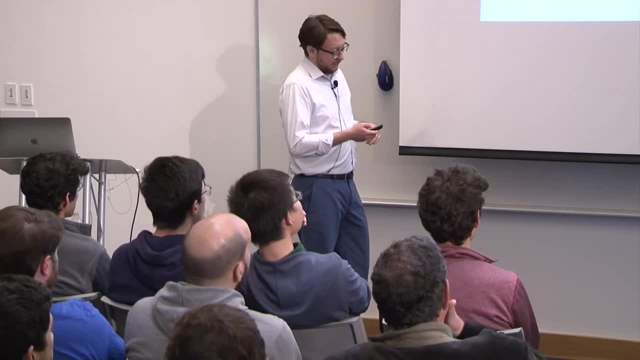 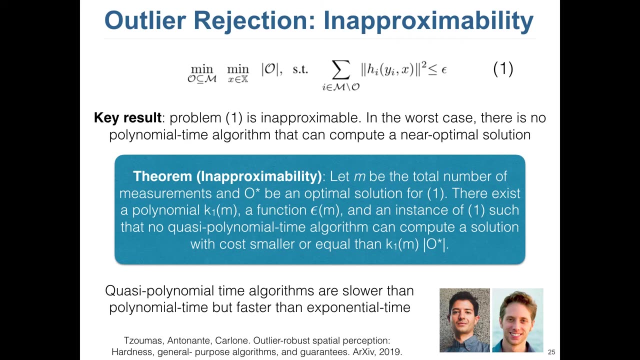 and other formulations. Now it gets to the bad news. Well, the bad news is that we tried to analyze this optimization problem. We tried to find if it is even possible to solve this optimization problem And we incurred inapproximability results. 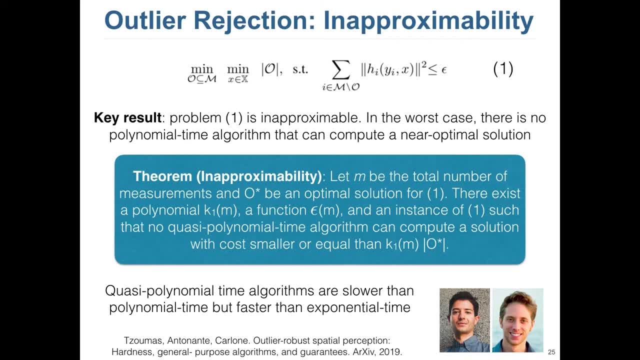 So the key result says informally that problem one is not approximable. In the worst case there is no polynomial time algorithm that can compute a near-optimal solution to it. The more formal statement says something a bit deeper, I guess. 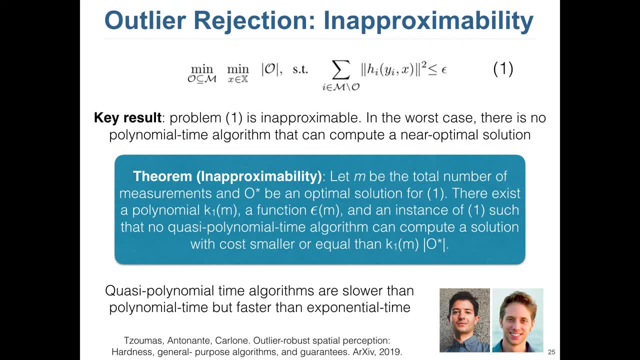 If m is the total number of measurements and o star is the optimal selection of the outliers, then there exists a polynomial function, k, a function k, k, k, a function- epsilon, and an instance of this problem such that no quasi-polynomial time algorithm can compute. 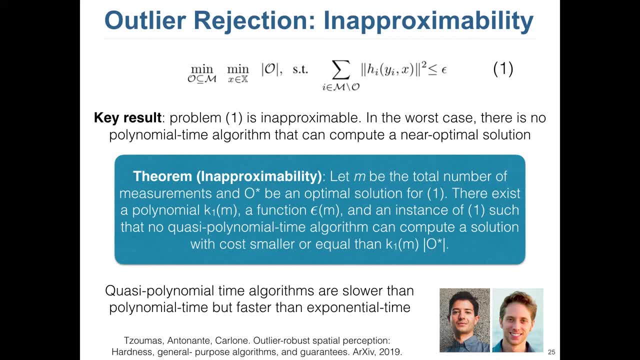 a solution which costs smaller or equal than k1 times the optimal. So o star is the optimal solution And any quasi-polynomial time algorithm cannot even get close to o star. It's k1 times away from o star. And for those of you who don't know quasi-polynomial time, 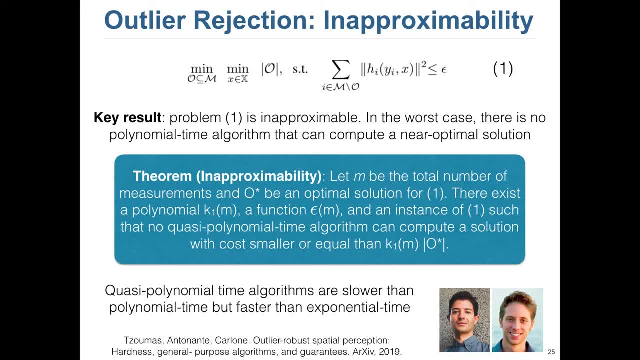 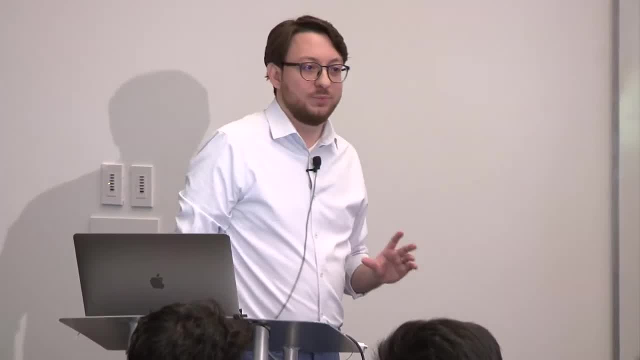 algorithm are essentially the same thing. It's essentially slightly slower than polynomial time, but faster than exponential. So this is saying, in the worst case we do not have any hope to really solve this problem even close to optimality. And here close to optimality means a very precise thing. 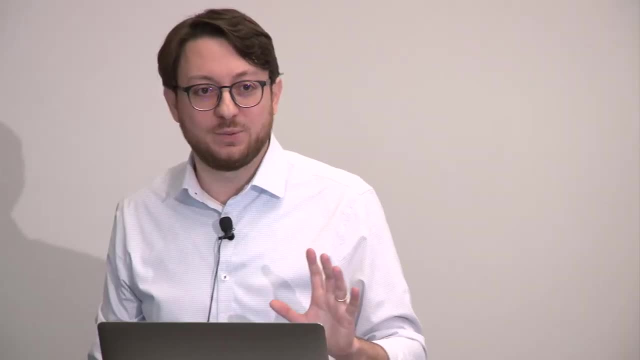 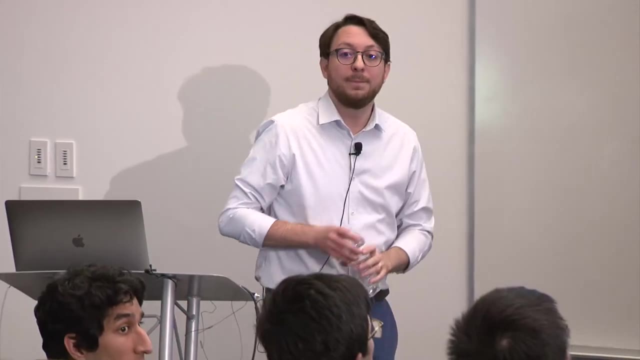 We cannot hope to find the outliers and reject few inliers. That's what it means. Questions Is sort of the right problem to be solving, Like where does epsilon come from? And let's say you've just chosen the optimal set of outliers. 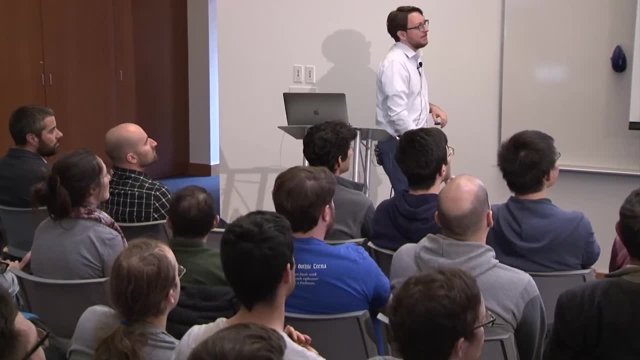 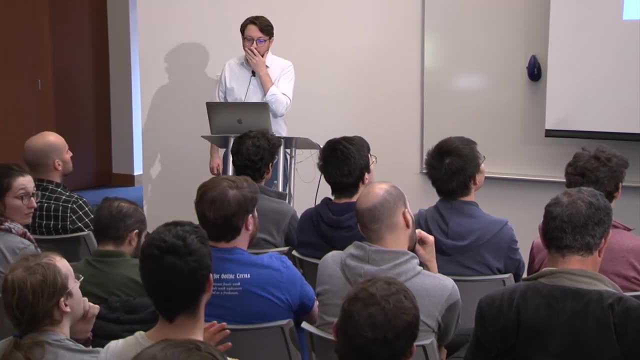 Aren't there a variety of x's that are solutions to this? Because you're sort of not directly penalizing, but you're just constraining that to be less than some value of the hx squared. You have that in the objective as well. 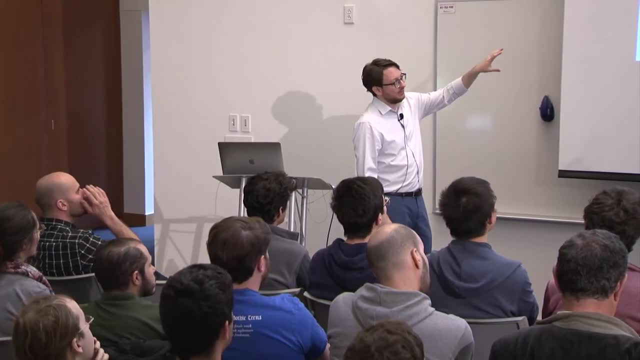 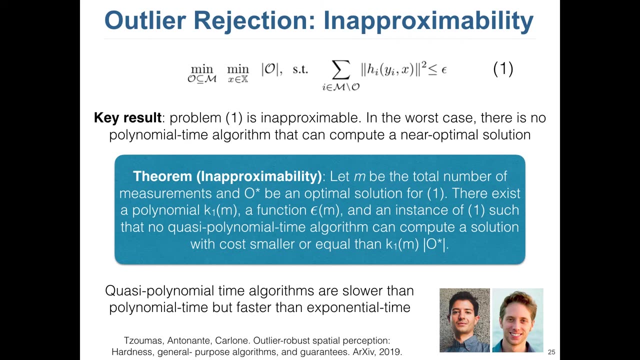 Yeah, So variation of these will also following. the same reason can also be shown to be an approximate. For example, something that we'll do next, which is reasonable to do, is that you say that, rather than the sum of the square is. 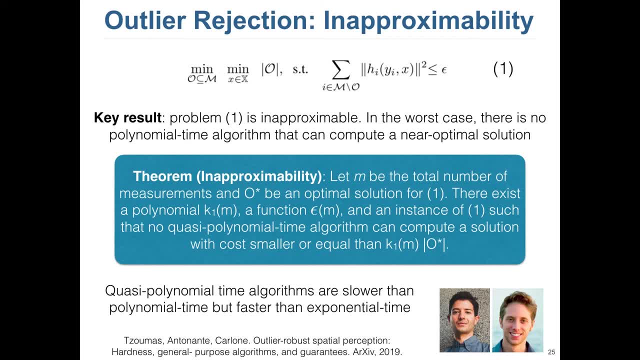 smaller than epsilon. you can say that each measurement should have a residual smaller than epsilon, which means you define what is an inlier, saying that an inlier is a measurement with the maximum residual epsilon that you decide. So a translation error, the maximum I can tolerate. 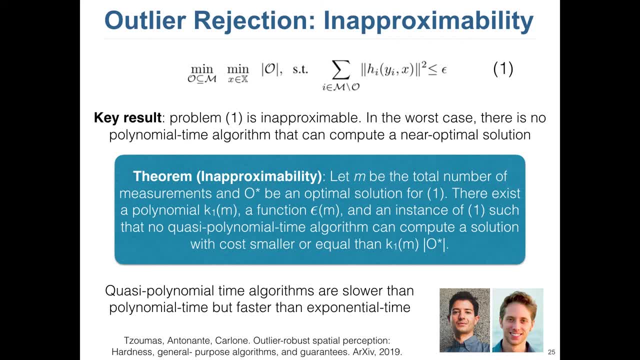 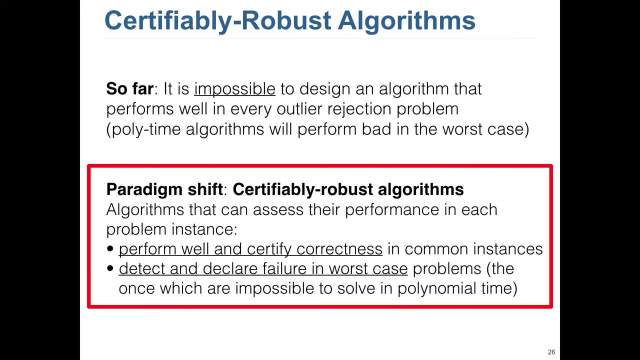 is like 10 centimeter. You can say that 10 centimeter is a bound, You can follow the same reason and you will still get an approximability. So so far pretty bad news. It is impossible to design an algorithm that in every East. 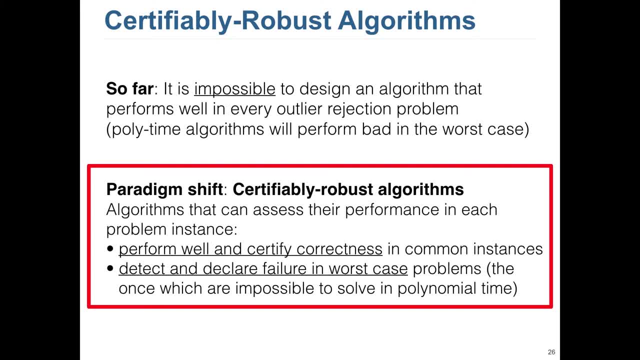 and South layer rejection will work well, because polynomial time algorithms will work badly in the worst case. So we can just keep up and say, OK, we cannot solve this problem, Let's do something else. What we propose is really like a change in perspective here. 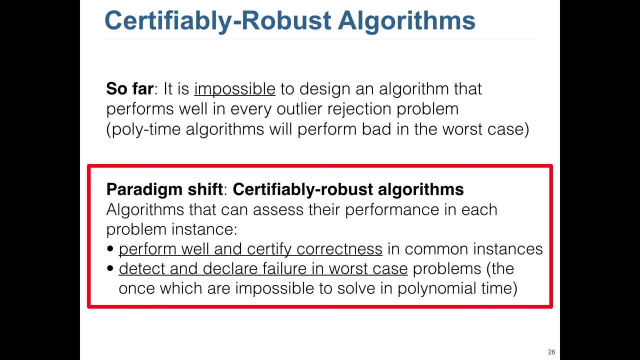 We propose this idea of certifiably robust algorithms, which I believe is a very interesting concept. Essentially, since you cannot solve every problem instance, we just want algorithms that can assess their performance in each problem instance. OK, OK, OK. In other words, we want an algorithm that works well. 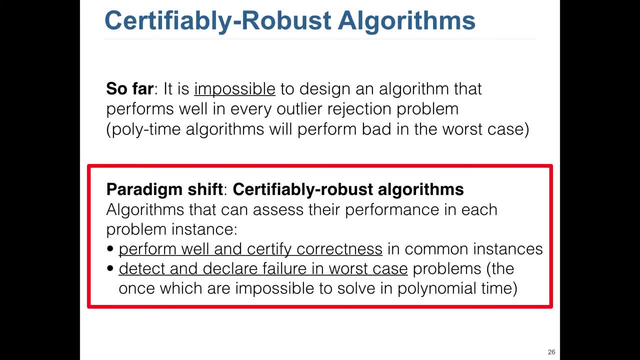 and certify that it is working well in common problems, one that you encounter every day when you operate your robot. But at the same time, the algorithm should be able to detect and declare failure in worst case problems. Should not just fail silently, Should say I'm not able to solve it. 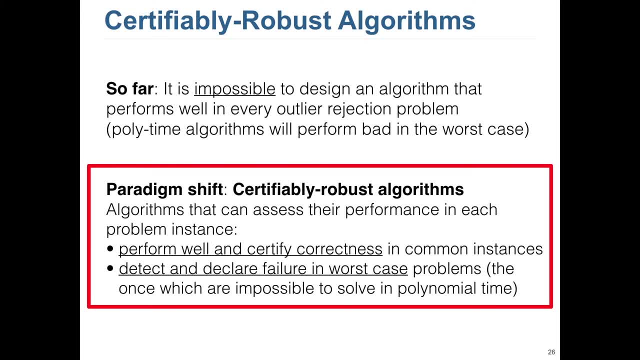 And anyway, that's pretty much the best you can do, because in the worst case it's impossible to get a polynomial time algorithm And of course one requires the very here I'm putting is kind of implicit. The algorithm should be polynomial time, right. 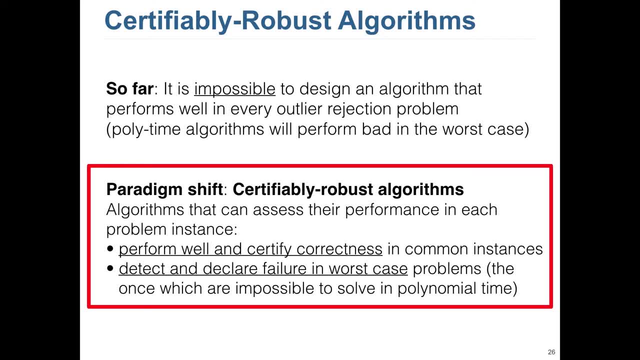 We are doing this to get efficient solution Seems to be quite interesting concept, but it's unclear if this is even possible to do. Is it possible to design these certifiably robust algorithms? Well, the fact that that's the item in the next part of my talk probably the answer is yes. 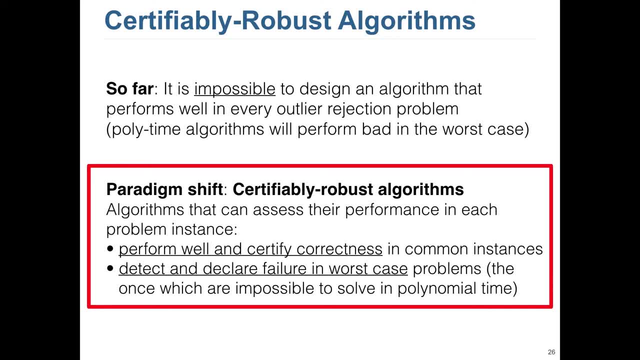 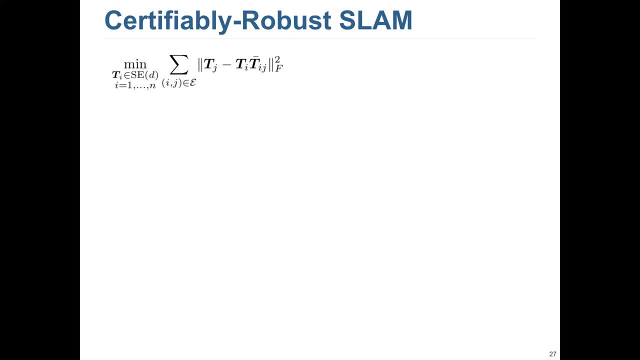 We can design certifiably robust algorithms, And in the following we'll provide two example. First one is about certifiably robust SLAM And the second one is about certifiably robust registration. Okay, I will show that it is possible. 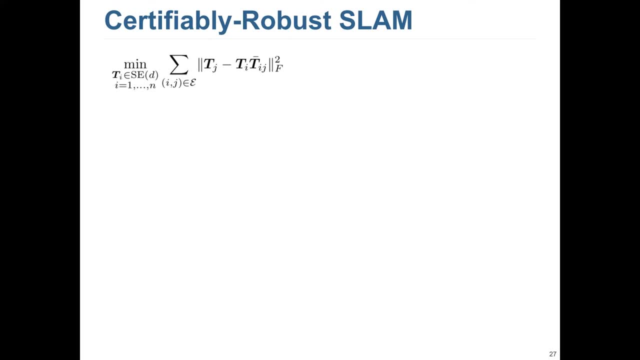 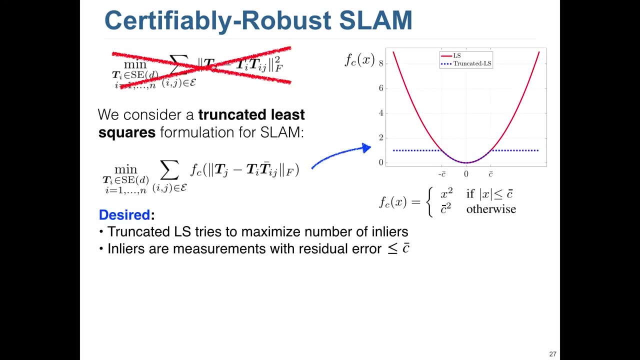 Certifiably robust SLAM. we started with the nonlinear least square function and we said that this is not going to do it. So we consider a variation of the formulation that I showed a few slides ago. So we consider a truncated least square formulation for SLAM. 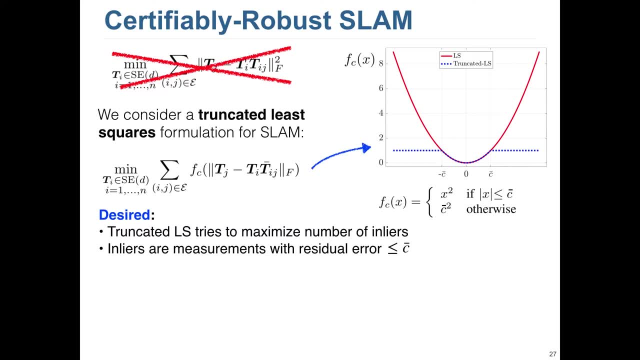 Truncated least square. you can see that this is pretty close to the formulation that we propose, but instead of having like a square of the residual error, you put the residual error as argument of a function where the function is a truncated quadratic cost. 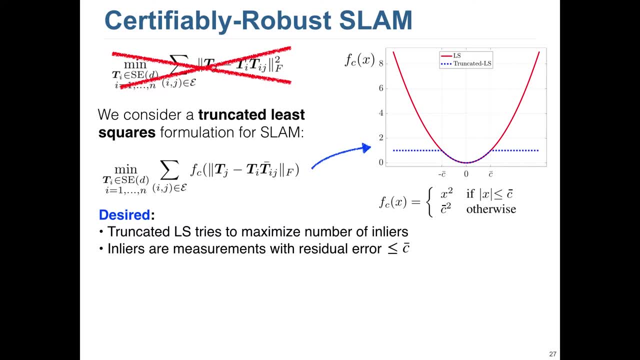 Rather than being quadratic all the way, it is just constant outside the bound. So the function again, FC, is quadratic if the argument is within some bound C and is constant otherwise. So why does does this make sense? Well, it has two desirable properties. 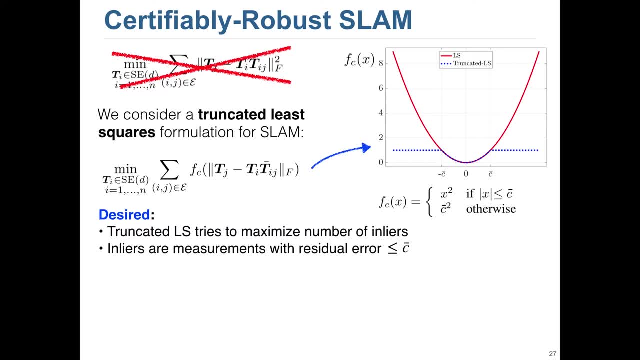 First of all, the truncated least square tries to maximize the number of inliers. Why is that? Well, you can see that the inliers are the one falling in the quadratic region and the cost is smaller in the quadratic region than in the constant region. 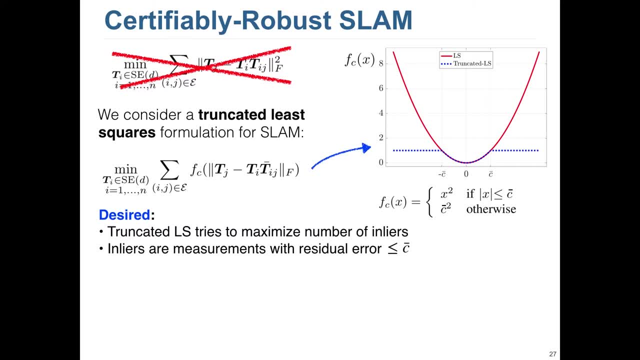 So the cost will essentially enforce that you pick as many inliers as possible And, by construction, the one that fall in the quadratic region have residual error which is smaller than C bar the maximum error saved. So only one of those things: the maximum error that you want to tolerate. 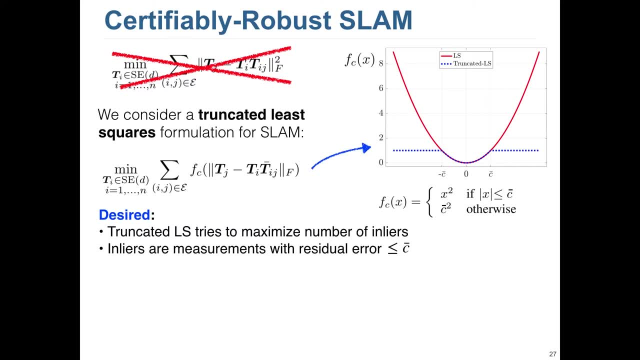 on some inlier. Okay, so it says these two desirable properties. I know that this is essentially a way to get rid of the fact that outliers with larger residual error are dominating the costs. Now, instead, outliers with larger residual error are just having a constant impact on the cost. 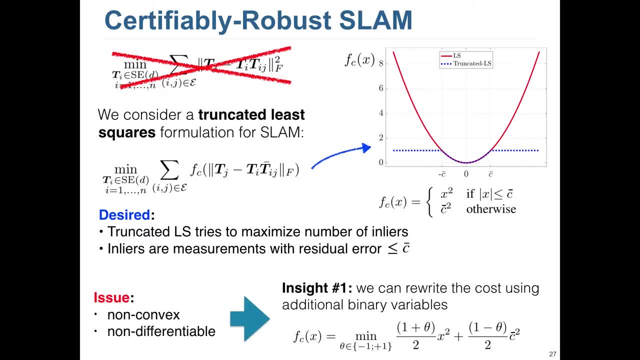 So it really address this issue, like the presence of outliers. So now I'm telling you that this is a reasonable formulation to try to solve, to get robotization and hope to help do that to solve, to get robustness to outliers. Unfortunately, this formulation is not the nicest one. 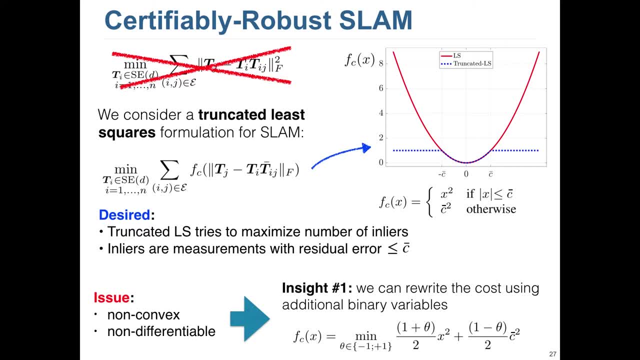 because the function fc that I'm showing here, this quadratic, truncated quadratic term- for those of you who are familiar with optimization- you realize that it is a non-convex, clear non-convex function and it is not differentiable. 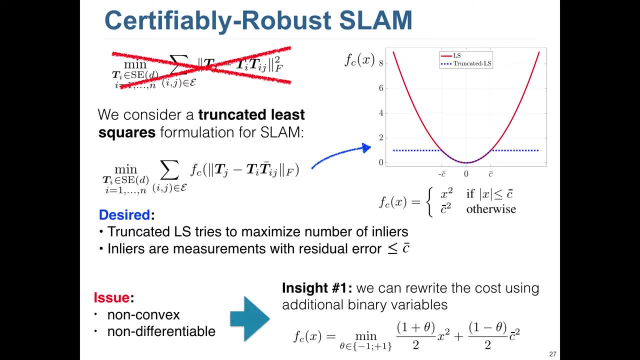 That can be or cannot be a problem. So, essentially what I'm going to do in the next few slides, I will show you that actually it is possible to get global solution to this optimization problem, even though the formulation to start with looks ugly. 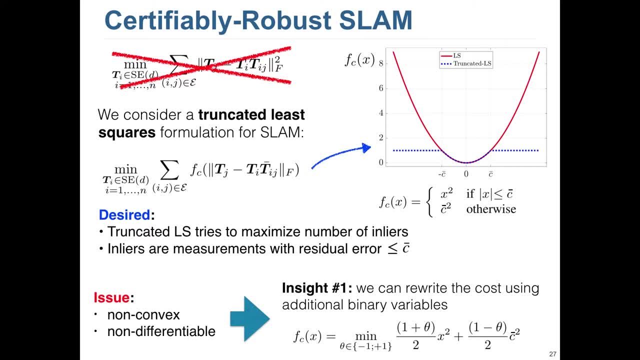 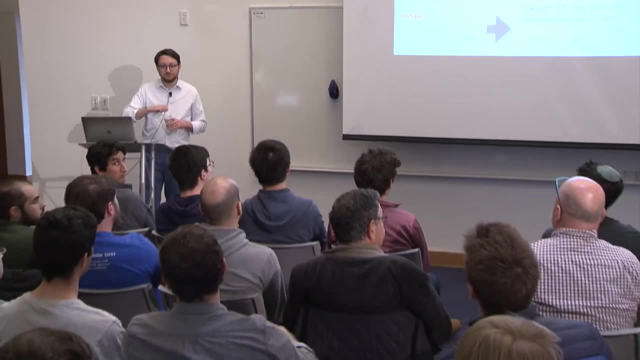 looks very difficult to solve, So we don't hope to solve the worst case of this. yeah, Not only is it non-convex, but if your initial guess is far enough off, then it's degrading. but everywhere would be zero. 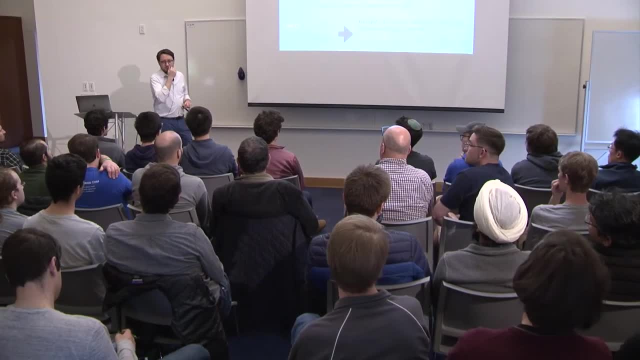 Surprising that this appears as a problem. I will show you that we will get a convex relaxation if you slide of that and does not even show up as a problem. I'm very surprised, but I agree. So that should show up. 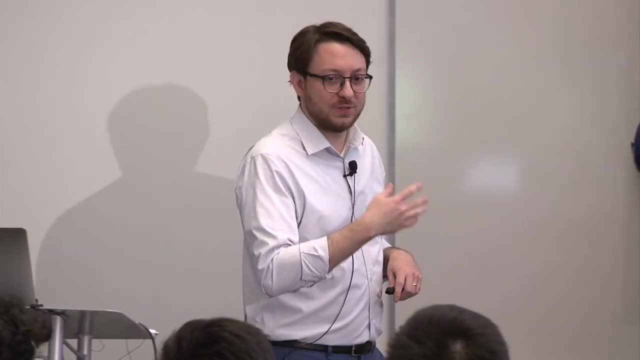 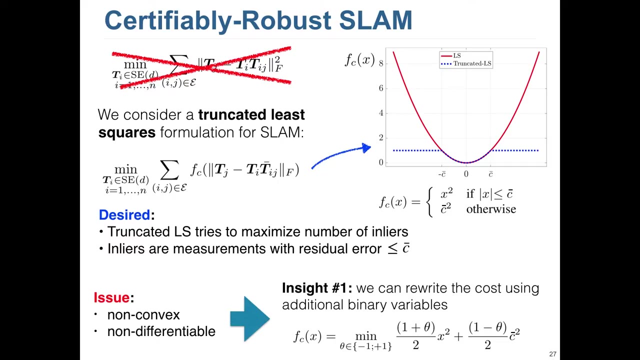 the fact that you have flat gradient, but it's not really a problem. You can just solve it, and I will show you how. The first insight is something that you can do in high school. I think it's a very simple one. 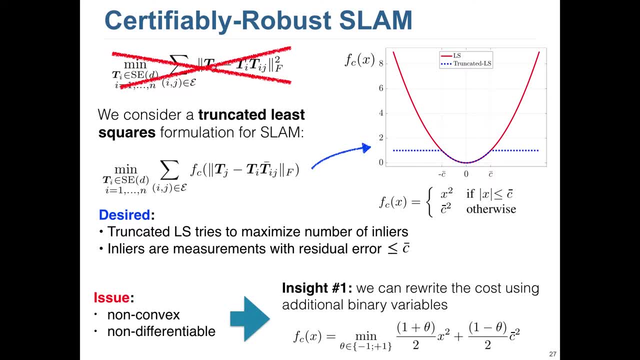 You can just rewrite this cost function, which I wrote as a quadratic in some region and a constant otherwise, by introducing additionally binary variables. So I'm just rewriting the same function there with binary variables. So you can imagine that the theta as a binary variable. 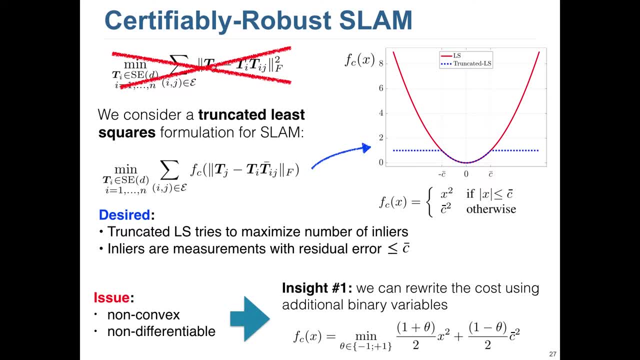 can be either minus or plus one. If the theta is plus one you get the quadratic behavior and this guy disappears And essentially you are inside the quadratic region. If you said the theta is minus one, the first time disappears. can you get a constant? 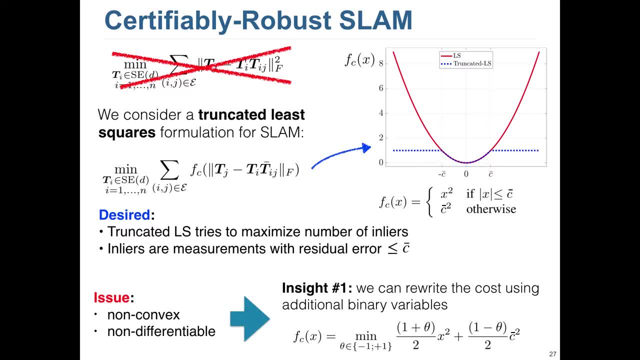 so you are in the constant region outside, In other words, is the theta is deciding. theta plus one is saying this is an outlier. Theta minus one is saying this is an outlier should be like out of the constant region. constant. that is the only threshold that you have here. 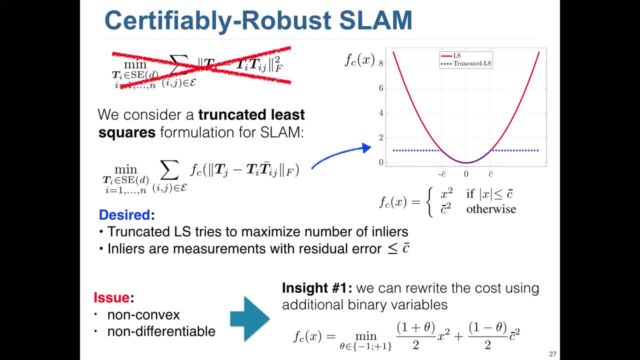 is the maximum error that you can tolerate to call a measurement in liar. Okay, so that's the first step. So we started with a weird problem. We made it a little bit more complicated by also including binary variables, So let's try to see how this problem looks like. 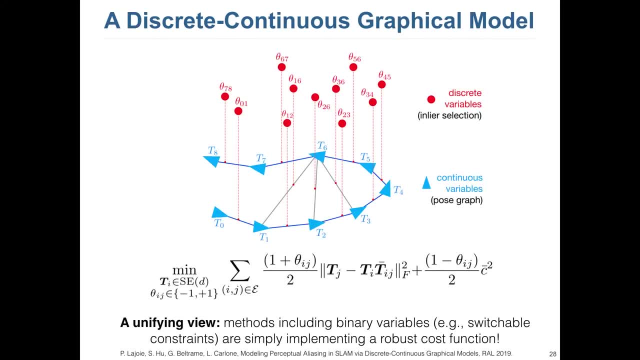 if you use this expression of the cost function And that's shown like in this optimization problem. Despite the complexity of the optimization problem, it's pretty easy to understand. Again, like you know, if theta ej is plus one, you keep the quadratic term. 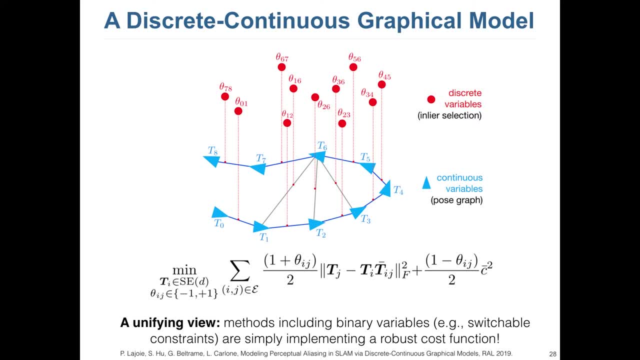 otherwise you delete it and you set it constant And you can visualize this graphically as a discrete, continuous graphical model. So in the previous slide I was showing you the graph of poses that we are doing estimation over, And what I'm saying is that now we augment this estimation. 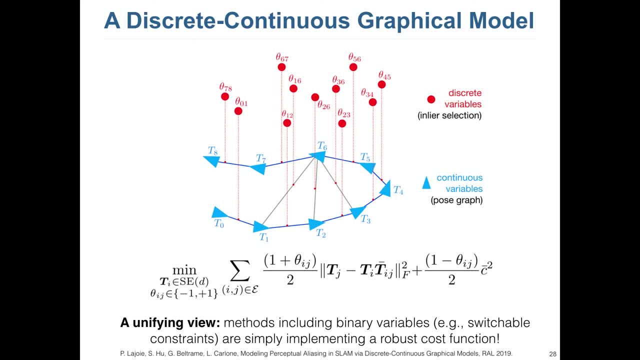 this graphical model with a binary variable associated to each age, And this binary variable will decide whether that measurement is in a liar or outlier. This is what we call the discrete continuous graphical model. For those of you very familiar with SLAM, you will say: well, but that's. 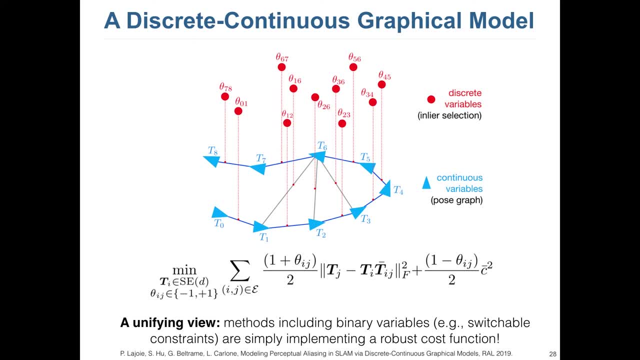 this idea is, like you know, switchable constraints- very close to other formulation And indeed it is, Like you know, the basic idea of including binary constraint to switch off variable is very common. What we did so far, first of all, 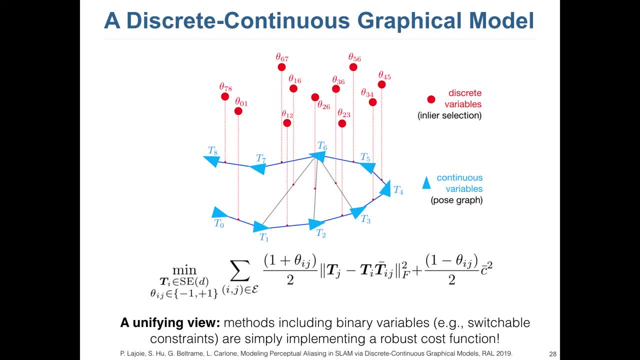 is to get to a slightly different expression, in particular for the second term, which will help us, But also, essentially, we are providing a unified view. So we are seeing that, while switchable constraint, the paper was calling this some probabilistic prior on the activation of the constraint. 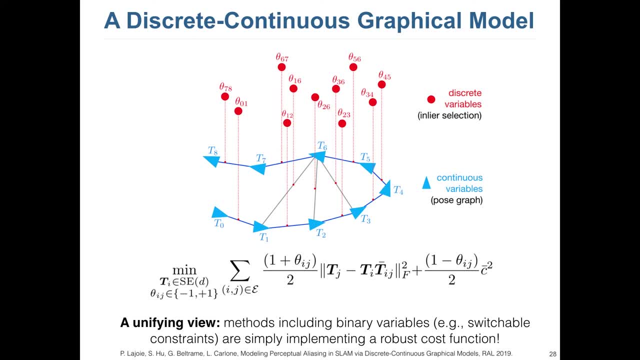 we are demonstrating this is only writing- a robust cost function. So now the C has a clear physical meaning. It's maximum error that you want to tolerate on the liars. So that's cool, but it's not like fully satisfactory. Ideally, we really want to solve this optimization problem. 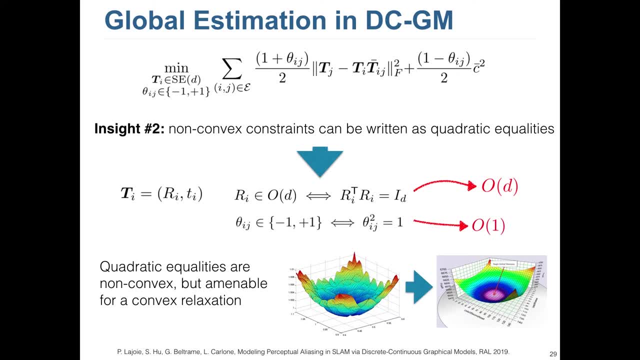 which is what we try to do next. So next, I want to show you how to get the global optimal solution, globally optimal solution, to this optimization problem. The insight tool that you have here is that all the constraints in this optimization problem can be written as quadratic equality constraints. 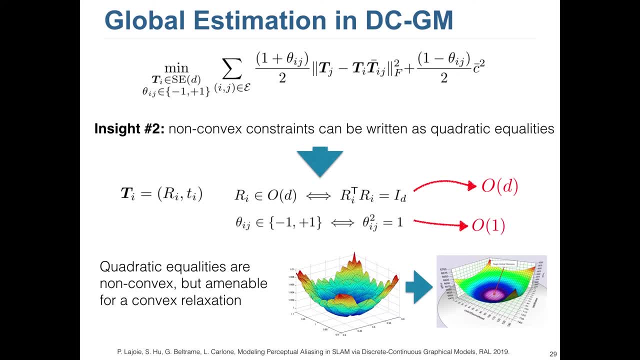 The constraints are a bit hidden here because they are really like hidden over here. The first constraint is that ti are poses, So they are a member of sci2 or 3, depending if you're on a planar setup or 3D setup. 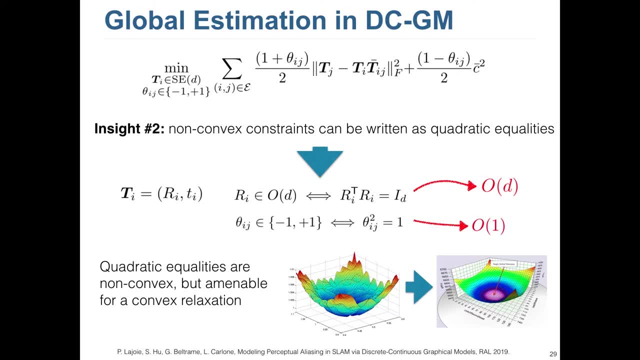 And I'm arguing this is true. that can be written as a quadratic equality constraint And indeed, if you have a pose, a pose is just a rotation and a translation. A translation is a vector which is unconstrained, so we do not have to worry about it. 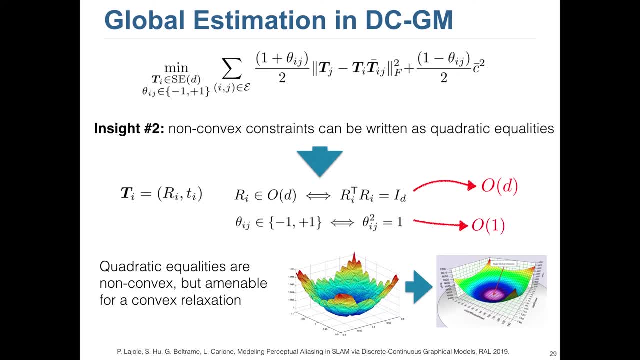 And a rotation is some orthogonal matrix, in the sense that rotation by definition should be orthogonal, which is R, transpose R, equal to the identity matrix of the right dimension And for those of you who are a bit more expert about this, I'm dropping the determinant constraint for simplicity. 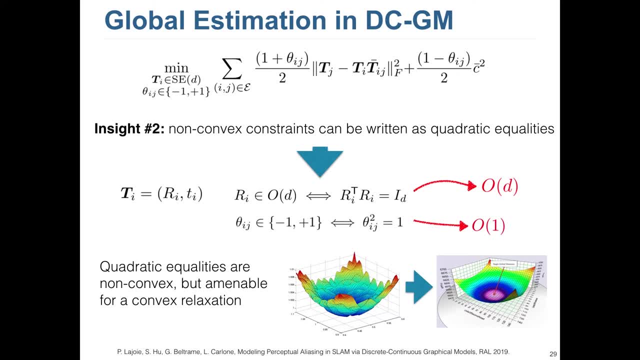 Okay so, because a rotation should also have some determinant equal to plus one. The second constraint that we have is this fact that the theta Ej should be either minus one or plus one, and it's pretty easy to realize that forcing the theta Ej to be binary is the same as forcing theta Ej squared. 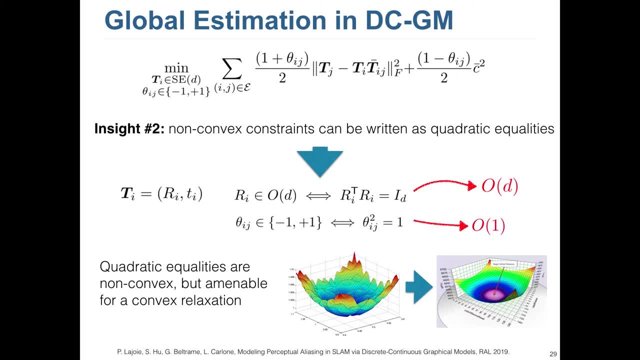 to be one. The only solution to that equation is like minus one or plus one. So I'm seeing that all this constraint can be written as quadratic equalities, and the good thing here is that all this constraint can be written as quadratic equalities, and the good thing here. 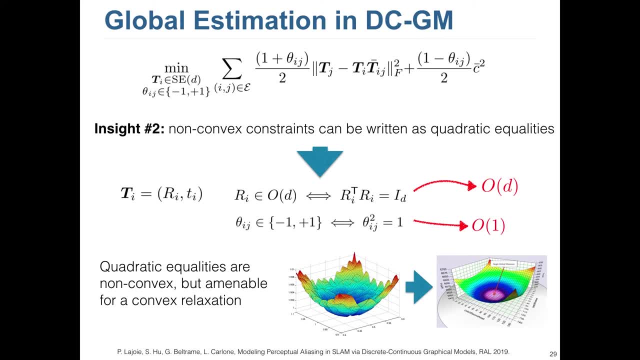 is that all this constraint can be written as quadratic equalities, and the good thing here is that all this constraint can be written as quadratic equalities. So, although quadratic equalities are still non-convex, they are amenable. they are good to do. 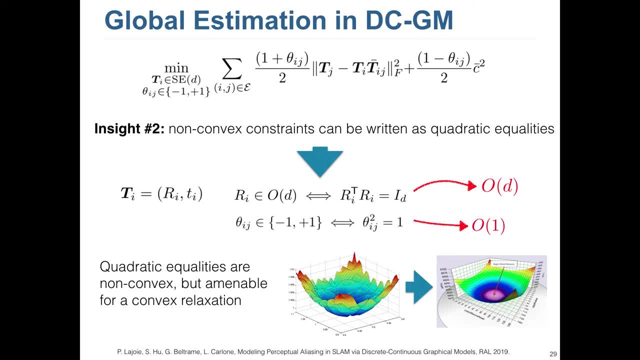 like a convex relaxation. So what you are going to do next is to move from these non-convex- the starting problem, which is non-convex and very difficult to optimize globally- to something that is a convex relaxation for which you can get to the optimal solution in polynomial time. 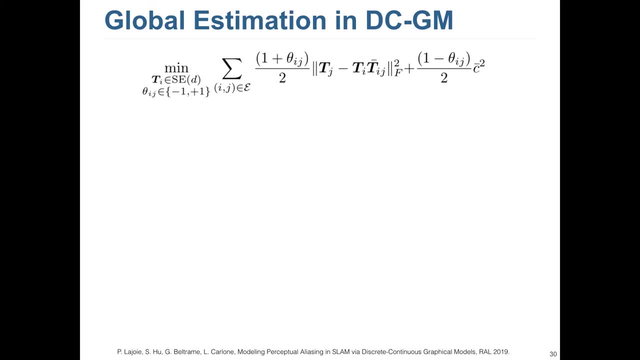 How do we do that? Well, this is next three slides. probably If you're not familiar with the optimization you want to cover your. So that's, like you know, the denser part, but I would like to show you that you know. 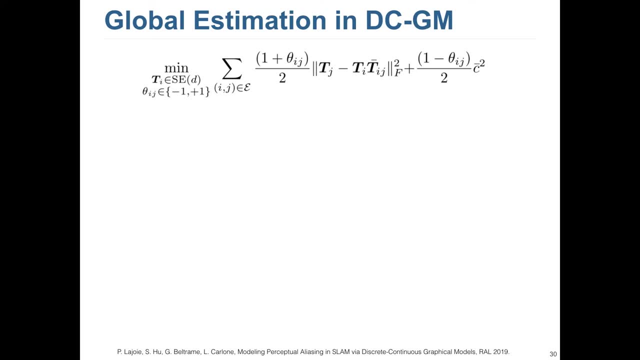 the math of getting the convex relaxation is actually is a lot of algebra. it's pretty simple. So you start with this optimization problem. The first thing that you do is you try to reparameterize the optimization problem in terms of a variable X. 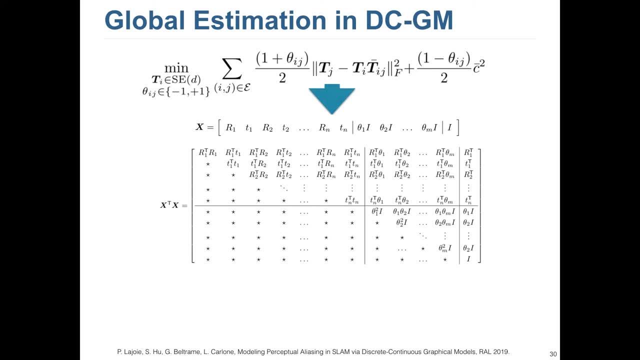 where X is only stacking all the unknowns, rotation translation for all the poses and the thetas. Okay, we're just stacking all in a single large matrix. Then the second observation is that if this is X which is stacking all the variables, 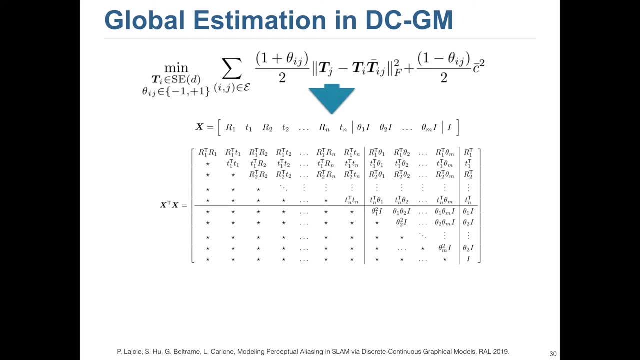 X transpose X is just. if you do, the matrix product will be just containing all the product within pairs of variables. That's the way like the product works. And finally, the observation is that you can rewrite every part of this optimization problem as a function of X transpose X. 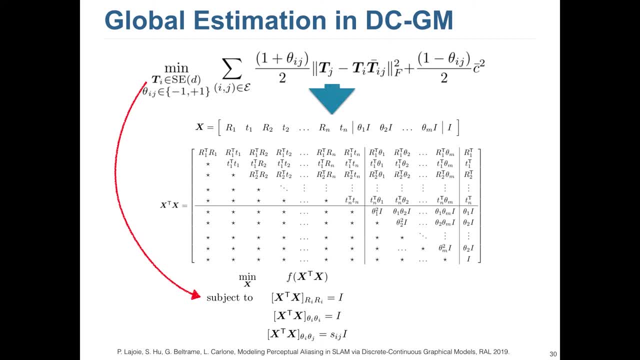 So you can write this optimization problem by using some entries of these: X transpose X. The objective in particular will be a quadratic function of X transpose X. I will not do the demonstration for that because it's a little bit algebraic, but I would like to show you. is that the fact that 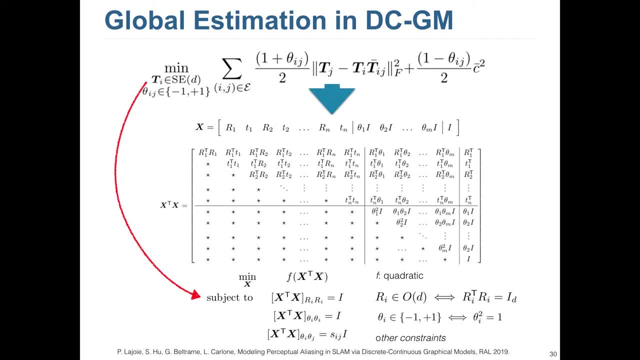 for example, rotation should be orthogonal, just means that we should pick, for example, the diagonal blocks of these X, transpose X and force them to be the identity. Similarly forcing that the thetas should be like thetas square should be equal to plus one. 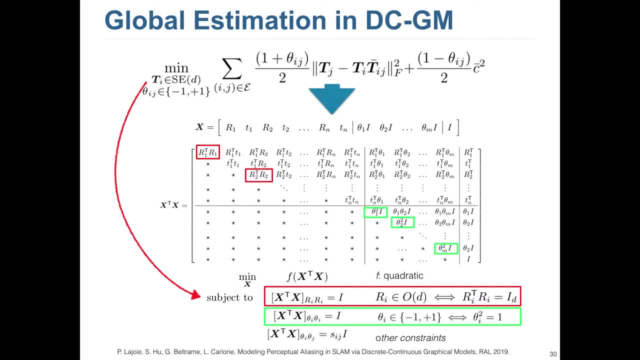 just means that you have to pick these diagonal entries of X transpose X and force that to be the identity. And we can also force extra constraint, which are all function of these matrix magic matrix: X transpose X. So what I'm arguing is that this problem 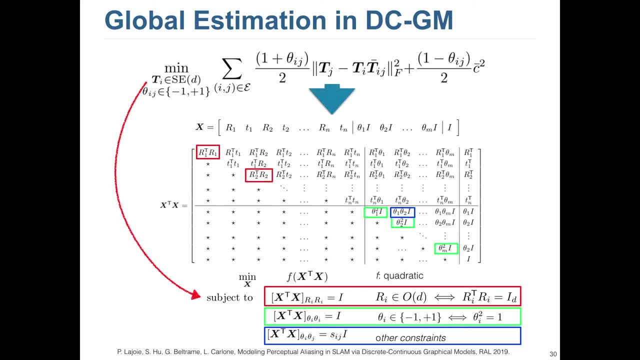 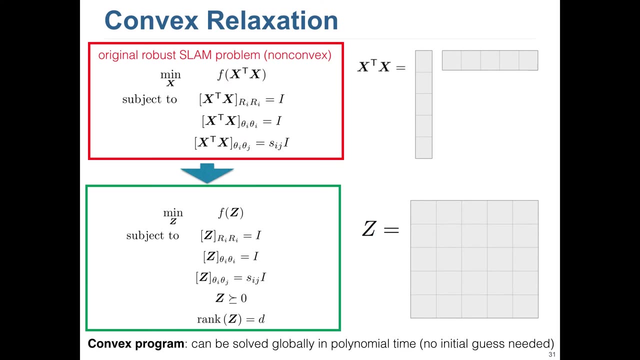 can be formulated exactly, except for the determinant constraint that I'm dropping, exactly as this problem, where the F is a convex quadratic function and the other constraints are quadratic equality constraints. Now this formulation, because of the quadratic equality constraints, is still non-convex. 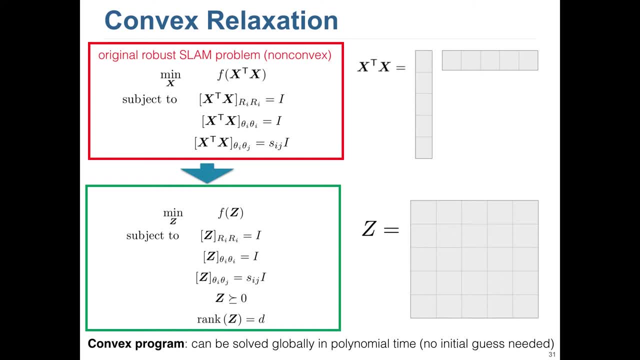 Quadratic equality constraints are non-convex And the trick is pretty much always the same: to get the convex relaxation, You take X, transpose X and you replace it with a full matrix Z. So rather than X transpose X, you use a single matrix Z. 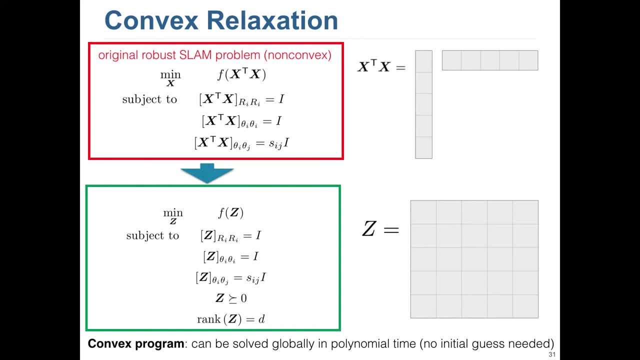 and you replace every X transpose X with a Z. Okay, For the matrix Z to be equal to X transpose X, Z should be positive semi-definite. It should have rank D, which is the number of columns here in the number of rows here. 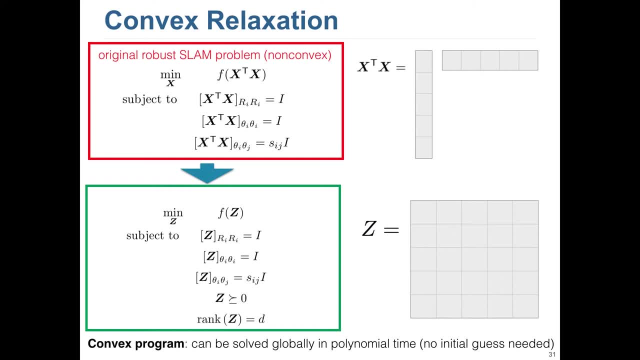 Okay, So I'm rewriting: instead of X, transpose X. the same problem as a function on Z. And now I'm realizing that this problem has a quadratic objective. linear constraints- which are good, they're convex- semi-definite constraint, which is convex as well. 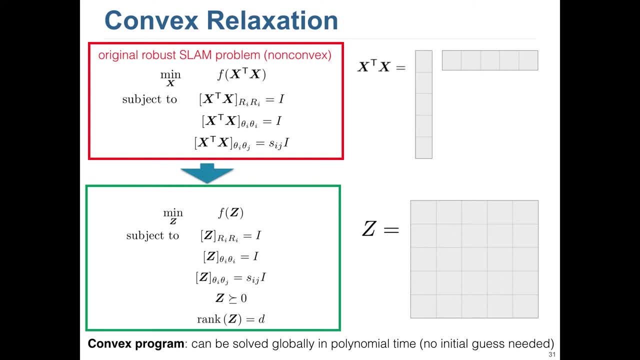 And the only non-convex is the fact that I want to enforce the rank of these matrix to be D. So in order to get the convex relaxation, I just drop the rank constraint and I get the convex relaxation. So we started with a difficult problem. 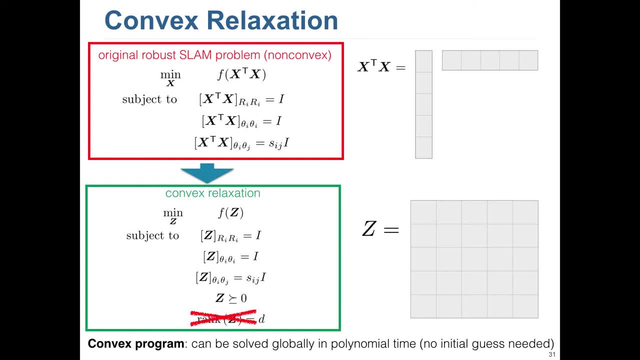 to solve combinatorial, non-convex and so on. We ended up with a convex relaxation which has the nice feature of being solvable in polynomial time and without need of any initial guess for the trajectory. Another question is: is the solution? 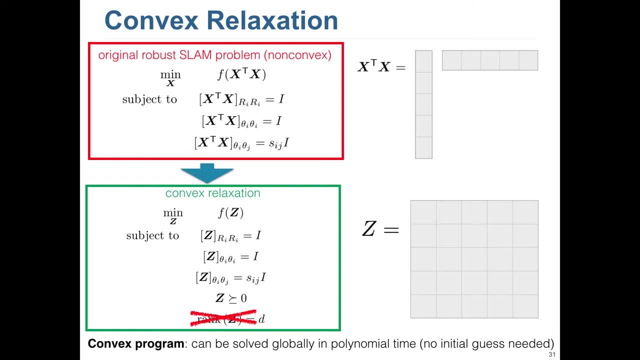 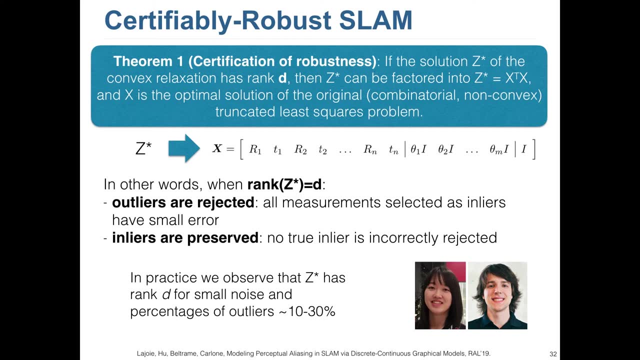 of this convex relaxation going to be a reasonable solution for the original problem. A few results about that. I think there is more work to be done on this, but the basic result is about certification of robustness. So it's easy to get results like: 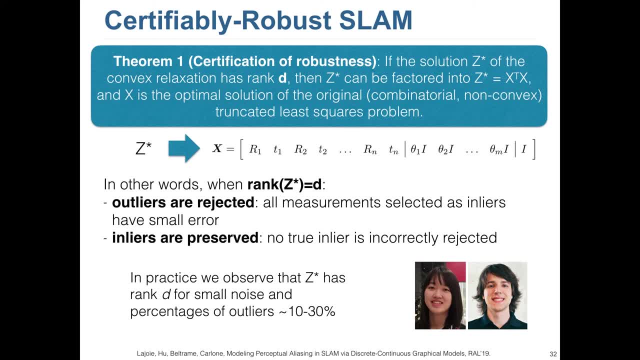 if the solution Z star of the convex relaxation has rank D, where D again is the dimension of the problem, two or three, then Z star can be factored into X, transpose X, and X is the optimal solution of the original combinatorial, non-convex truncated relaxation. 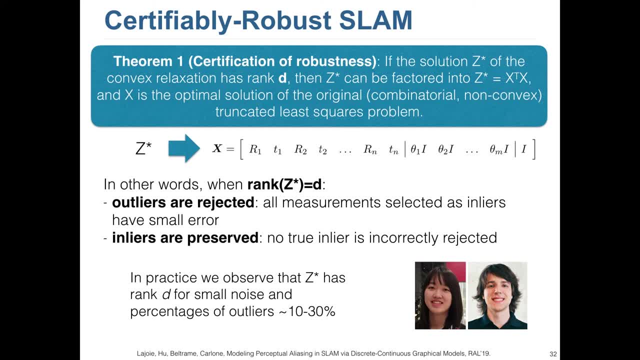 So that's the answer to the D-square problem. In other words, you take Z, transpose Z star. you can just extract all the poses and all the decision about the layer and outlier. Put it in practice. this means that when the rank of Z 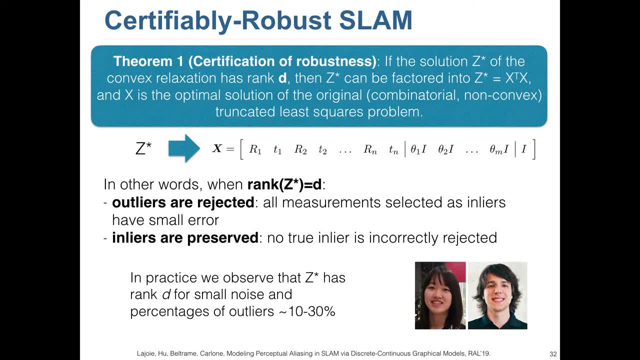 is exactly D, all the outliers are rejected and all the measurements selected as the layers will have small error and also you can guarantee that the layers are preserved, just because we said that the cost of having a layer is smaller than the cost of having an outlier. 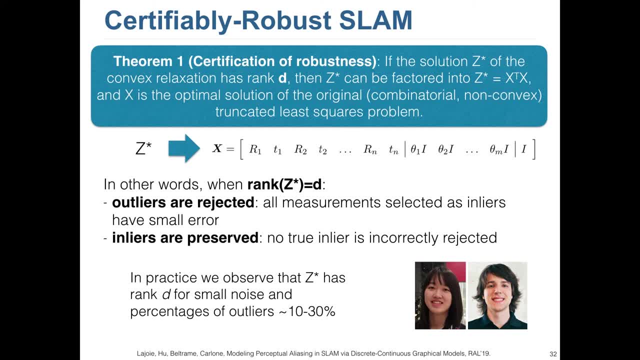 So this is work done by C and Pierre-Yves in my group, and the nice thing is that in practice, we observed that in a domain which is not huge this time, but in a domain in which the measurement- noise- and the number of outliers is not huge. 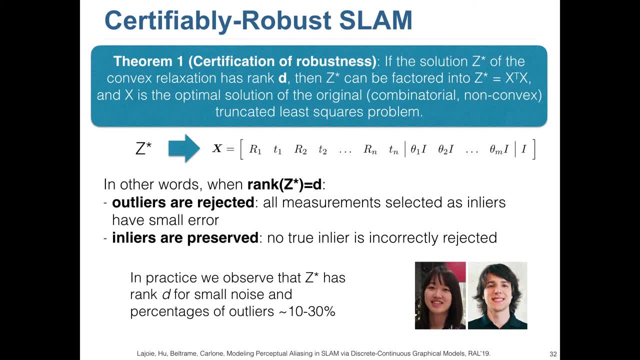 Z. star has more rank, has rank D. So that's similar to the notion that I was telling you about certifiably robust algorithms. There is a setup, there is a common problem, instances in which the percentage of outliers is not huge, in which you can solve the problem. 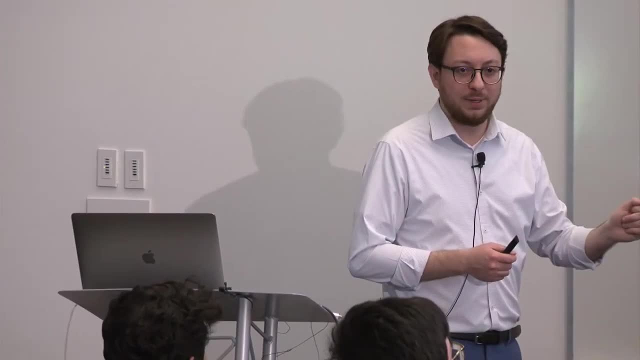 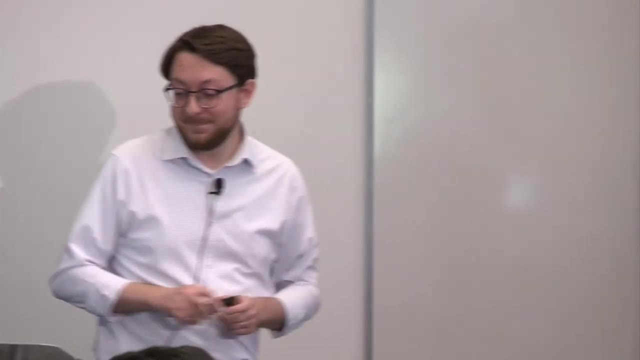 and you can certify that you got that. you got the best solution for that, In the sense that you didn't reject in layers, you rejected all the outliers. Yep, In those tests, would the outliers add a uniform noise on the truth? 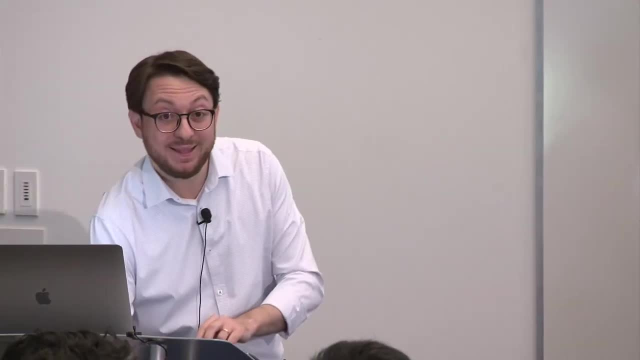 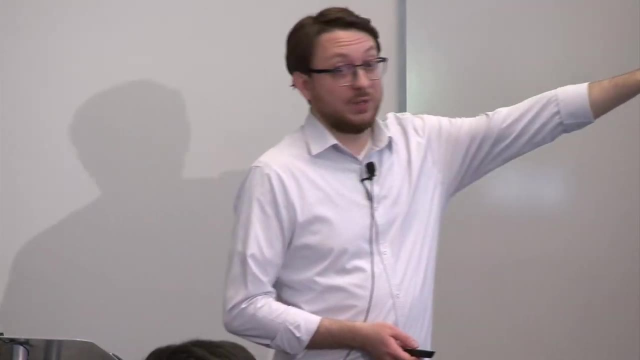 or would they include- I don't want to confuse notation, but in layers and outliers on the objects, for instance, Like if I had pixels inside the object versus outside of the object. sorry, So, that's for SLAM. Yeah, so I think what we do is. 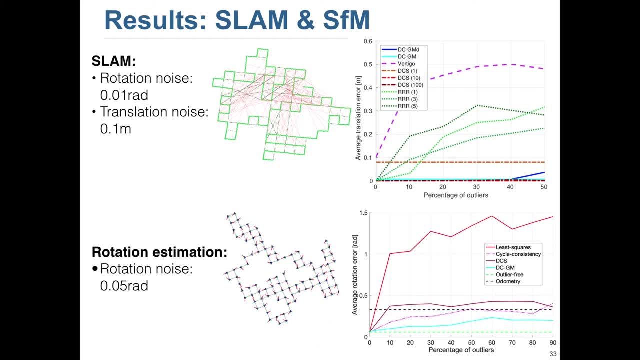 we just pick random pair of poses, add a loop closure, fake loop closure between them and set the fake loop closure to be some random measurement. So they are at random, So set up. here you have like two examples for SLAM and structure from motion. 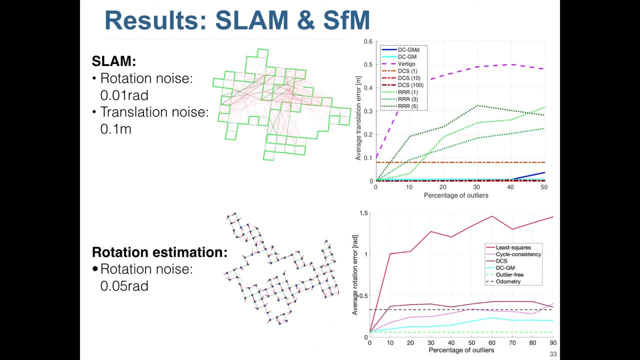 and you get the pose graph, which is this stuff in green and the outliers are the. all the lines are in red. Some rotation noise which is comparable to real application translation noise: 0.1, 0.1, 0.1, 0.1, 0.1.. 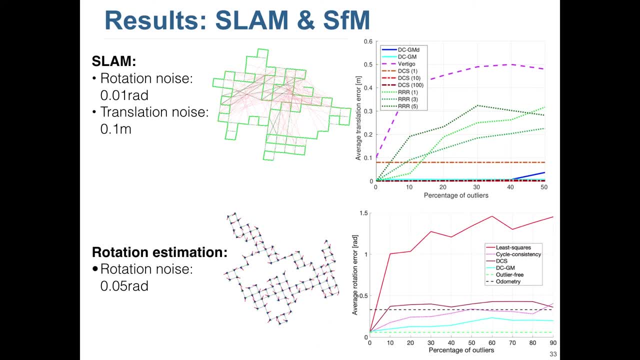 It goes up to 10,000 meters standard deviation. and here what I'm showing is that for increasing percentage of outliers I'm showing how well we can reconstruct the trajectory of the robot. So these are narrower, so lower is better. 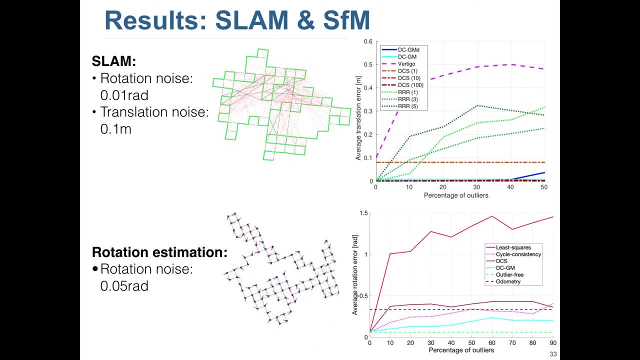 They're comparing how to approach, against a number of set of that techniques, how it approaches this quick, continuous graphical model, which is the one in cyan at the bottom You can see it's pretty much flat, independent on the percentage of outliers, which is good. 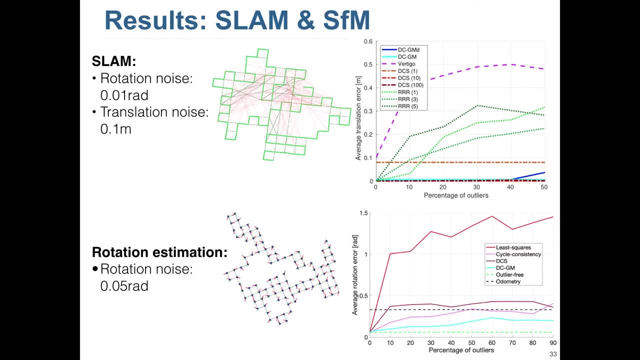 And where, comparing against a number of other techniques which pretty much for outliers you know, larger than 10%, And if you're not careful about the way you do parameter tuning we'll get like a quite large error. And DCS is interesting because, depending 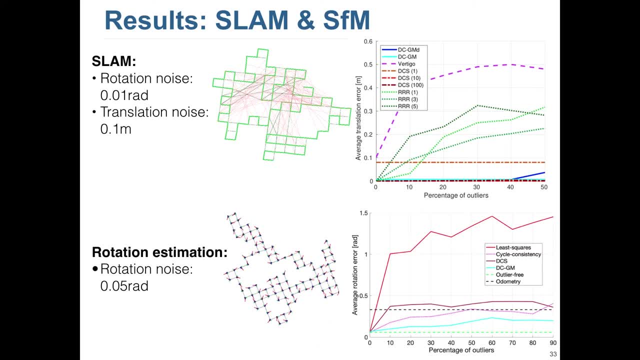 on the parameter tuning can get like a bad error or can get like good performance, So it's very sensitive to that And, by the way, like the default value for that parameter is, here are different values of the parameter one: 10,, 100. 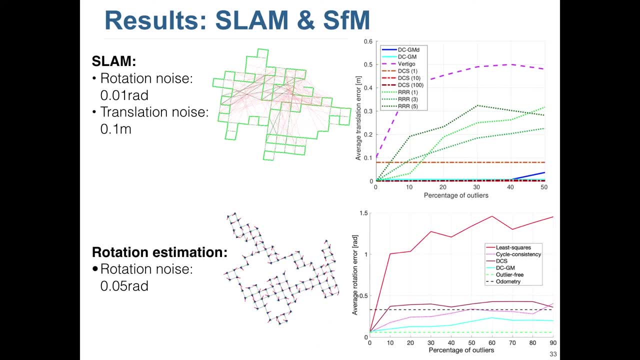 The default that the paper suggests is one which is the one that doesn't work: Rotation estimation. that's like the same problem, but instead of estimating poses attached to the nodes of the graph, you just estimate. the rotation is a popular problem which shows up. 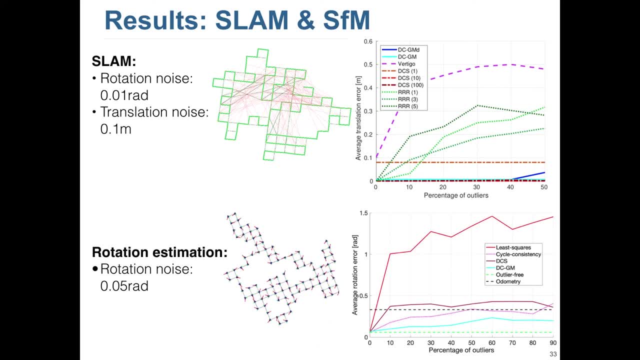 in structure from motion. And here again we are comparing DCGM, which is the approach which is down here in Cyan, with a number of other techniques We can get, like you know, much better. The interesting thing here is that even when the rank 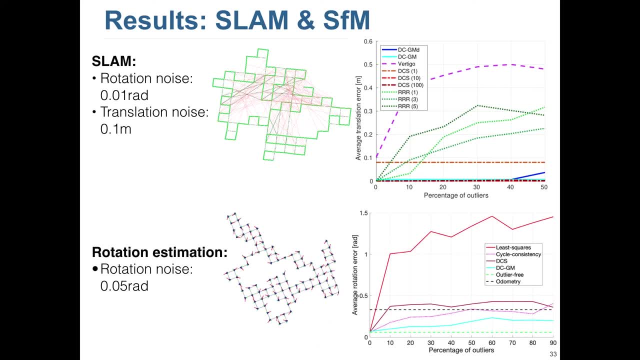 is not D, even when the relaxation is not exact, the error is still there. The error is still better than the others, which is something that we need a little bit more investigation. We don't know why. Here, the only thing that is better. 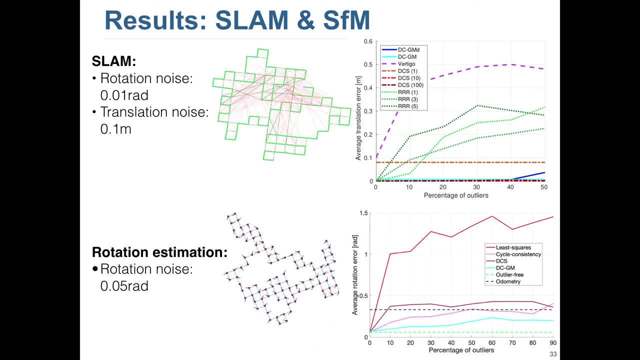 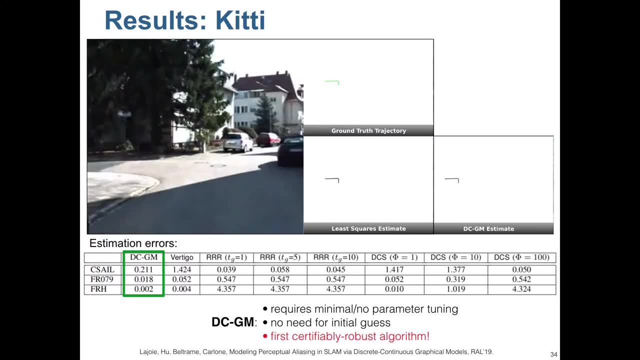 than the proposed approach is the green one, which is the ground truth, like you know, without outliers. Okay, so it's not another technique. Okay, more real results, like on the KIDI dataset standard, SLAM benchmarking datasets. 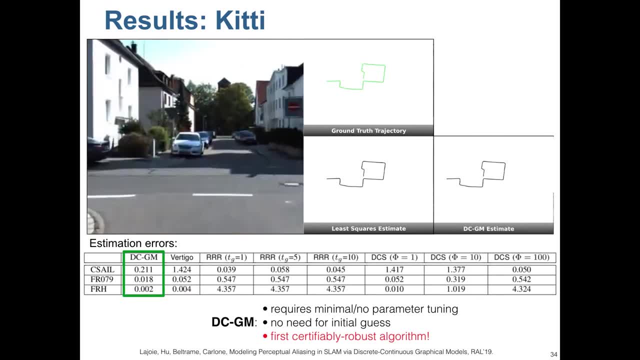 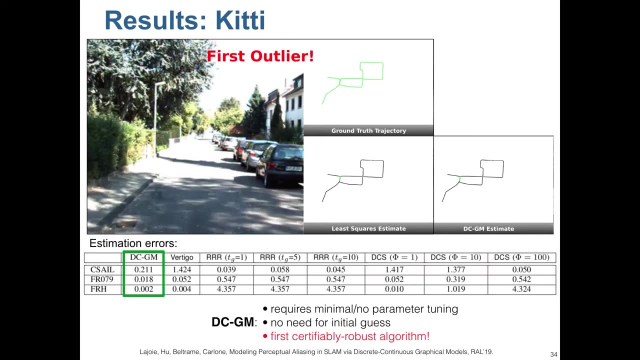 Here the message is that you know, this is our approach and the error for our approach, and this is, you know, the RRR and other technique for different choices of the parameters. In general, we are doing better, although there are like. 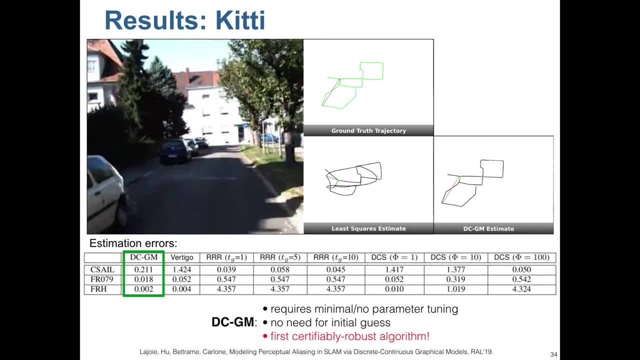 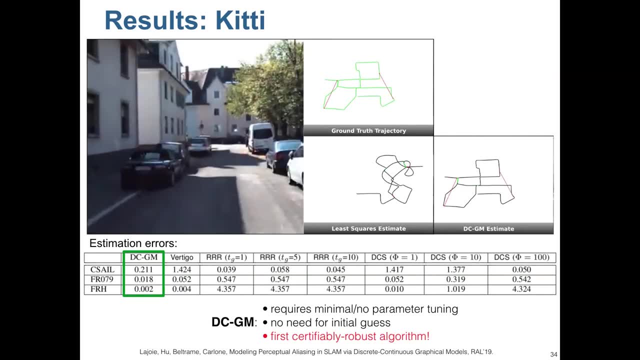 setups in which you know there is no algorithm performing the best. And here I'm showing a video in which this is the ground truth trajectory of the robot of the car. This is the least square estimate and that's the robust estimate with our technique. 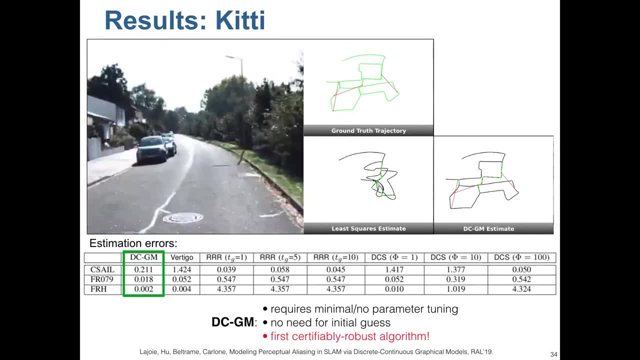 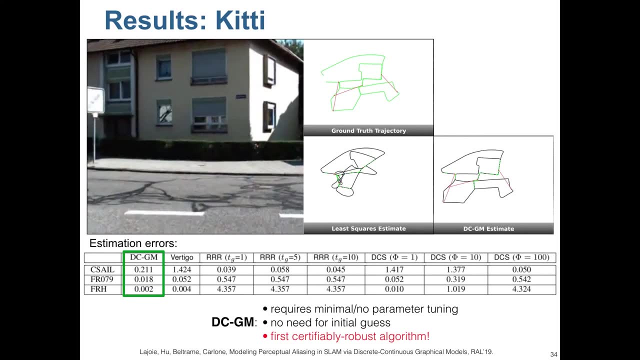 And in red again, you see, like outliers which are due to bad place recognition. So at the end we have this. This is an idea which is an algorithm which requires minimal to no parameter tuning. We just have to set this C bar. 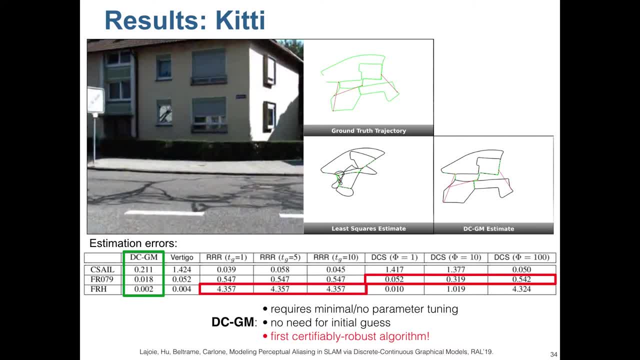 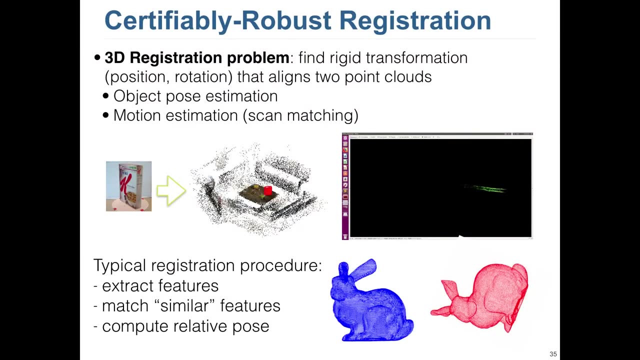 Does not require initial guess, because we end up having a convex relaxation of the problem, And it's the first example of certifiably robust algorithm, So it's indeed feasible in certain regime to get this kind of certifiably robust algorithms. I want to spend the next 10 minutes or so. 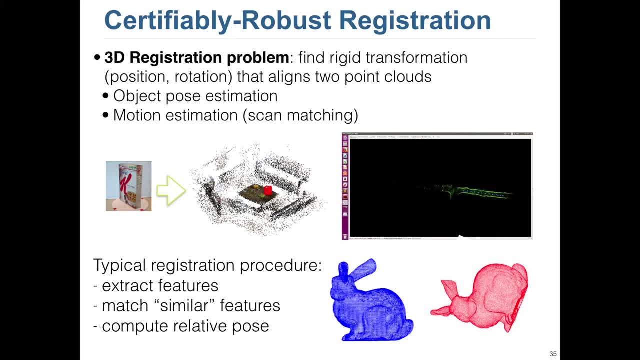 telling you results about certifiably robust registration. The nice thing about this is that the results that we end up having- Yeah, So you're still assuming the correspondences are given- right, But can be wrong. What's that? But can be wrong. 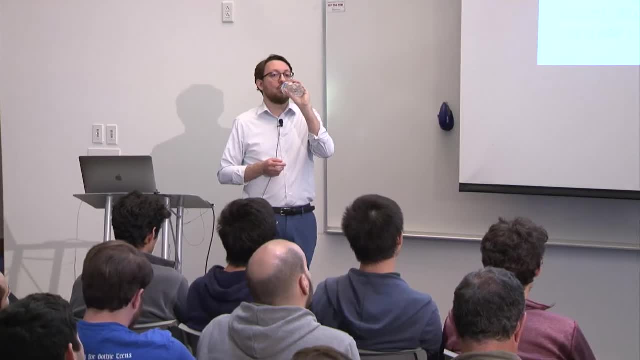 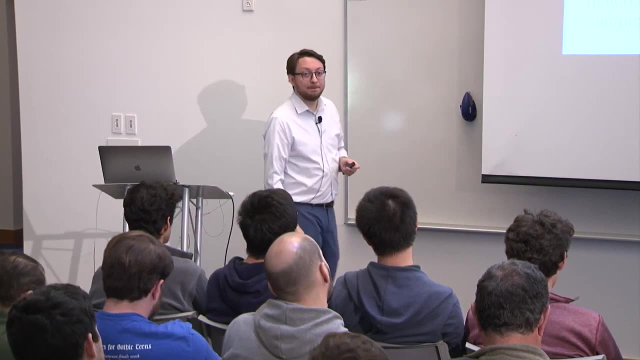 Right. So to what extent does outlier rejection give you robustness to bad correspondences? And because they shouldn't come in just this Gaussian way, but they come in some correlated way. So do you feel like you're also addressing the correspondence problem implicitly? 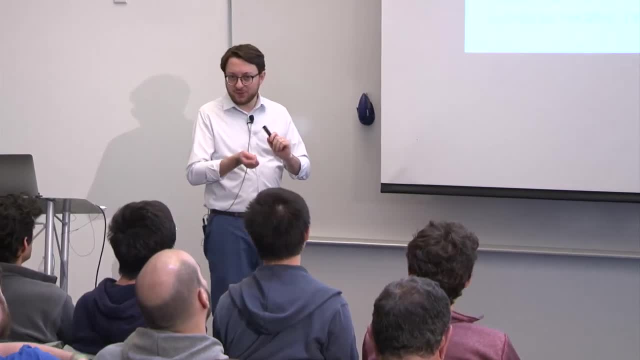 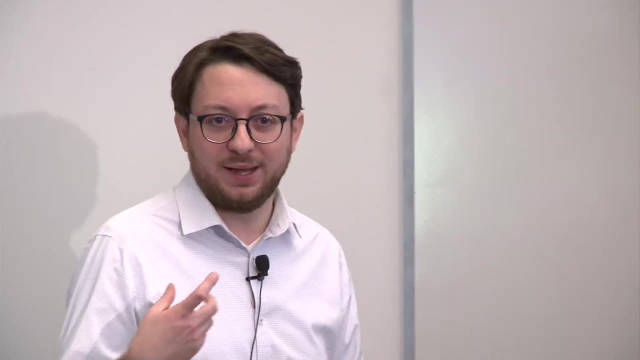 So the outlier and liar decision will decide on the result. So I think that some correspondence is being good or bad. And if you're worried about if you can capture the correlation between inliers and outliers, I didn't tell that because I didn't have time. 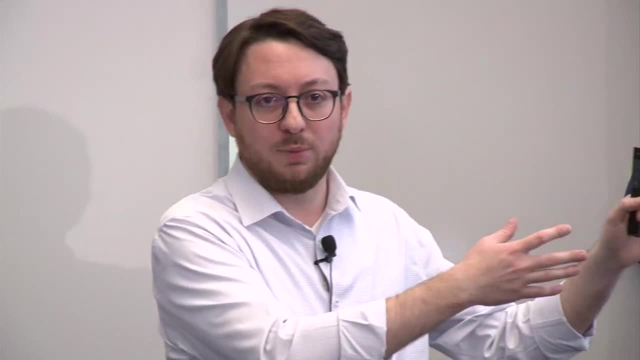 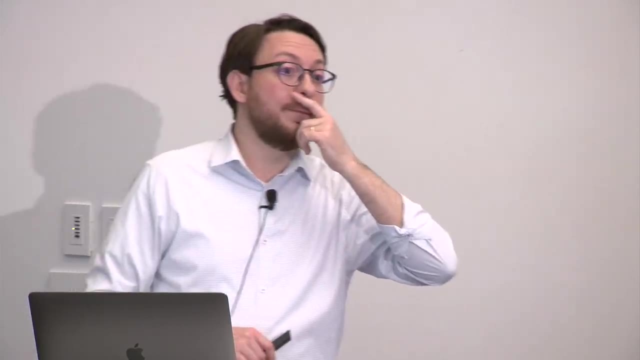 But you can explicitly model. If you know that there is some correlation there, you can also model that in the problem. So you can say that some correspondence correlated to some other correspondence That is about the SLAM problem. So yeah Well, are you done answering the question? 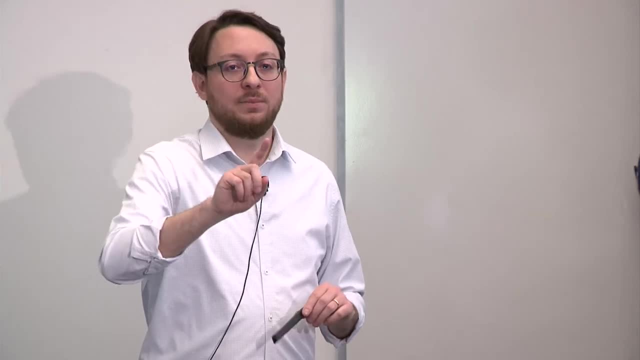 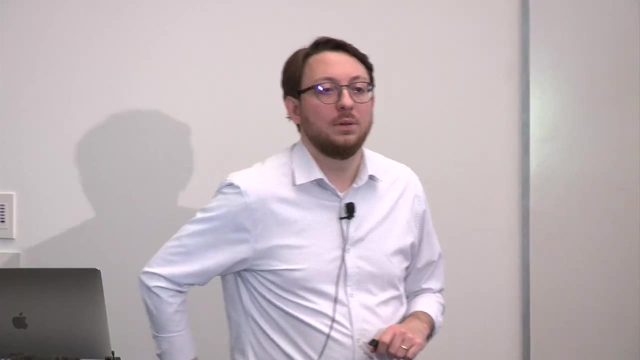 I think so Sorry. Yeah, I was wondering One more thing. The correspondences part would be clearer on the registration part. That's why I'm going fast. I was wondering if you tried augmenting the cost function to promote ranking solutions. 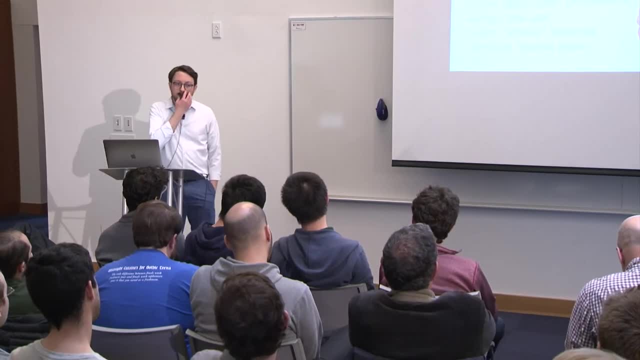 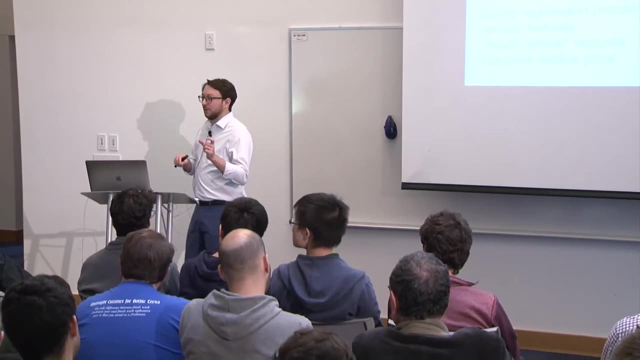 No, it's a good idea. I think it's a good idea. We tried with some- you're thinking about nuclear norm and things like that- right, What was the question If we tried augmenting the cost function with some cost encouraging, lowering solution? 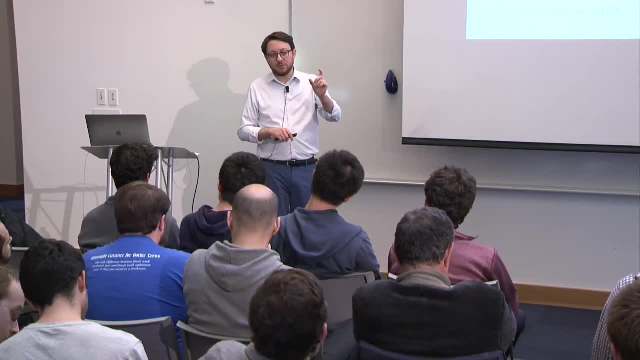 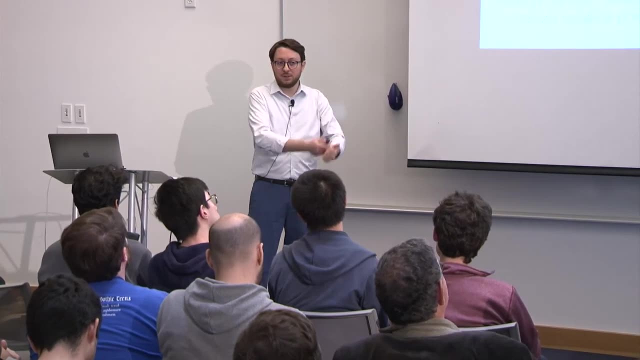 like the nuclear norm. I think there is a little bit of trade-off there, Because the problem is that if you get an optimal solution at that point, you cannot go back and guarantee that you're rejecting outlier and liar because the cost function is sounding different at that point. 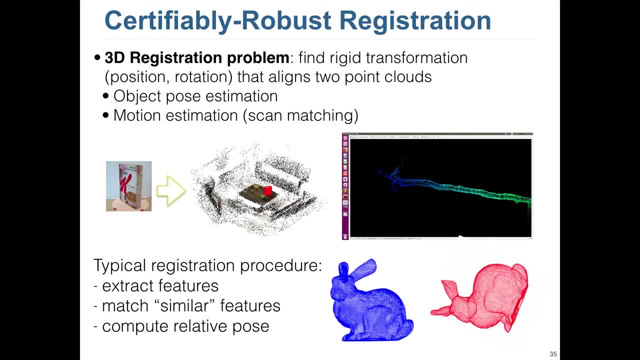 So that's something to think about. So I want to wrap up and to do this quickly and talk about certified robust registration. The registration problem is about finding the rigid transformation within two point clouds And it's a common problem in object that I posed: estimation and scan matching. 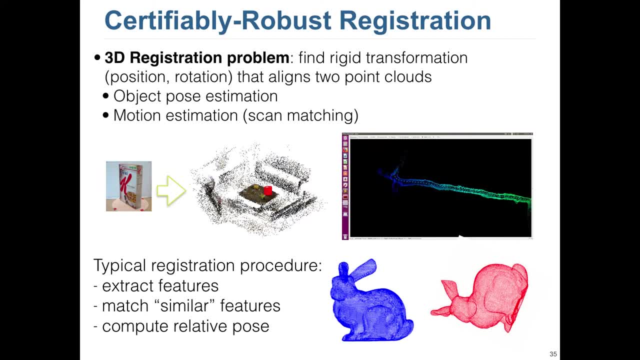 So a typical procedure to do registration. you have two point clouds that you want to match. The first step is that you extract features in these point clouds which can be just point with high curvature. There will be some feature detector there that you can use. 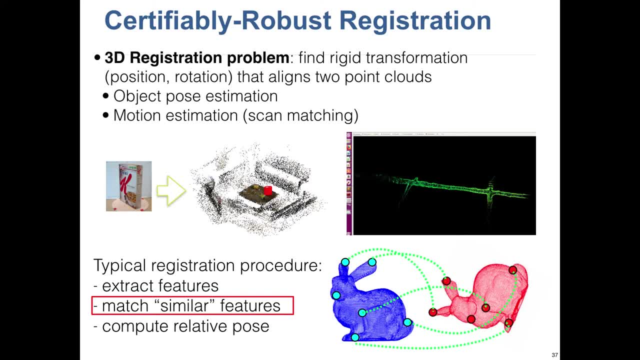 Second step is to match features that look similar. For example, you can attach some descriptor to each feature and then match feature that have similar descriptors. And the last step is to compute the relative pose by aligning corresponding features. Really, what I want to look at is a certifiably robust approach. 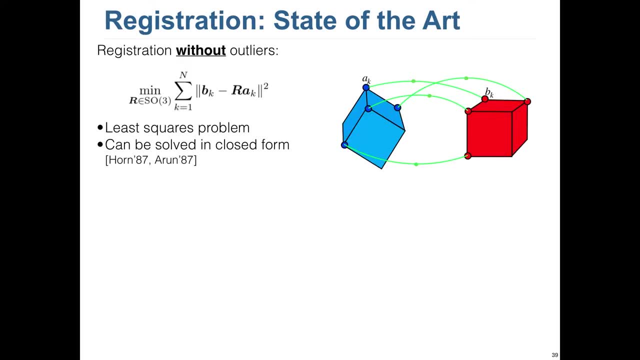 to compute the relative pose. So the state of the art here is that if the correspondences are perfect, so all the correspondences really match one point in the point cloud to the corresponding point in the other, then you can formulate again the outlier-free problem as an all-linearly square problem. 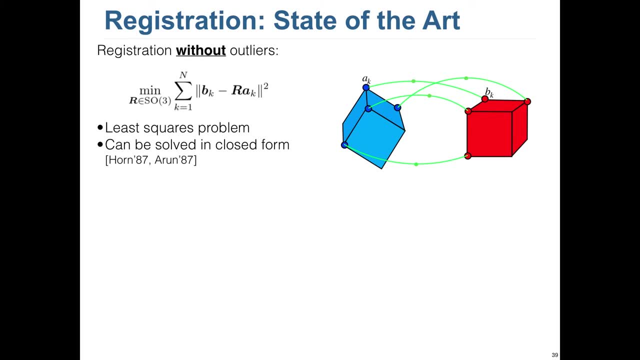 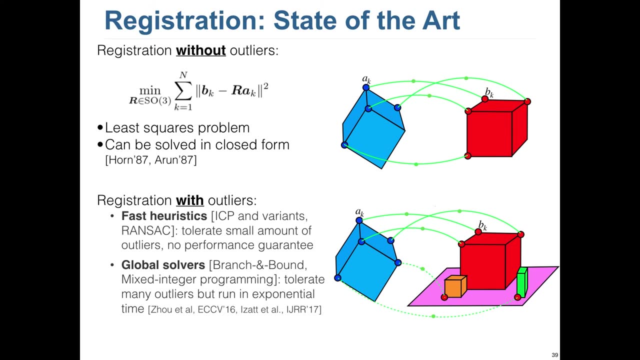 And good news there is that the problem is solved. There is closed-form solution to solve the case without outliers. In the case without outliers, what happens is that some of the correspondences are wrong. this dashed line in the sense that this point. 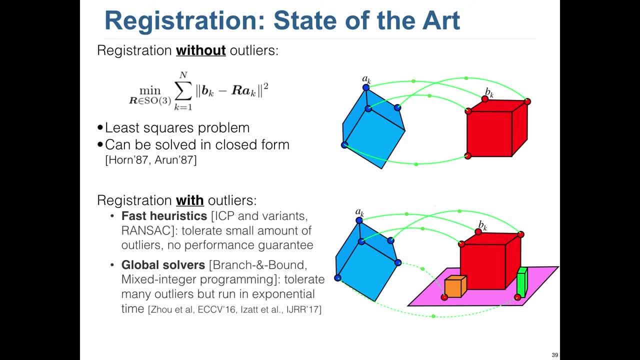 does not really correspond to that point. in the other point, clouds, And I believe there is a little bit of a dichotomy for the case without outliers, and the dichotomy is between fast heuristics which are fast but do not provide performance guarantee. 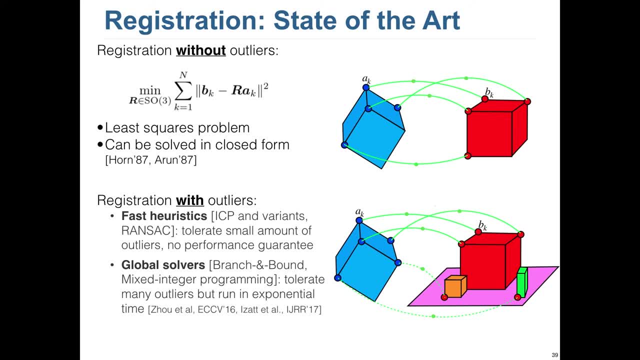 and fail in the presence of large number of outliers and global solvers, like branch and bound or mixed integer programming, in which you do get guarantees but in the worst case they run in exponential time. So the question we ask is: can we develop? 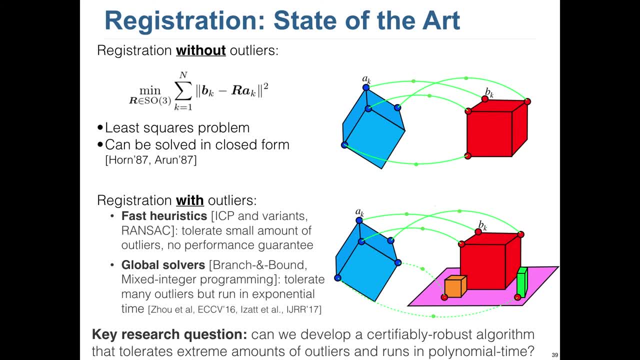 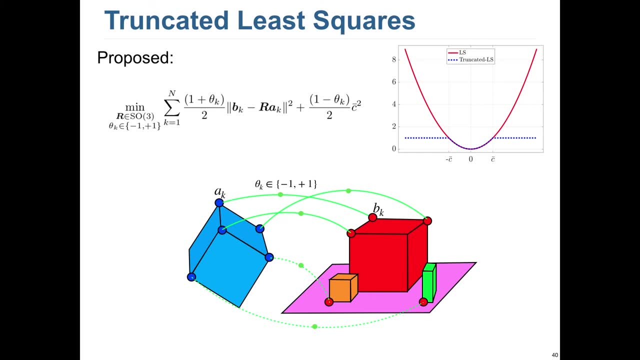 a certifiably robust algorithm that can tolerate extreme amounts of outliers and run in polynomial time. The formulation is the same as before. We have a truncated least-square-cost function in which the theta is decided in between inliers or rejecting the measurement as outlier. 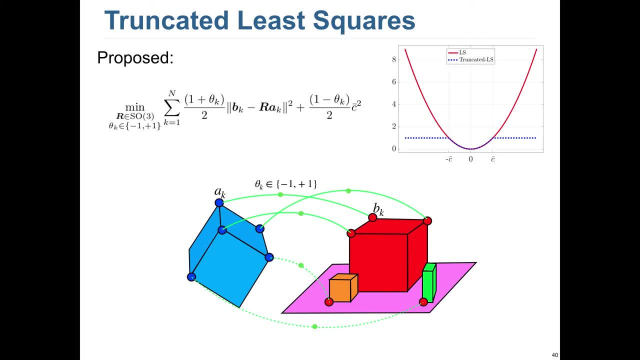 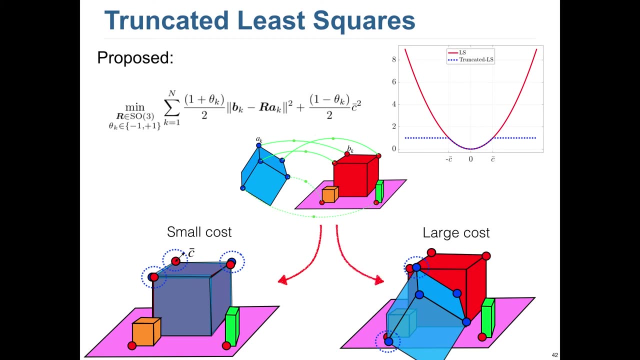 And again it's the idea of the truncated least-square-cost and truncated quadratic cost. I'll go a little bit fast because I'm late, but what I want to show again is that the cost function essentially will try to maximize the number of inliers. 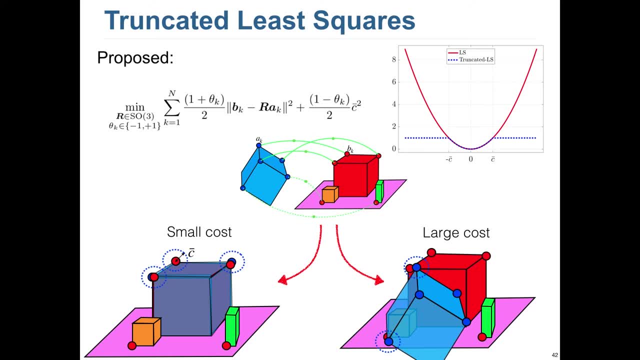 For example, this solution for the problem will explain three: will have three measurements, three correspondences. being inlier, therefore, will have smaller cost than this solution, for example. So really, what the optimization problem is trying to do is to maximize the number of inliers. 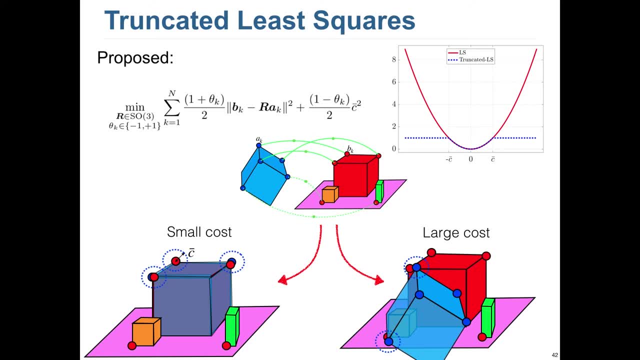 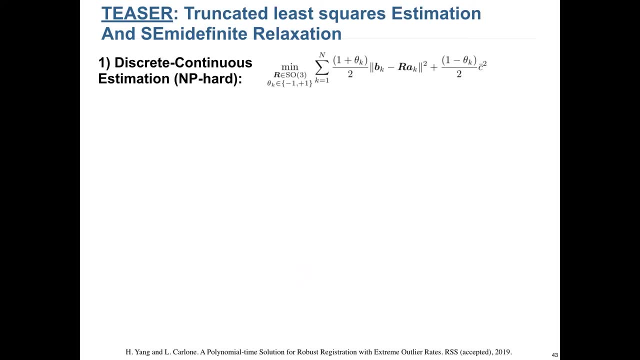 Does it answer or clarify the question that you had? OK, So here we have a similar convex relaxation. I will not show you how to get the convex relaxation, but you have an idea which is pretty similar. It's like the version 2.0, what I was discussing earlier. 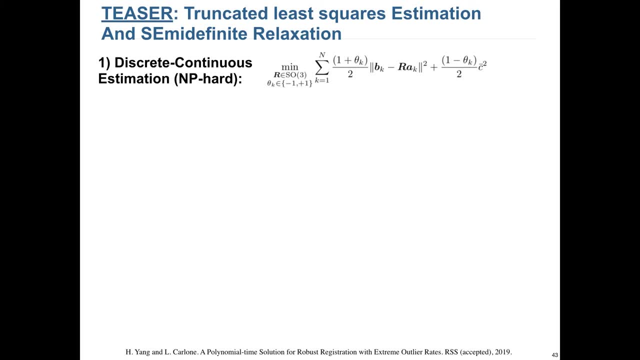 in the talk. So we propose this algorithm, which is called TEASER, which is truncated least-square estimation and semi-definite relaxation. And here I want to give you the teaser of TEASER. We start with this very difficult optimization problem. 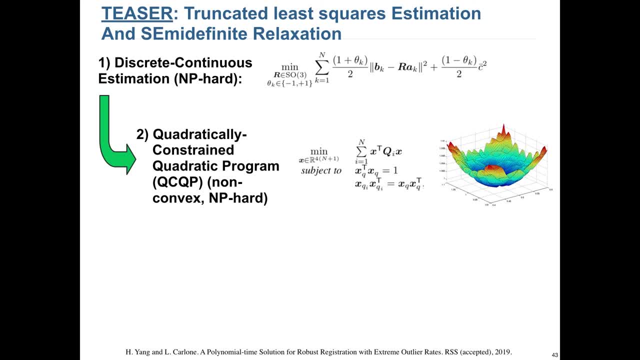 We are clever to reformulate it as a quadratically constrained, quadratic program. There is a little bit of extra cleverness in the formulation with respect to the SLAM case and we do a convex relaxation of it. I'm seeing here the convex relaxation is non-trivial. 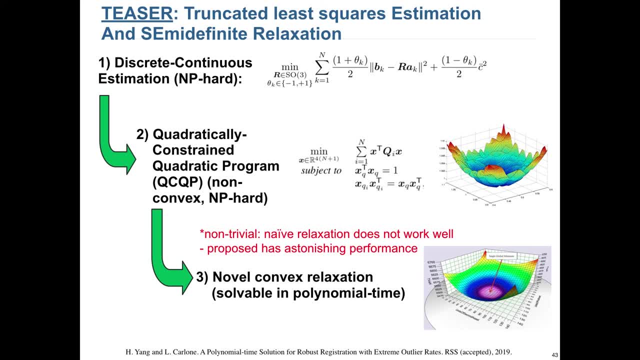 Typically there is a trivial way to get the relaxation of a QCQP. If you do the trivial relaxation, it does not work well. Instead, I will show you that the relaxation that we do has a pretty surprising performance. I believe I spent zero time on these. 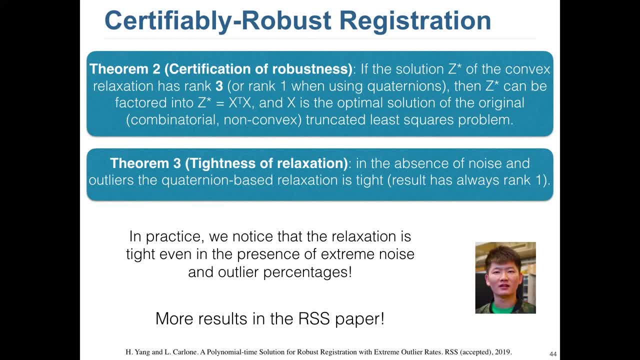 Guarantees are pretty similar to the SLAM case. If you solve the convex relaxation, you get the low-rank solution, You are solving exactly the original problem And, in particular, if you get the rank one solution when formulating the problem with a quaternion formulation, 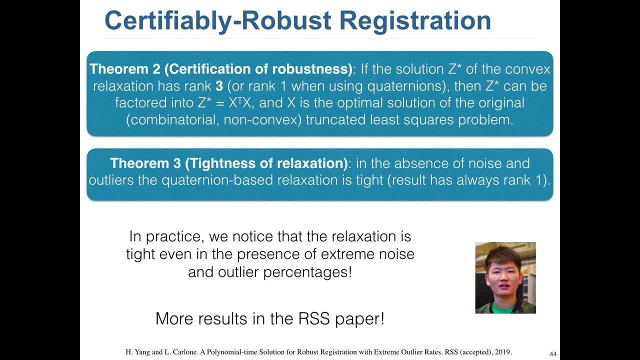 you are solving exactly the original combinatorial problem And Hank, who is the mastermind, the mastermind of this paper, was also able to show that in some cases you can prove that you get the rank one solution. It's a very simple case. 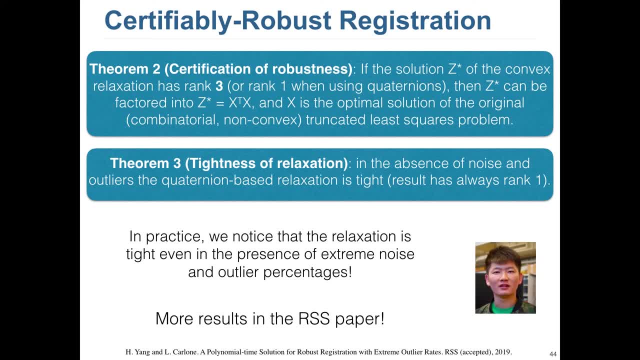 like. no noise and no pliers, unfortunately, but that's a good starting point And this paper is accepted on RSS. There is probably, like you know, five times more than what I'm seeing. Check it out, It's pretty cool. 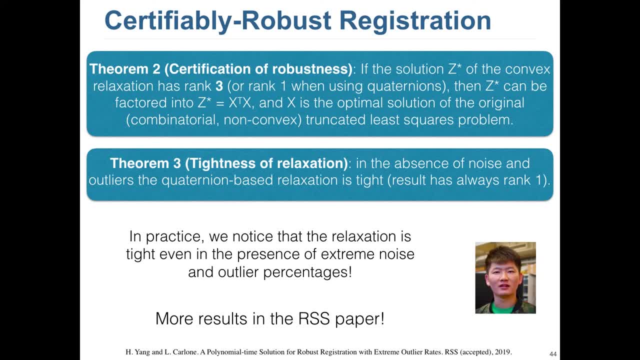 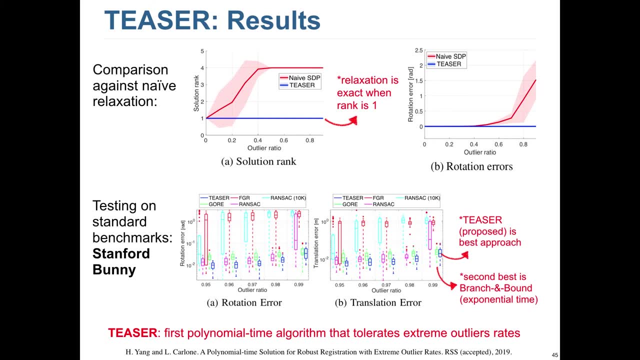 In particular. here I'm talking about how to relax the rotation part, but the paper is talking about scale estimation and translation estimation as well, So I want to spend the last 30 seconds here with the results. so why I'm excited about this. 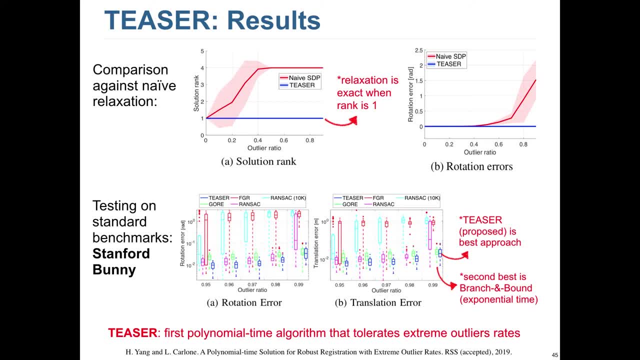 So this is the results for a teaser, and this is the level of outliers, outlier correspondences, that you have in the problem and the rank of the solution. The blue is the rank of the proposed solution, which is the proposed relaxation, and it's always one. 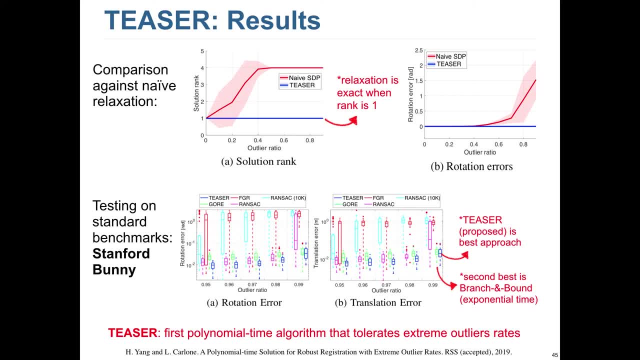 meaning that the proposed relaxation is always tight. If you do the naive QCQP relaxation, it breaks pretty much right away after you have a few outliers, And this of course translates in the fact that the rotation error for increasing outliers is quite flat for our approach. 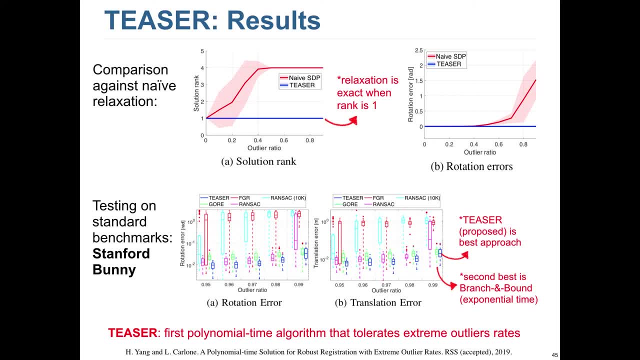 meaning that we are able just to reject all the outliers without problems. We did standard testing on the Stanford bunny, which is a standard data set here, and these. I want to tell you a couple of things about these results. So first of all, these are results. 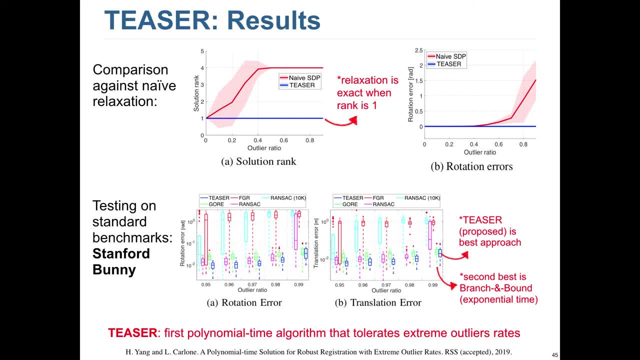 for outlier ratio up to 99%, which means you have 1% of good data. The other one is just clutter And I'm showing the rotation error and the translation error for a number of approaches, including RANSAC, fast global registration. 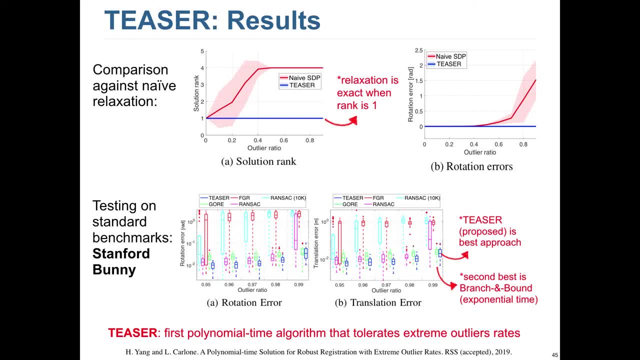 which is a state-of-the-art approach, and GOR, which is a branch-and-bound approach, And our approach is TESER, which is the blue one. so it's the smallest error, both in terms of rotation and translation, And we are happy because it's a very low error. 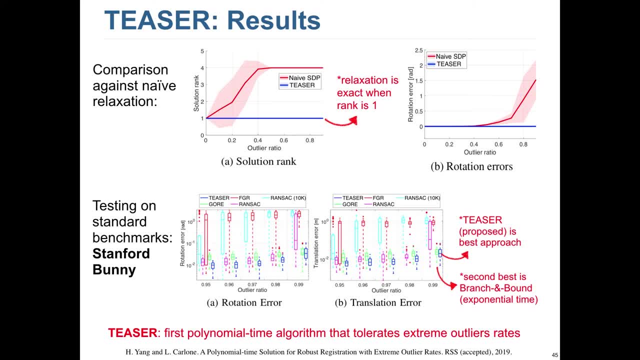 but we're also happy because this is a polynomial-time algorithm, while the second-best approach, which is the one in green, is GOR, which is branch-and-bound, It's exponential time, So we are doing even better than an exponential-time algorithm. 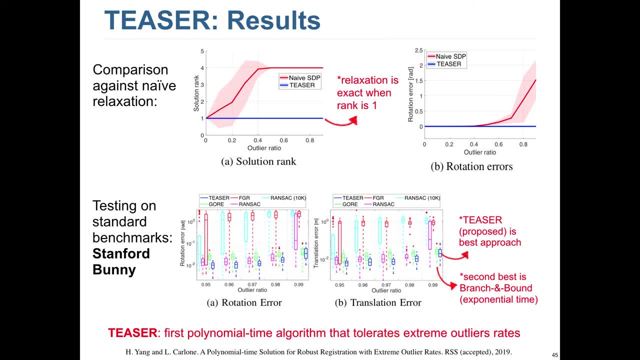 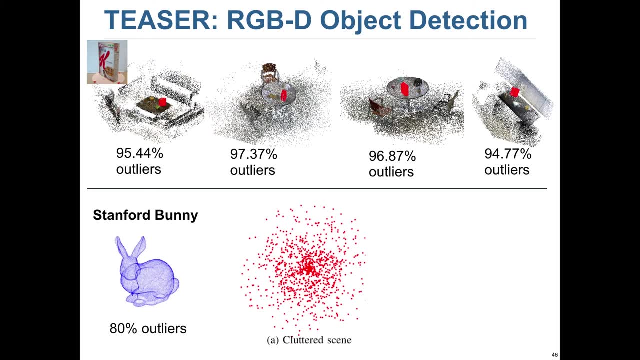 So TESER, at the end of the day, is the first polynomial-time algorithm that tolerates up to 99% outliers. I'm running late. This is to show that, in practical point, cloud registration problem is not uncommon to have. 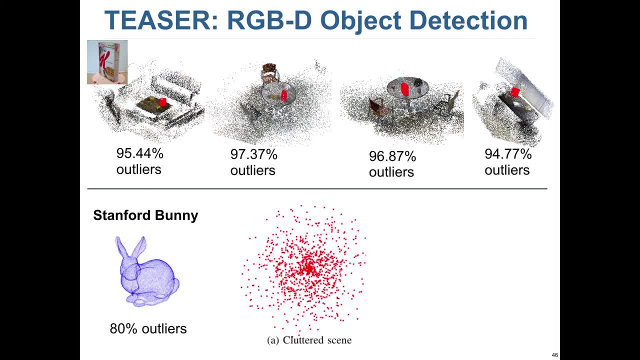 a really huge number of outliers. so it's really important to go to approaches which are resilient to a huge number of outliers. So, for example, in this problem RGBD dataset, you can get anything you know between 95% to 96% of outliers. 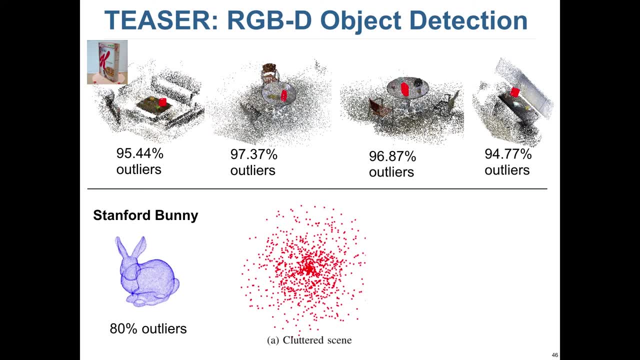 And to tell you that these are indeed difficult problems to solve, I'm showing here an example in which we have the Stanford bunny, We downsample it a little bit and then we add 80% of outliers, 80% of random points. 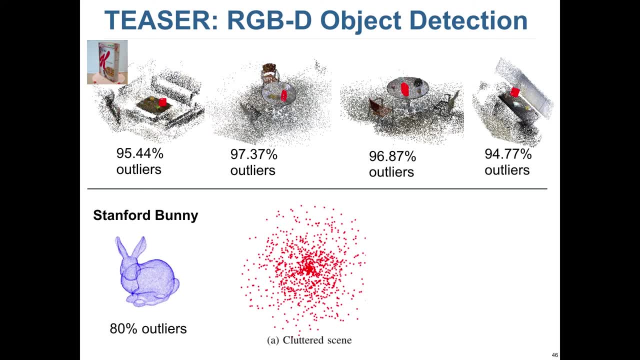 Do you guys see the bunny in the red? Kind of yeah. So the algorithm you know is returning the optimal solution. It's certifying that this one in green are indeed in outliers And of course, this is a setup. 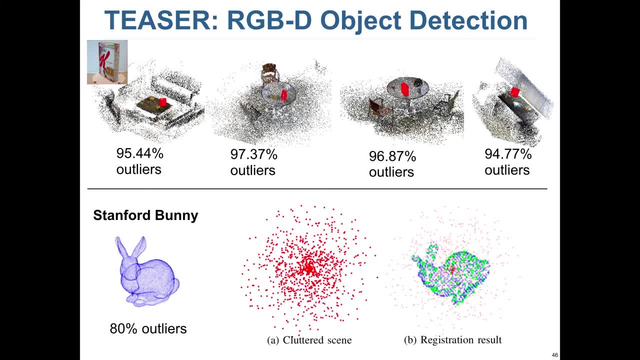 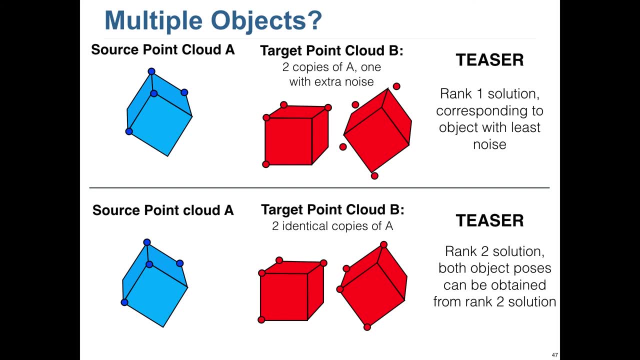 in which the algorithm for the algorithm, it's pretty easy, It's 80%. The algorithm is able to go up to 99%. okay, And this is a very cool example, but you know I'll not go over it. 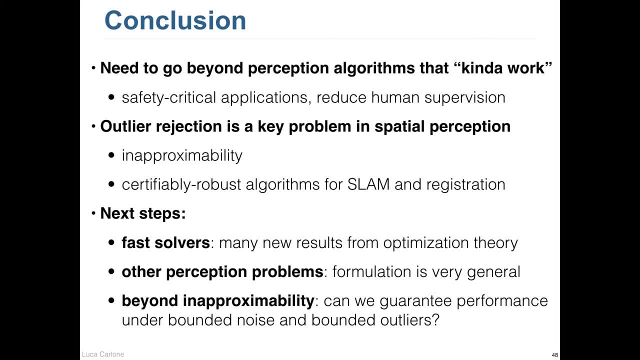 If you have questions about multiple objects, just ask me. To conclude, I believe we need to go beyond algorithm perception algorithm, that kind of work. We really need to do that, to go beyond, to enable safety critical analysis of the critical application. 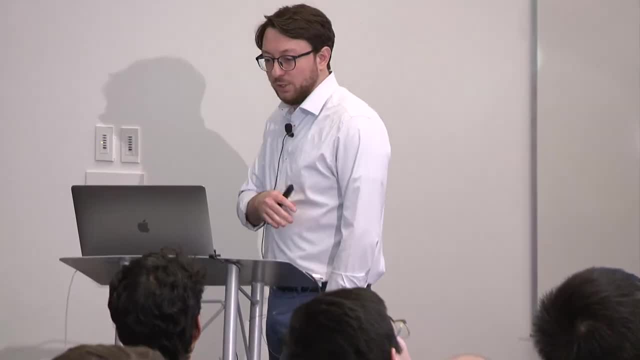 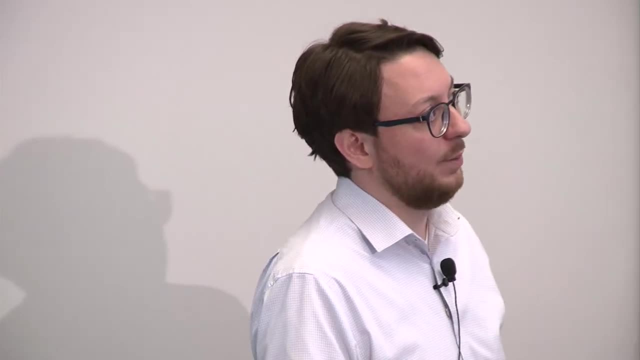 and to reduce the human supervision, And I will show you in this talk that outlier rejection is a key problem and unfortunately it's inapproximable. but it's still possible to design certifying robust algorithms and I show you two examples. 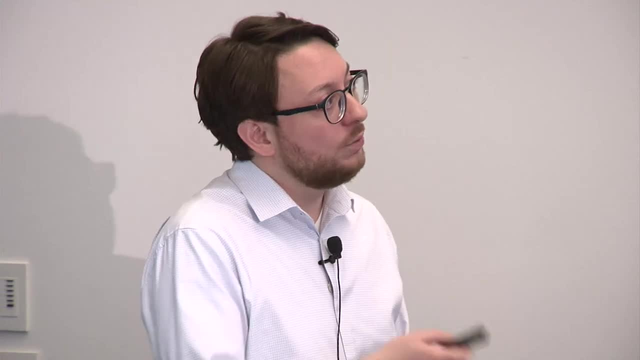 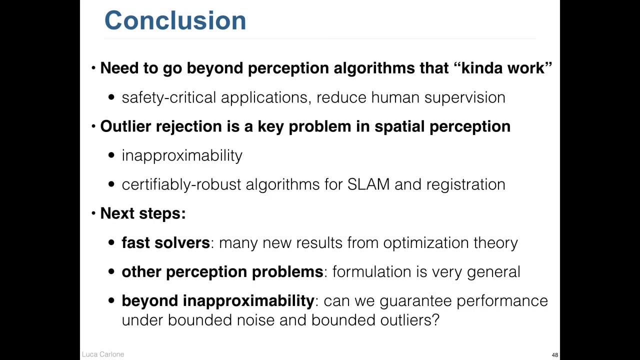 one for SLAM and the other one for registration. What we want to do next is really like to put out fast solvers to really like enable large-scale solution of these problem instances. And since we believe that this truncated, least square formulation is quite general, 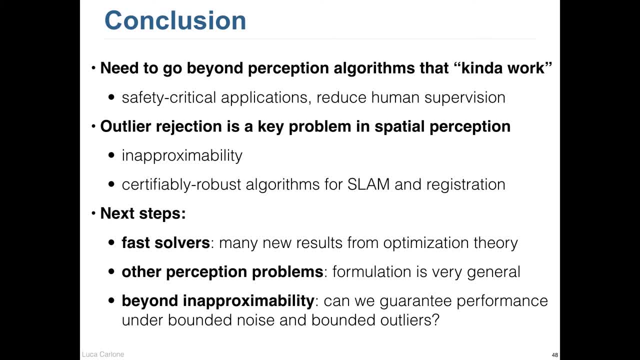 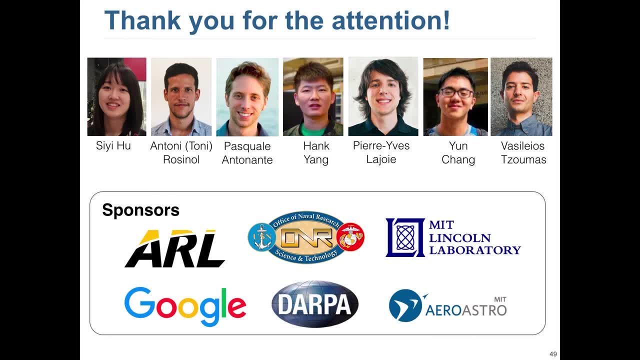 we would like to do to use it for other perception problem. We are still exploring that. Of course we'll get some theoretical results to go beyond inapproximability. So, guys, I'm already late. I want to stop here. thank every student and postdoc in my group. 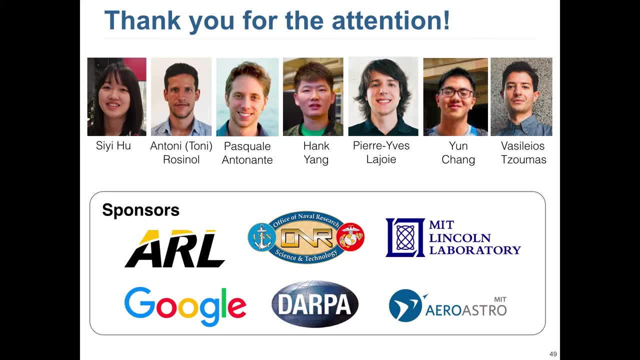 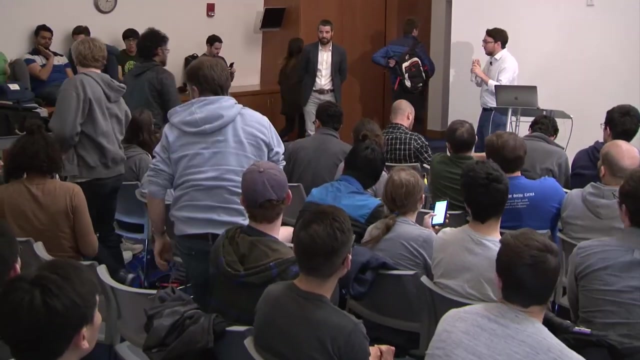 They're really doing the hard work like behind these slides. Thank the sponsor and thank you guys for the attention. I'll be happy to the questions. Hi, when you saw the STB reactions of the correspondence problem, how often do you get matrix? 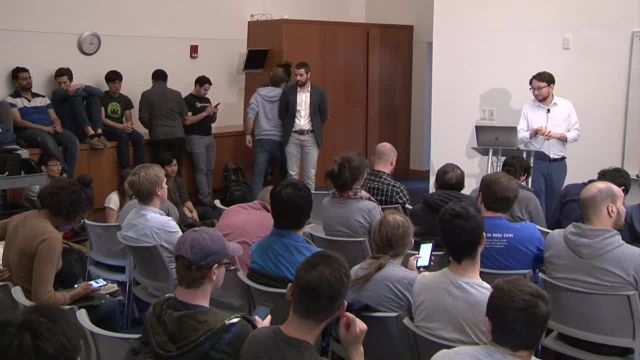 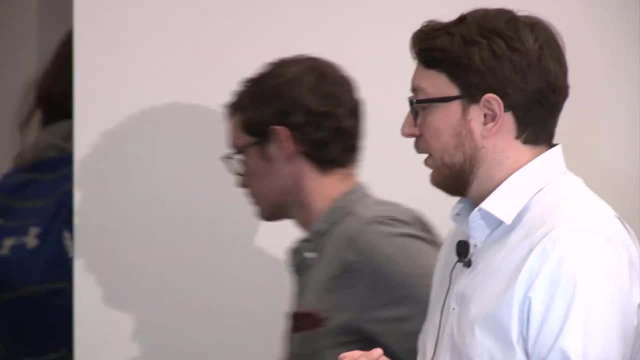 that's actually rank D And when it's not rank D, can you do some running to project it back to the feasible set? Yeah, so first of all. So that is problem dependent right in the sense that here what we can prove is that in some cases 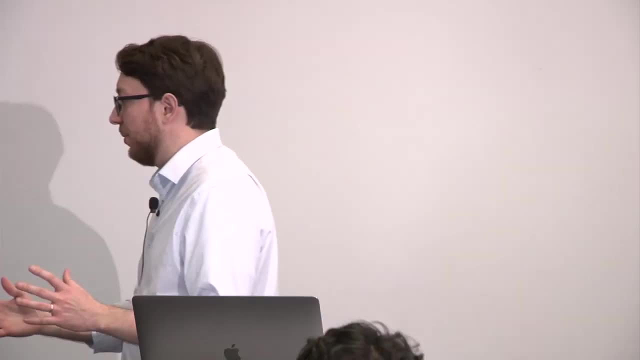 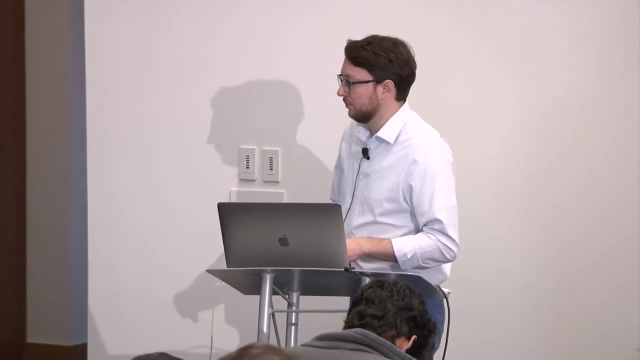 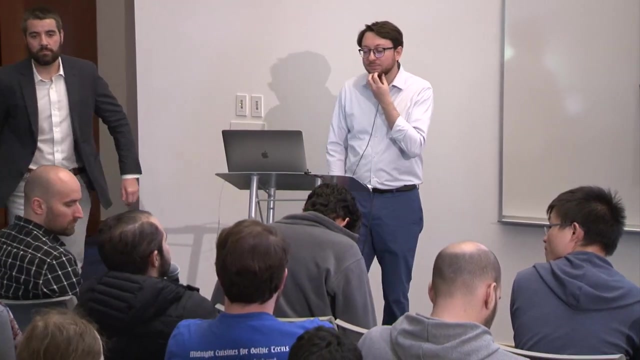 when the noise is more or when the outlier is not. they're not, you know, huge number. you do get rank D, So there are regime in which you can prove it, but that's not true for generalized DP. So can you elaborate a bit more on which are the specific? 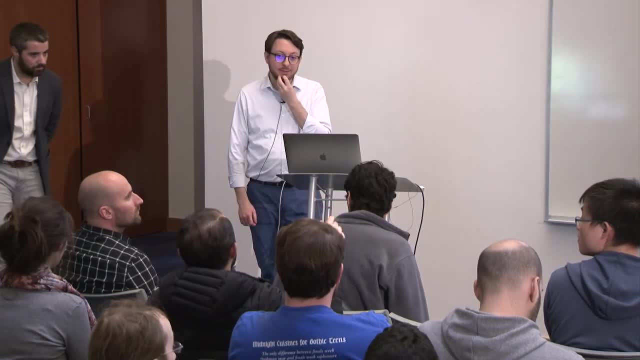 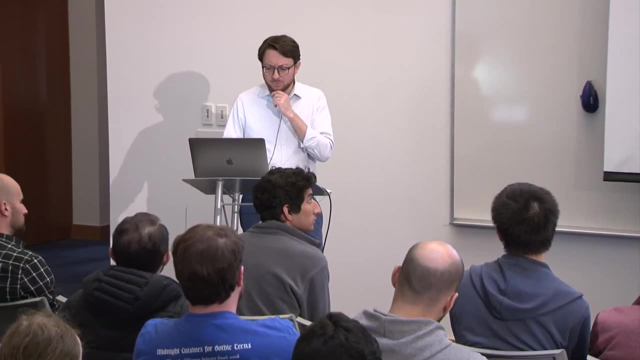 conditions that usually lead to like non-full rankness in the optimization problem. Like more, like in a numerical sense. you know what does it mean to have more outliers in that sense, The numerical addition which, which, What makes you kind of like break that rank condition. 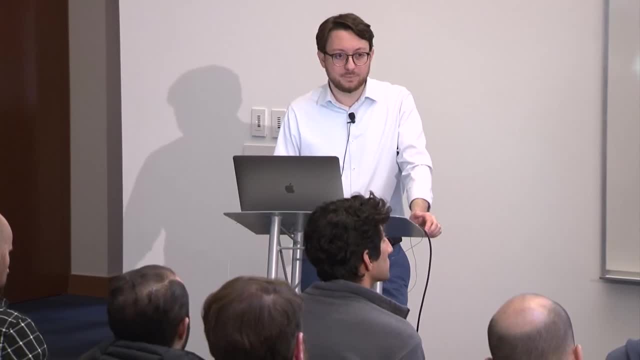 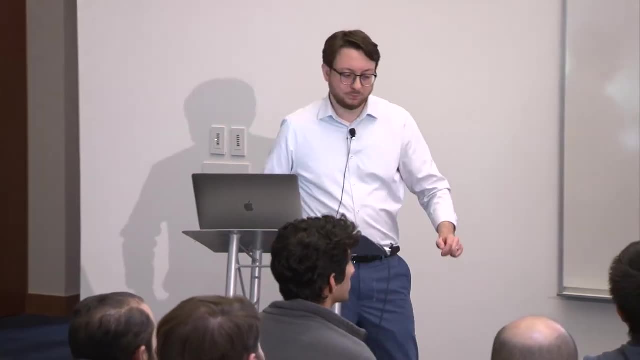 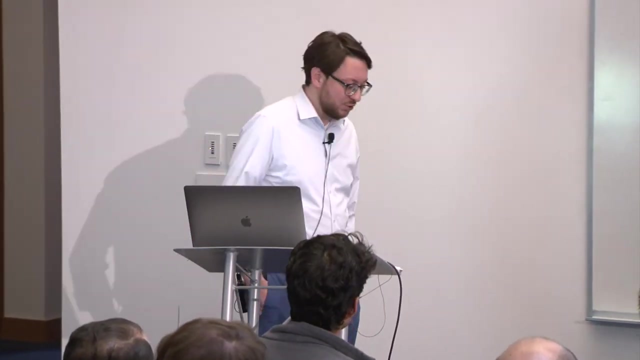 like. you know what kind of like makes you have a higher rank. you know, can you like elaborate? you know why does the solver find that to be the optimal solution? sometimes, Typically, the way you can prove this, I do not have like a huge intuition. 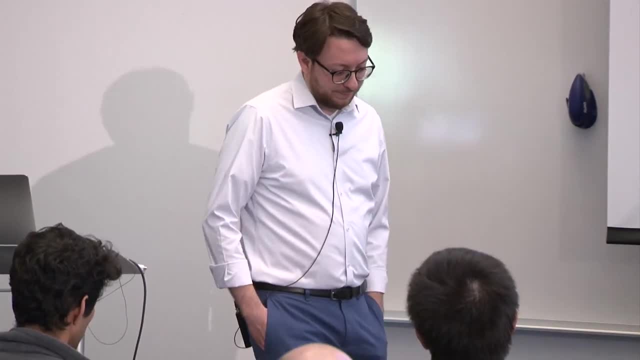 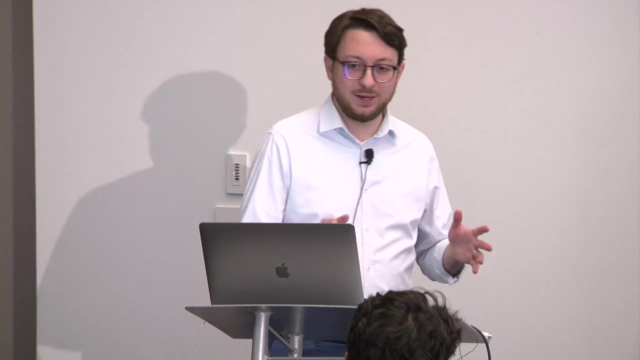 but that typically the way you can prove this is that the rank constraint becomes redundant when you have no noise, in the sense that even if you try to solve it without that constraint, you still get like a rank dissolution. And what you can prove typically is that if you start adding 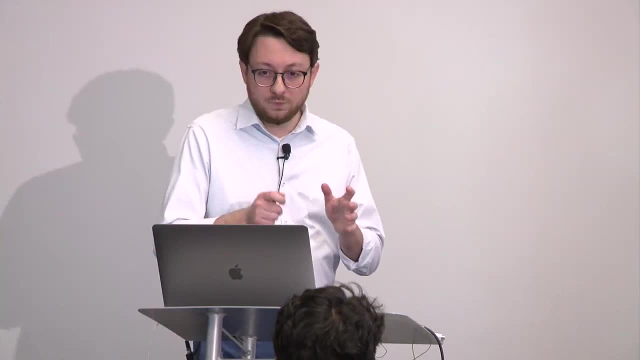 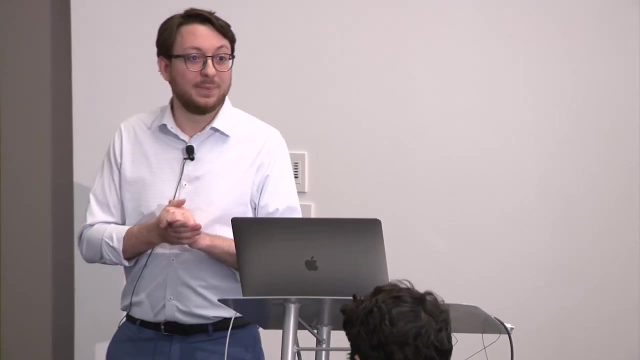 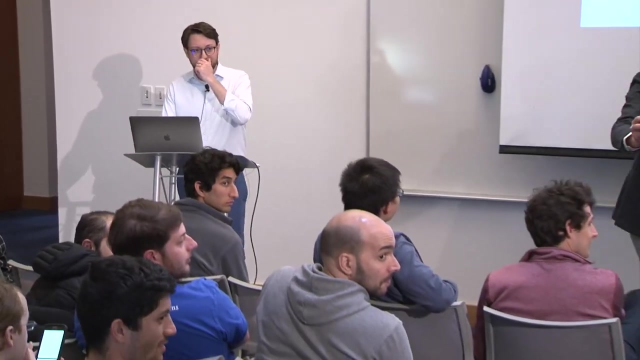 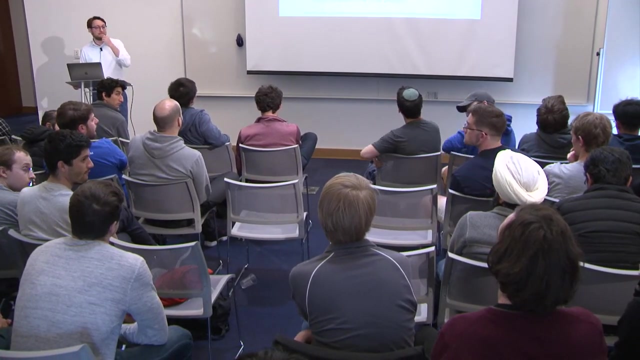 a little bit of noise. that remains true for a while. That's the only intuition that you have so far, that I have so far. Thank you, And we're going to continue with the initial question. Would you like to wrap up with a question? 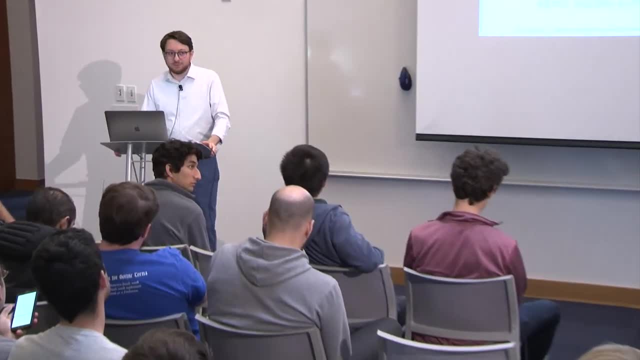 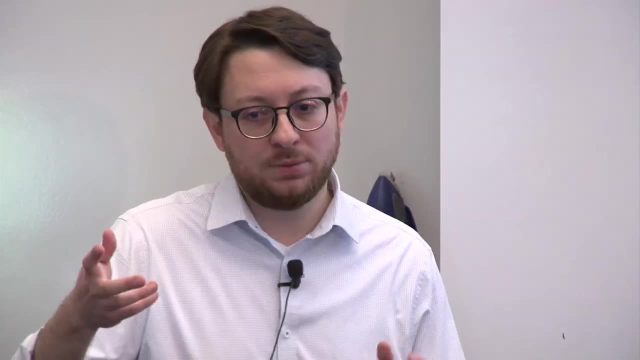 So you dropped the determinant condition on the rotation matrices. Did that result in any problems For this lamb problem? we did that for, like for many different types of relaxation, What turns out is that in practice you get a solution and you can get either rotation with a terminal plus one. 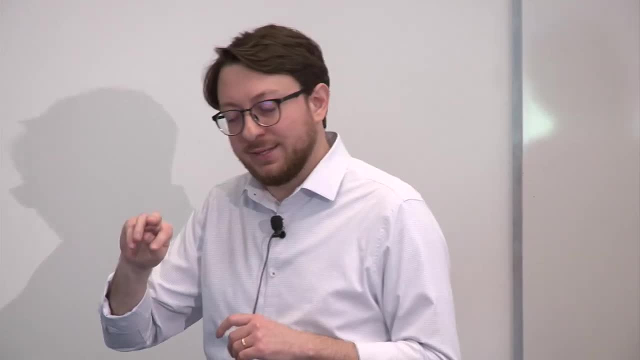 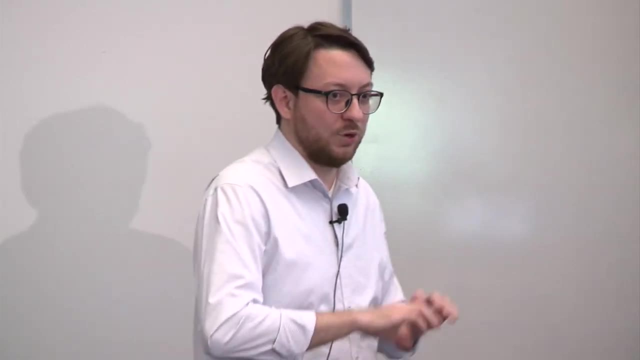 or reflection with a terminal minus one. What ends up happening once you relax? that is that either you are lucky, you get all rotations or you get all reflections, for which you can change the sign and still get the right rotation. So it's not a big deal. 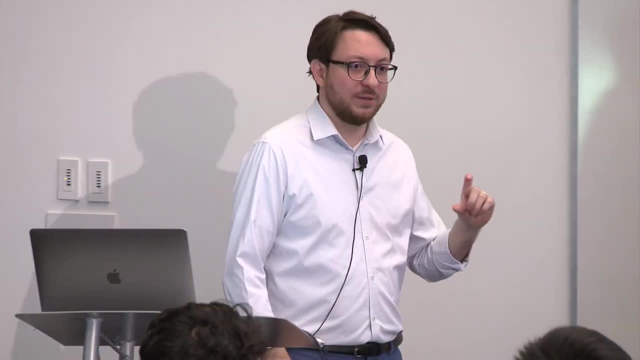 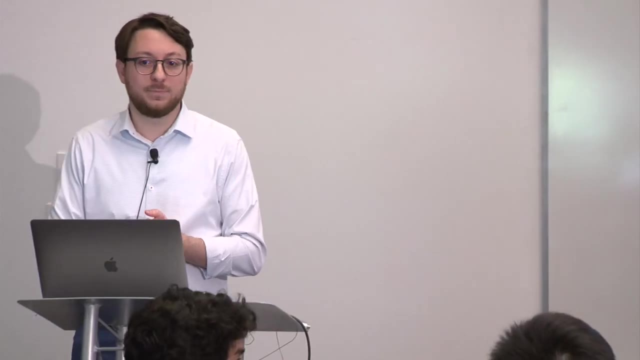 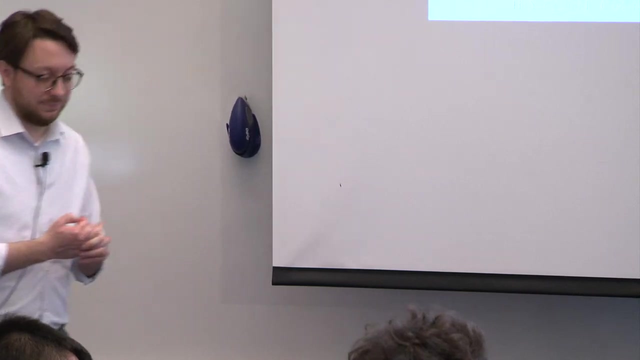 And you can prove it, that if you have moderate noise will never happen, that you have a rotation and reflection as part of the solution. You can prove that formally, Yep. So my general question back to your three axes And do you have a sense of whether humans can do SLAM? 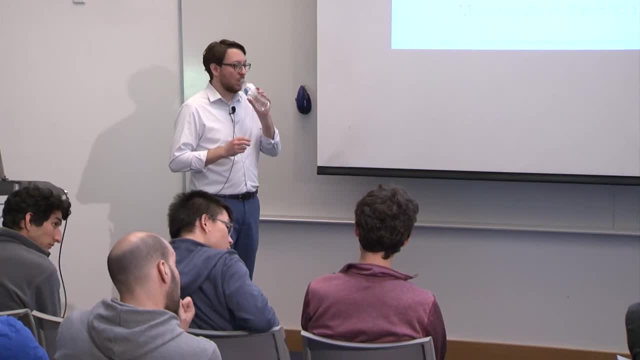 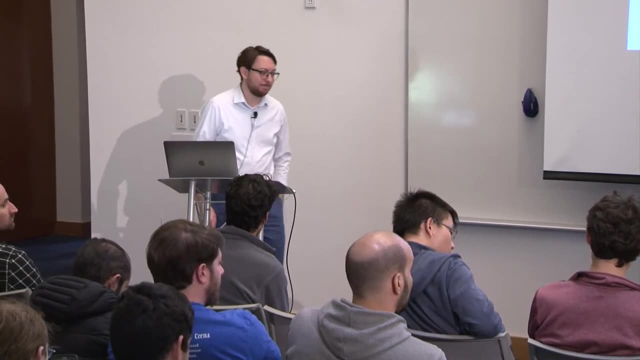 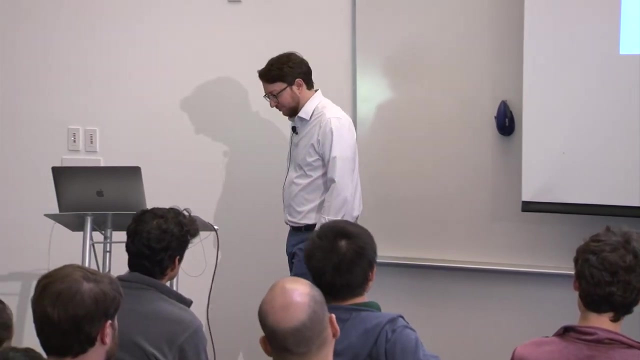 well, So if you put one of your grad students in the tunnels and told them to map it, could they do it? Or how bad are the computer results? like the other alternative algorithms to what a human could do? or a sense? Yeah, we definitely get lost in the tunnel. 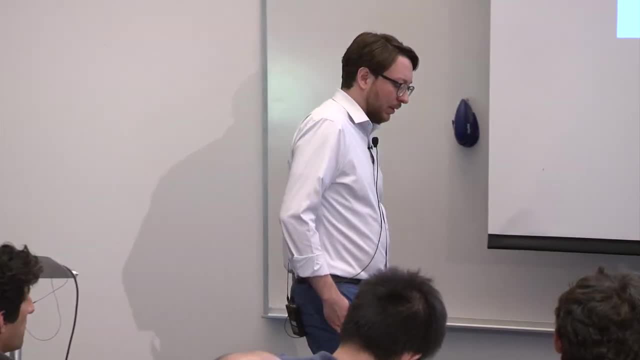 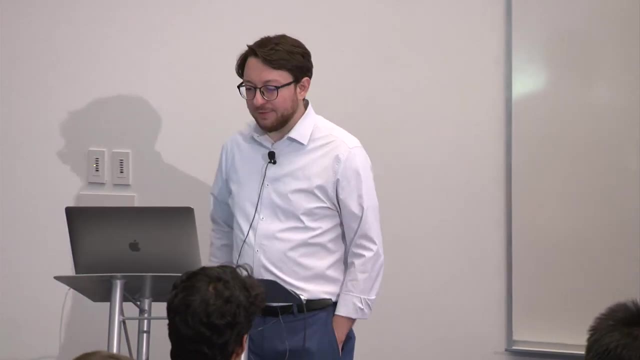 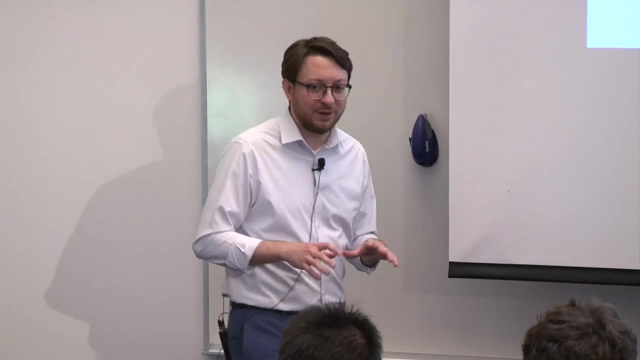 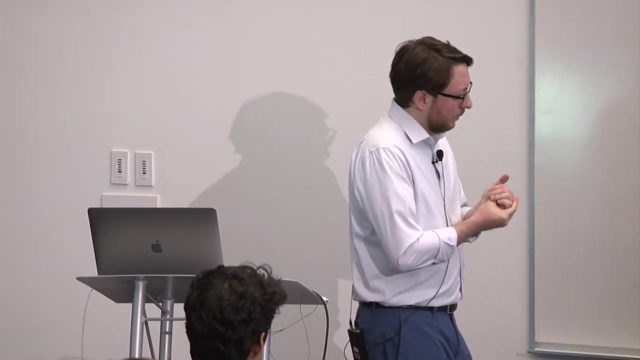 I can tell you that, Yeah, Something that humans are much better doing is leveraging multiple cues like semantic cues, appearance geometry, Like combining all these. definitely, humans are much, much better, Probably on the SLAM side and on the just purely geometric side. 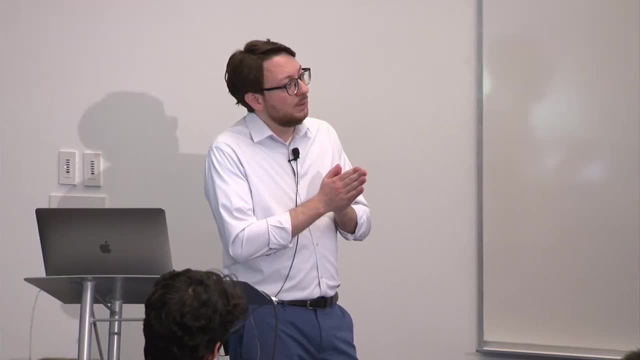 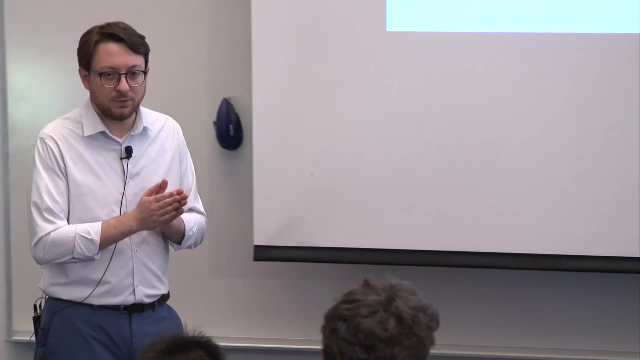 yeah, So what I was going to say is that I put humans there, but it's somehow like an unfair comparison in the sense that it depends a lot on the sensor that you put on board. Humans are constrained in the set of sensor, Contrary to what Elon Musk says. if I put a light there, 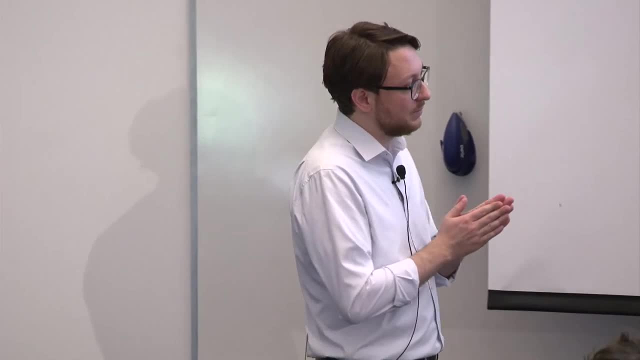 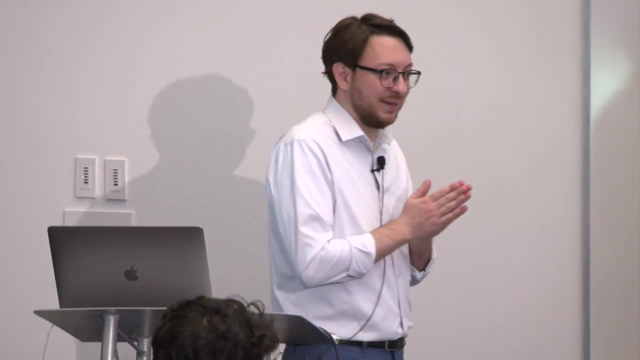 maybe things might get better if you have a mapping with lighters and so on. Yeah, So it depends on the sets of sensor. Humans probably are not the best at doing SLAM. if that can answer, I have a question. Yeah. 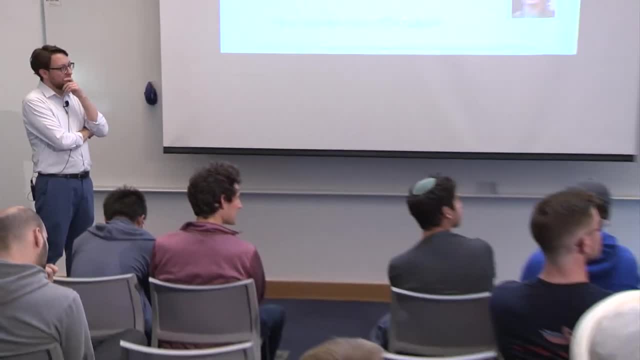 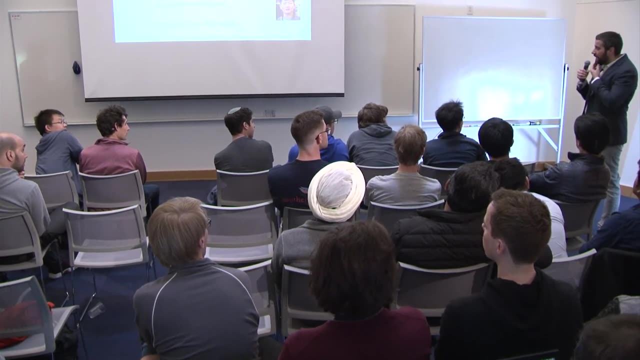 Yeah, Maybe also a general question. So you've talked about perception because you work on perception, But I think I might not be the only one in the room wondering, like, what can we steal from you, right? So there are many other problems that many of us 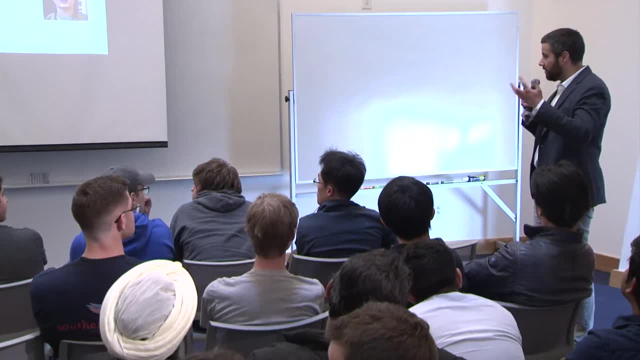 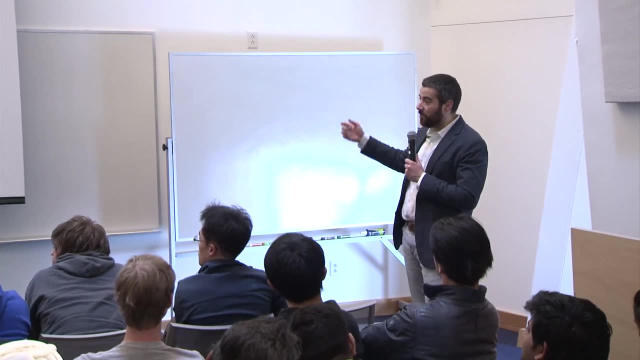 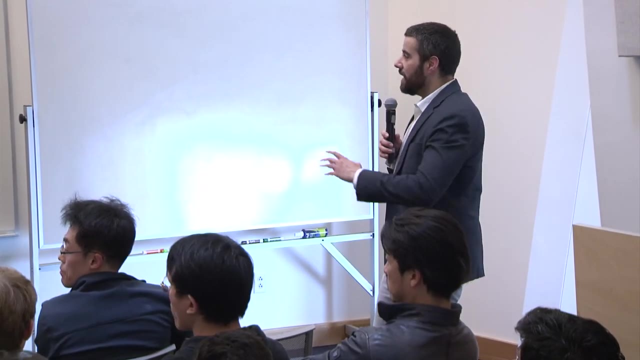 work that there's also hybridness associated with just- I don't know- planning control problems, where that might not have to do with correspondence problems or outliers, but also other types of discrete changes in behavior. So why is this a perception talk and not just general optimization? 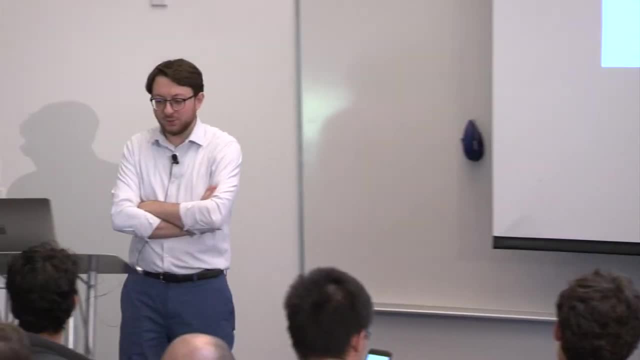 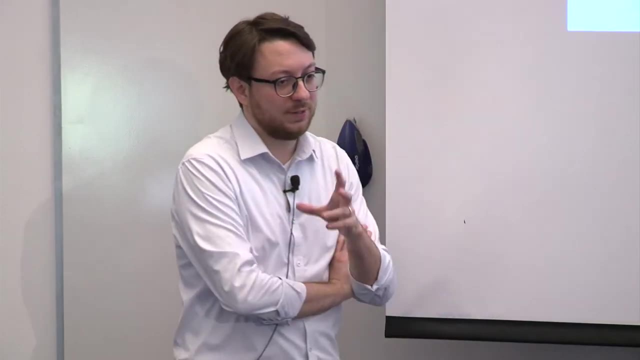 True, I think that if you have a problem, like even in planning, which you're playing in particular with rotations and you're playing with binary variables, probably you can still apply this convex relaxation. Here there is something a little bit important about again. 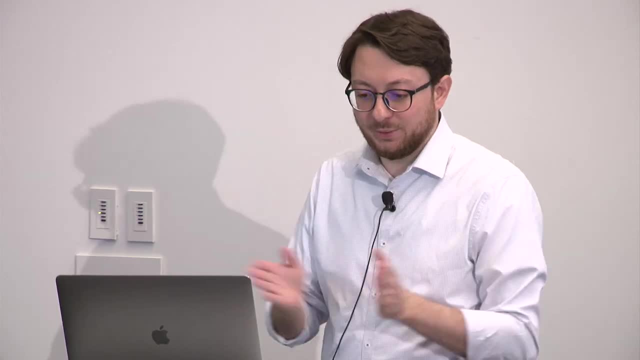 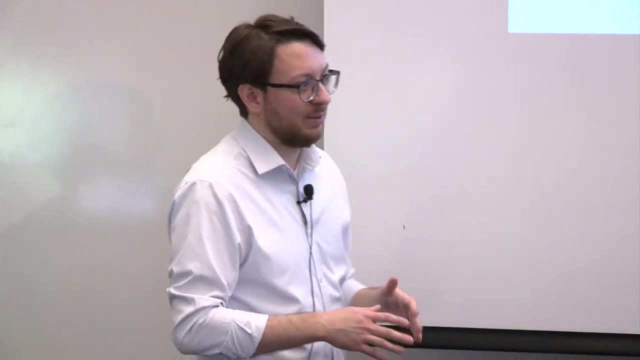 both the binary variables and the rotation being something that you can express as quadratic constraints, And this typically results in good relaxation. Yeah, And you can do the same with the other simulations. If you see the same structure in a planning problem, probably you can do the same. 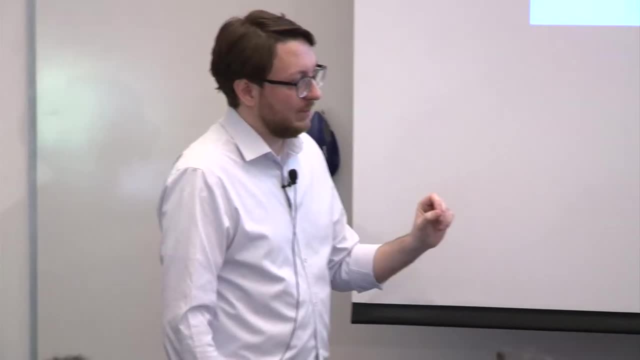 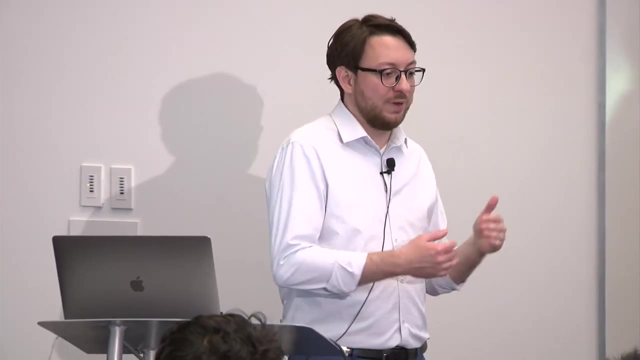 Everything ends up being. you also need to be a little bit clever about the problem formulation, in the sense that this truncated, least square formulation that I have ends up producing, after you do a lot of manipulations, end up producing quadratic cost function in the QCQP case. 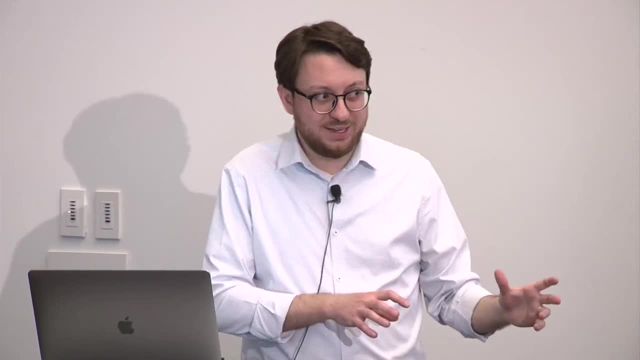 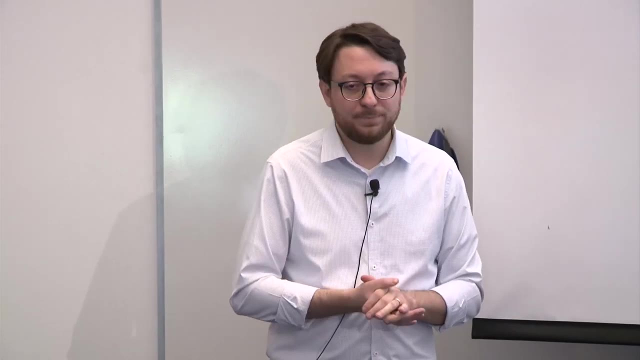 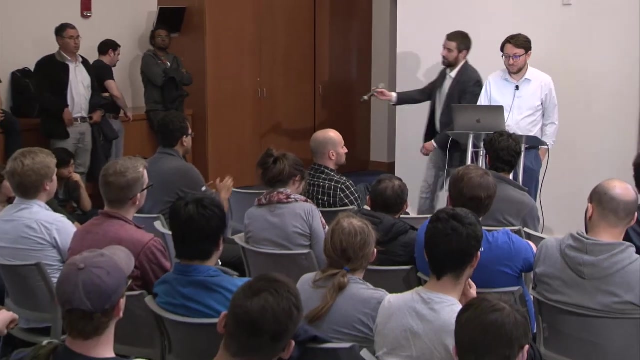 So you need to find that kind of formulation for which the cost is ugly but it's not too ugly, to reformulate it as something like a QCQP, for example, which you guys do in planning as well. So, if I get it correctly, all of this is like an offline slam. 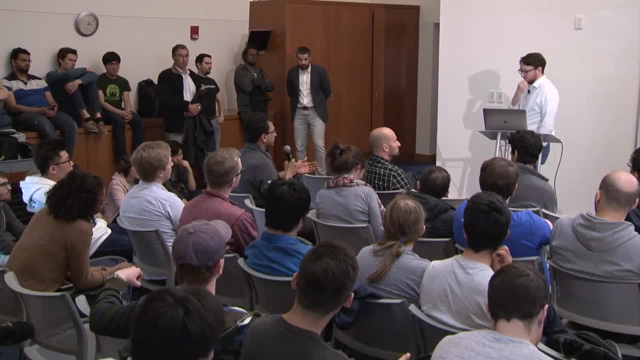 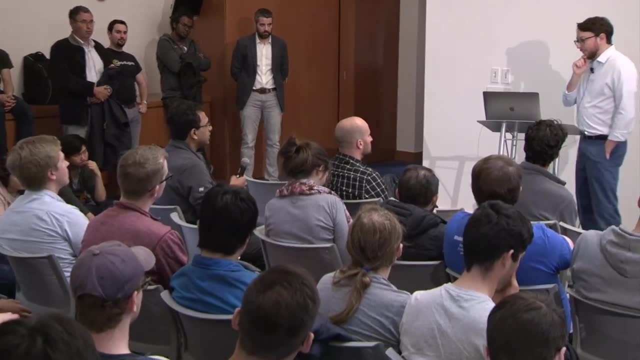 How hard is it to extend these ideas? When I get a new sample, I decide maybe I can reject some of my past samples, or maybe reject the current sample. The way I see this is: it's true that right now it's batch. 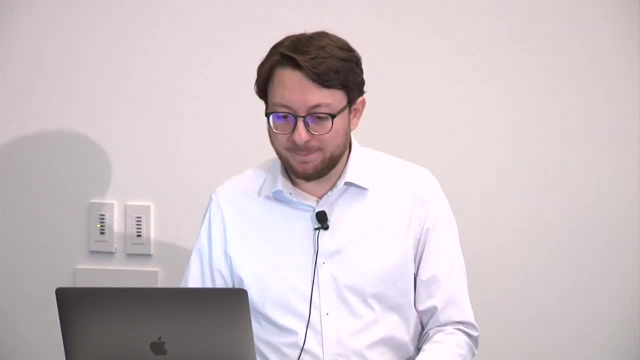 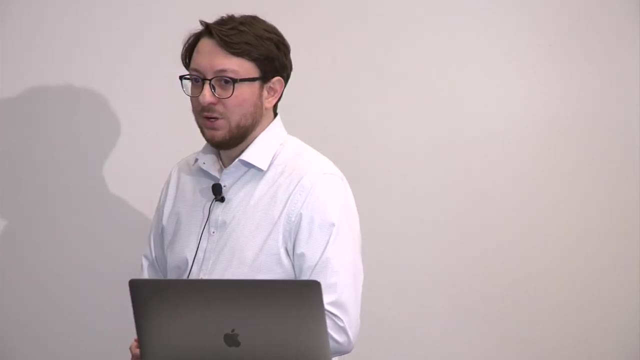 You have all the measurements and you do it. The way I see it is that So you can use it in a recovery stage, like if you detect some problem in your slam, you call these and you solve the problem that you have. Or it would be interesting just designing. 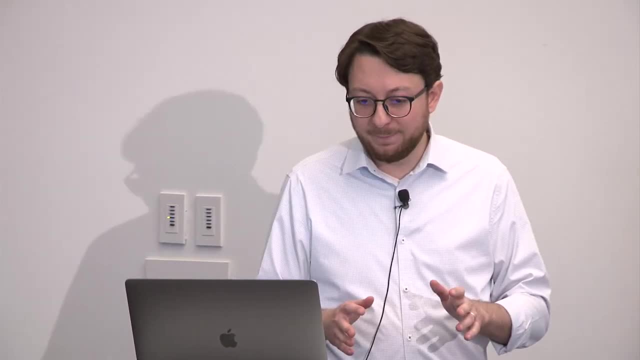 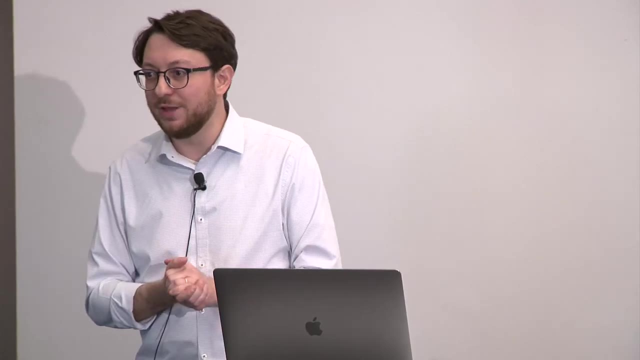 an incremental version of these. For example, you can do some gradient descent technique that as soon as you get more measurements, we'll try to improve the cost function and so on. It's definitely a good avenue for research, But right now, the way we're thinking about it, 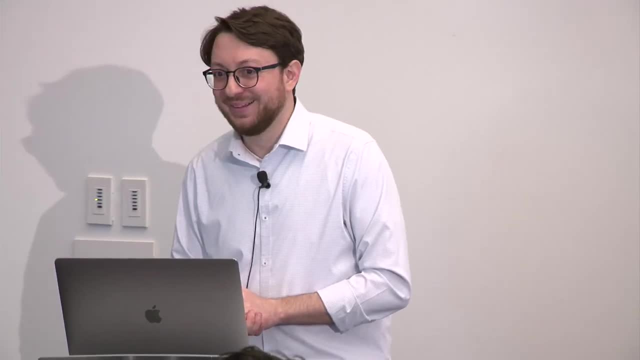 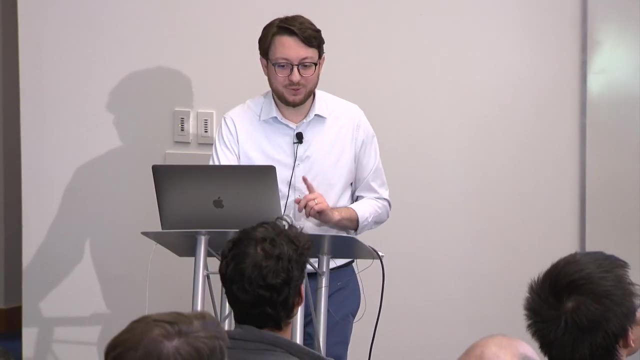 is batch optimization is already difficult enough. So, guys, before taking further, there's another question. I want to show you, really, one thing about the multi-robot keys, And it's a minor thing, but I believe if you guys are not convinced about this being something, 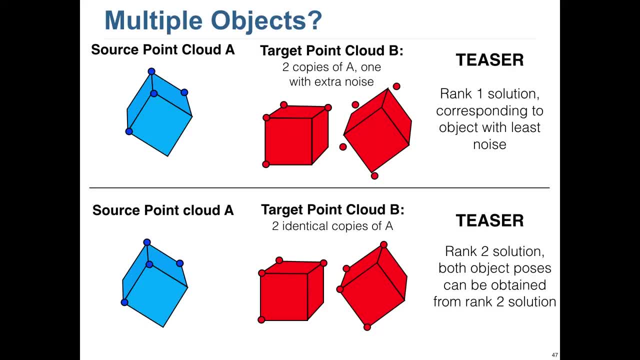 interesting or surprising. I'll show you what happens here in the case in which you have two point clouds: one point, cloud A, which I'm showing here, and a point cloud B that, in this case, contains two copies of the object in A. 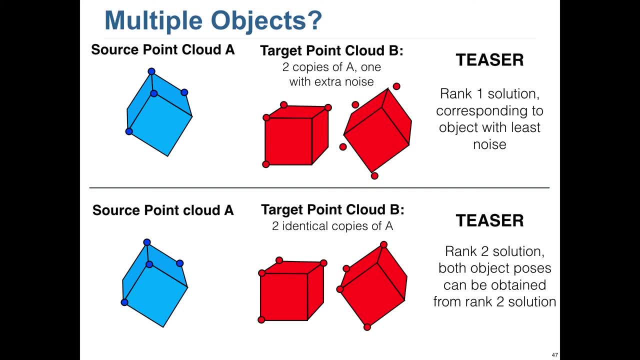 But one of the two copies is a little bit noisier, a little bit more noise. So in this case, the convex relaxation that we propose is still giving a rank one solution. So, no problem, It's able to solve the problem. 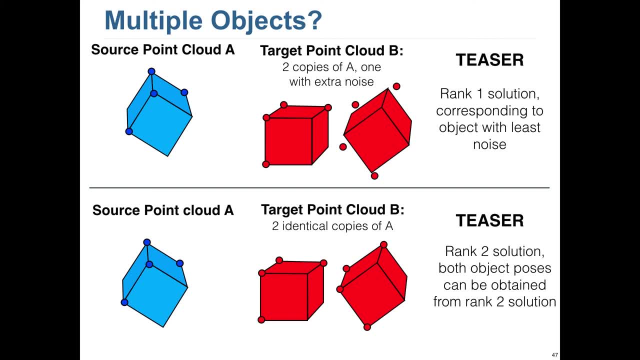 And it's returning the version with less noise because that fits better the data. The thing that is surprising is that a few days ago is that if you said you have the keys in which the second point, cloud contains two identical copies of the object A, what happens is that teaser, which.